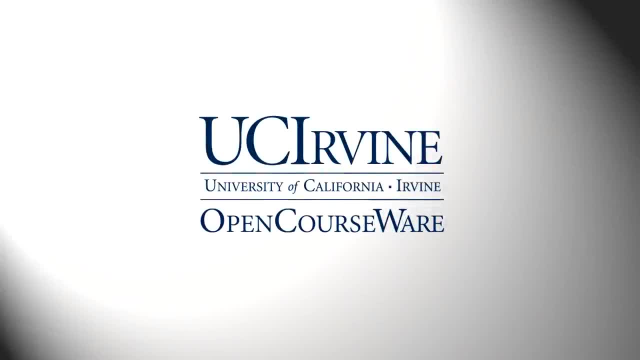 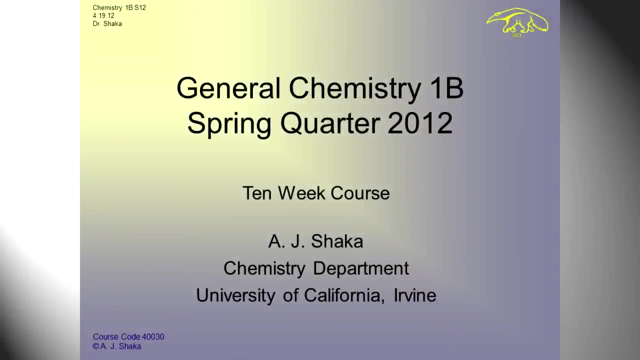 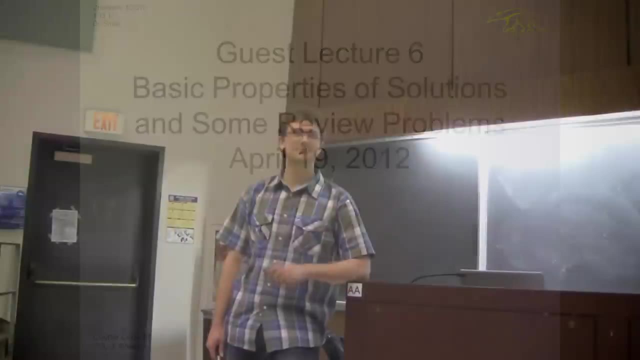 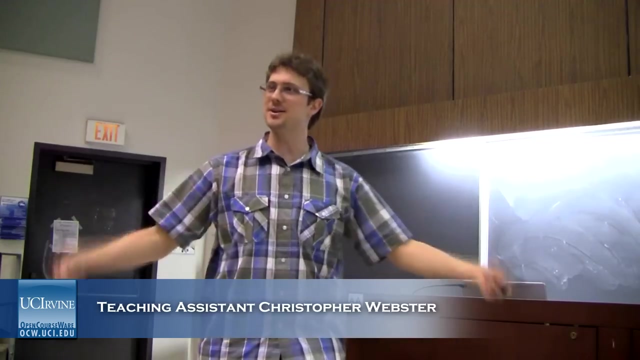 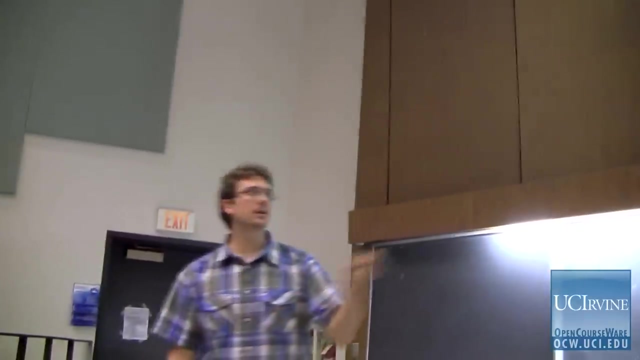 Will I get a round of applause at the end too? Now, Just based on this, That's awesome. Okay, so seven today. I don't know if we'll get through the whole day because apparently my other TA, Mohammed, went through a lot of slides, but we'll get through as much as we can. 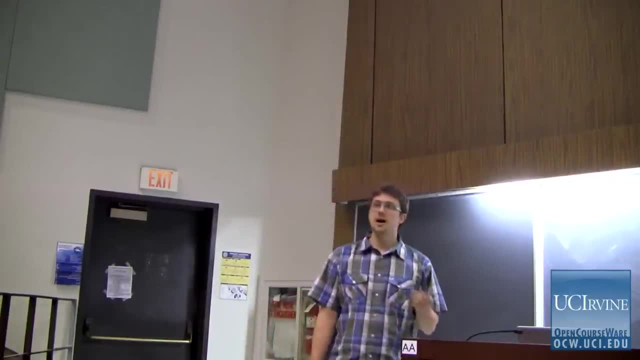 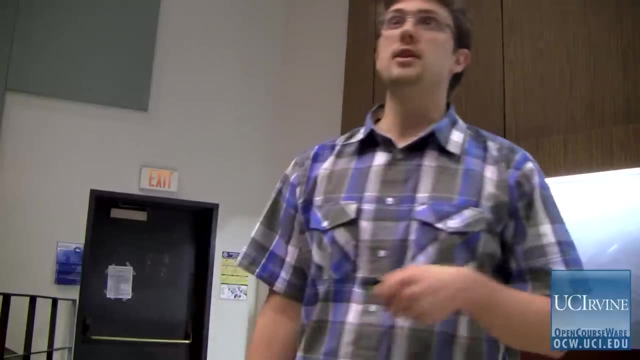 The test is next Tuesday and it covers chapters five and eleven, as well as any review chapters like one through three. Take a look at the syllabus if you're not sure. I would highly suggest to everyone that you read the textbook. The textbook has a whole lot of good information. obviously, That's why we buy it. 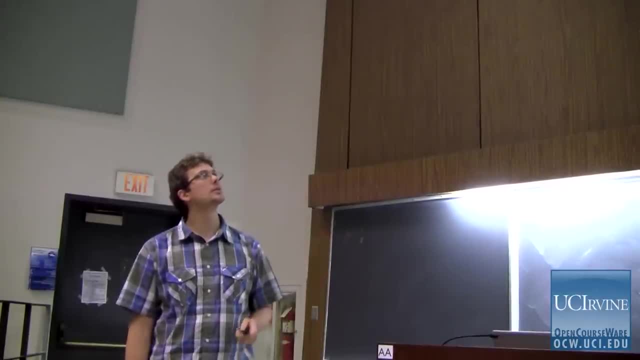 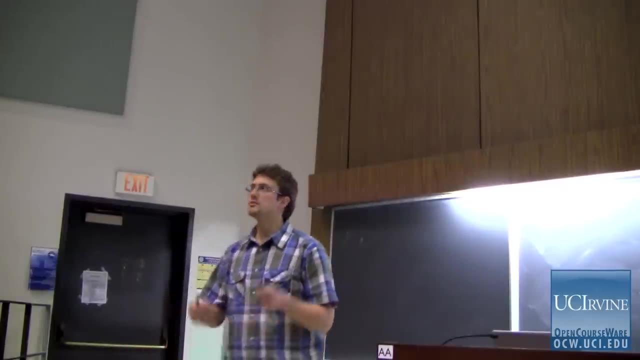 But today we're going to be covering a little bit further ahead in the course. So guest lecture six- I'm that guest Hello- Basic properties of solutions. So when we think of chemistry- like you just picture what happens when we perform chemistry- you usually think of someone. 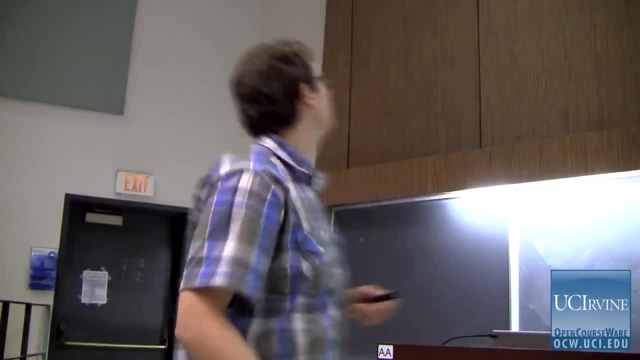 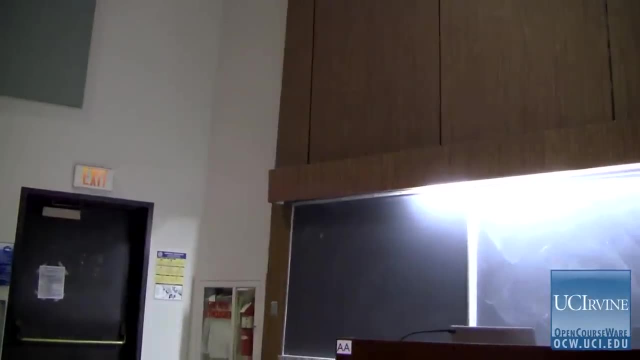 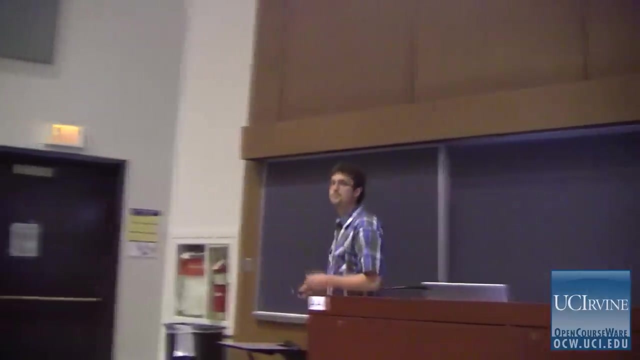 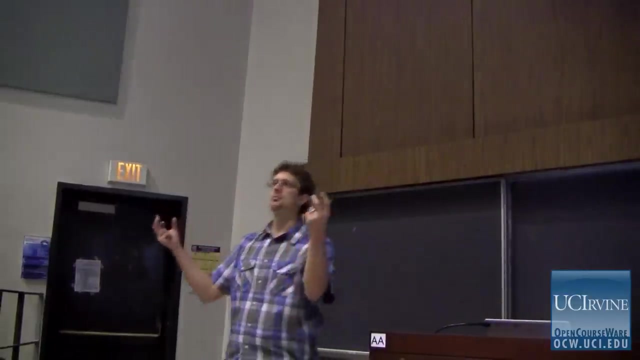 Are you raising your hand there? Yes, Is it possible to turn those off? Oh, yeah, sure Is that better? Okay, So typically, if I picture someone trying to perform some chemistry, I don't usually picture them taking two solid blocks and rubbing them together. 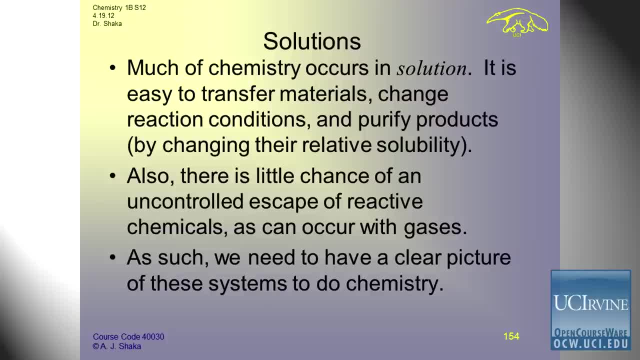 I picture them mixing some solutions. Solutions are very convenient and much of chemistry occurs in a solution, So when we want a reaction to happen, we get. in general, we need two things to collide together. Yes, this isn't always the case, but we need two things to hit. 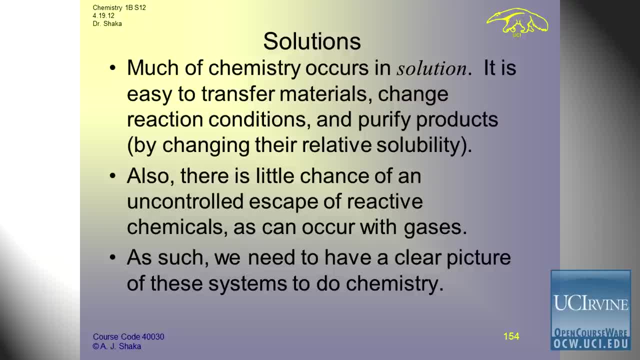 And for that to happen it's a lot easier. in a solution where, Okay, everything's rolling on top of each other, Yes, in a solid state, they're fixed in a fixed spot. It's a lot harder to get them together to react. 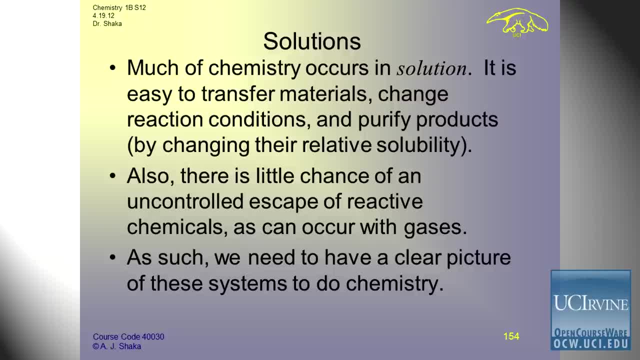 And in the gas phase, yes, you have lots of collisions, but gases can be dangerous. in general We do lots of chemistry with gas phases. I'm just saying it's a lot easier to do it in a solution, And so understanding the characteristics of solutions is very important. 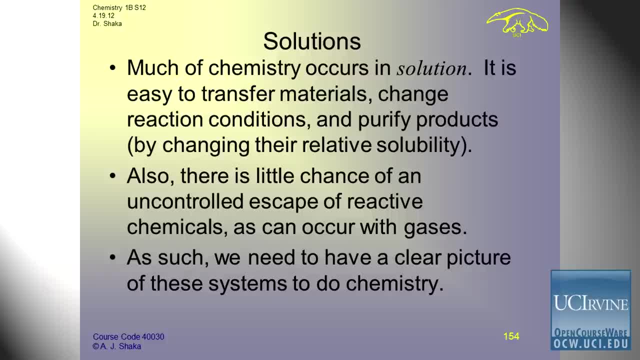 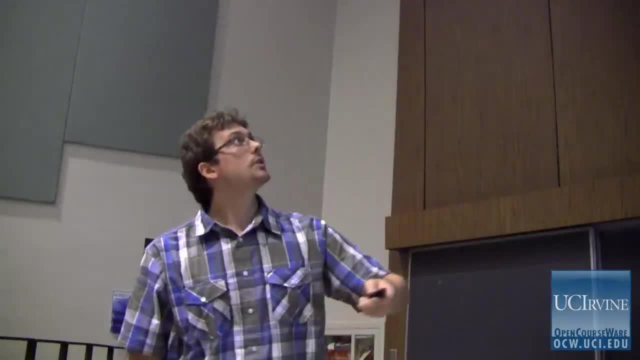 So, for instance, it says here that there's little chance of an uncontrolled escape of reactive chemicals. It's very true. In the gas phase, however, we can sometimes have some accidents. So, for instance- and I don't know if you guys saw this in the news recently- 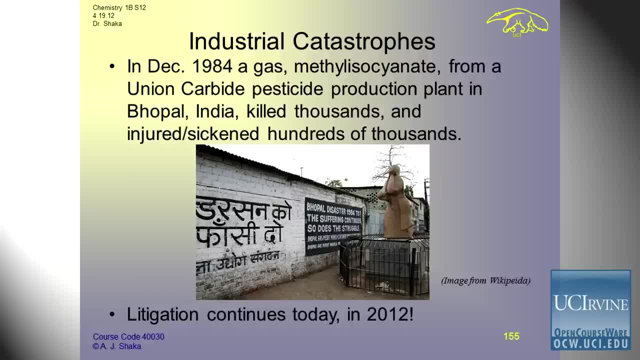 You don't have to look in the science magazines to hear about this. This was a giant accident back in 1984, where methoxycyanate was spilled as gas down. in where was it? Bhopal, India. Thousands and thousands of people were dead. 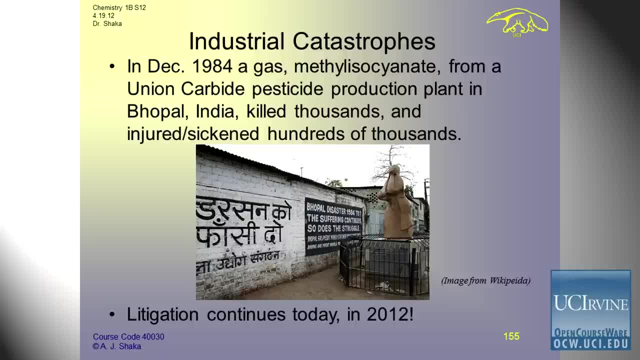 It's because of things like this that we're always questioning: how can I do this chemistry in a safer way? And oftentimes we want to do it in a liquid form. So, for instance, we know that North America has a lot of natural gas. 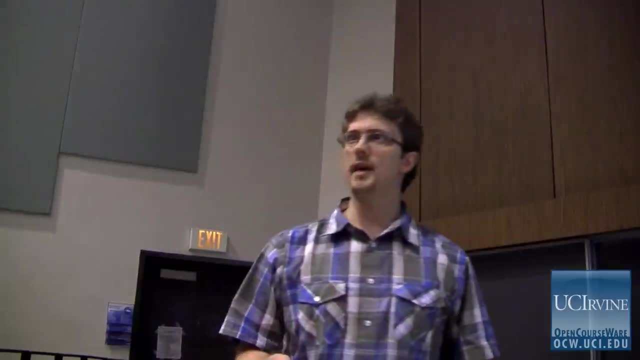 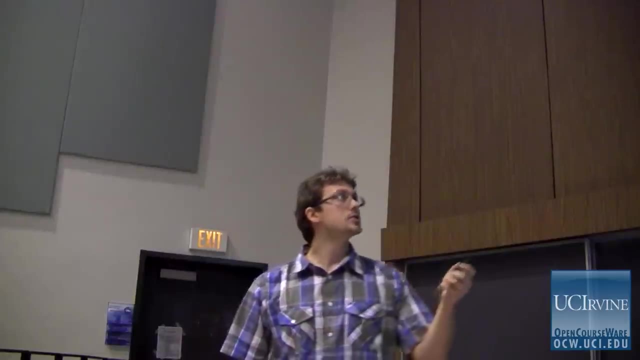 Yes, we could use it for fuel, but it's very dangerous to transport natural gas, And so we always look for ways on how to convert that to a liquid fuel like methanol. Convert methane to methanol so we can avoid accidents. 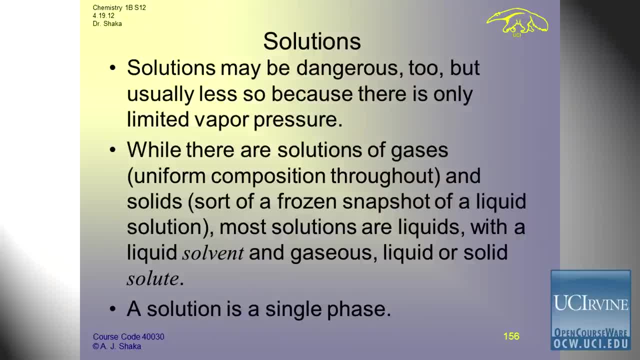 Okay, So solutions can of course, be dangerous too. I know I've spilled things on myself before, But while there are solutions of gases, uniform composition throughout- and solids- sort of a frozen snapshot of a liquid solution- most solutions are liquids with a liquid solvent and gaseous liquid or solid solute. 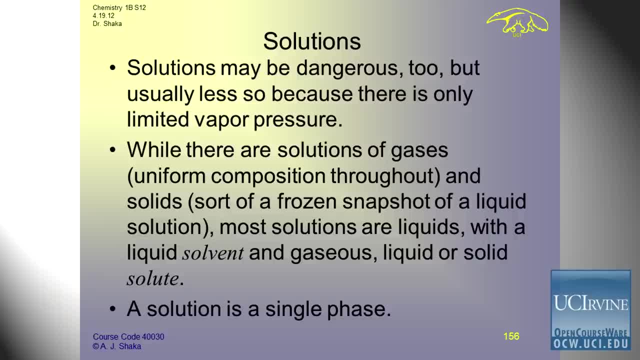 So if you think about that for a second, that last line, liquid solvent and gaseous liquid or solid solute Hydrochloric acid, you guys usually use it as a liquid, right? HCl is actually a gas at room temperature and we dissolve it into a liquid, usually water. 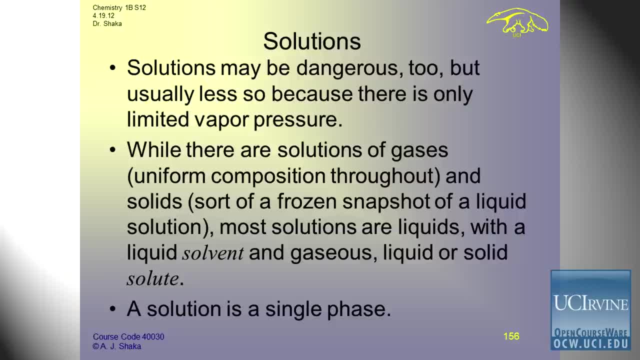 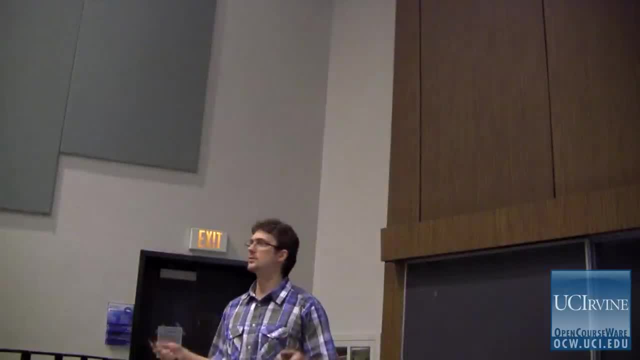 and that gives us the HClS that we work with in the lab. So that's actually a solution. right, It's a gas mixed in Same with a liquid-liquid solution. I could take something, any liquid windex and mix it with more water. 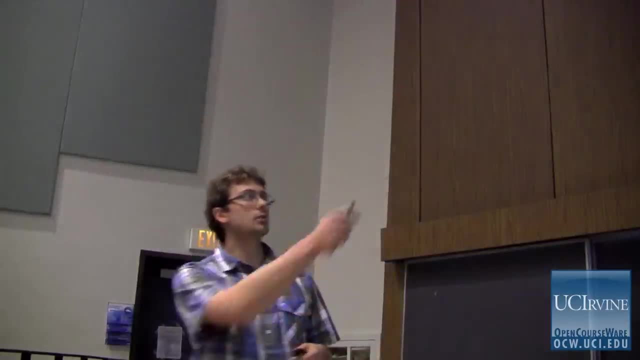 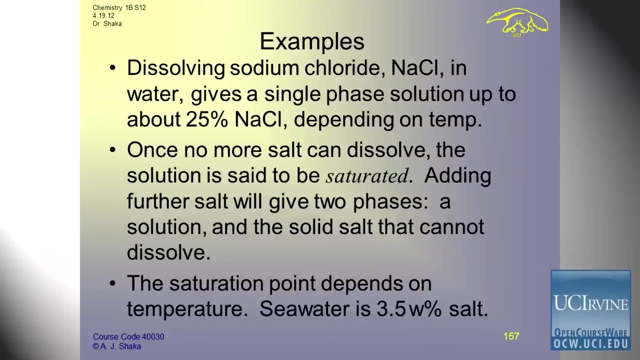 That's a liquid-liquid solution And a solid with liquid. that would be something like sodium chloride, which is a solid at room temperature in a liquid. So, but a solution is a single phase. If I take sodium chloride and mix it in with some water. 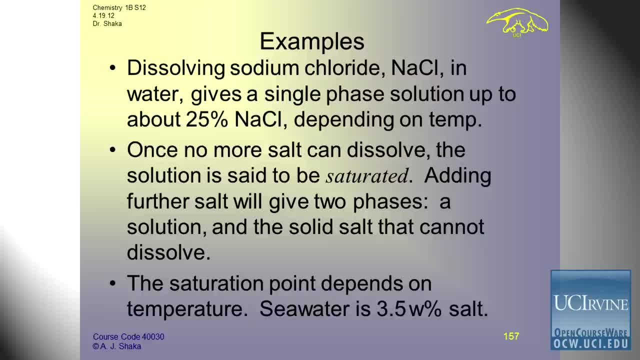 I don't see two different phases present. That's because the sodium chloride is fully dissolved, So I have one phase, just the solution. So dissolving sodium chloride in water, it gives us a single phase, like I was saying. 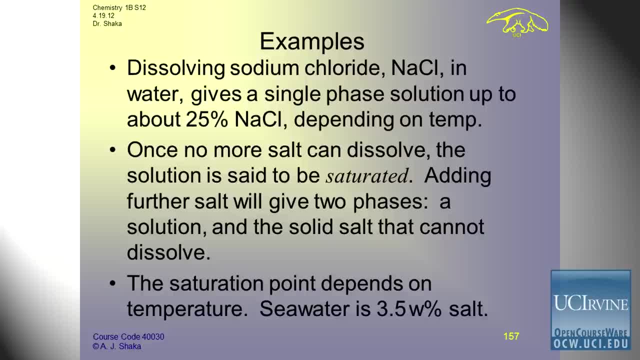 up to about 25% sodium chloride, and that's by weight. So in your first chemistry class you may remember- and I'm not sure if they do it here at UCI, but they may do- a solubility test where you take some water. 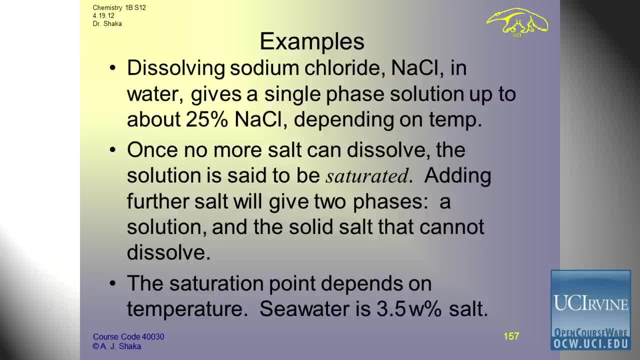 and you put in sodium chloride, And so all of a sudden it will no longer dissolve the sodium chloride and then it starts piling on the bottom. That's when it's reached its saturation point, And for water at room temperature that's around 25%, 25%. 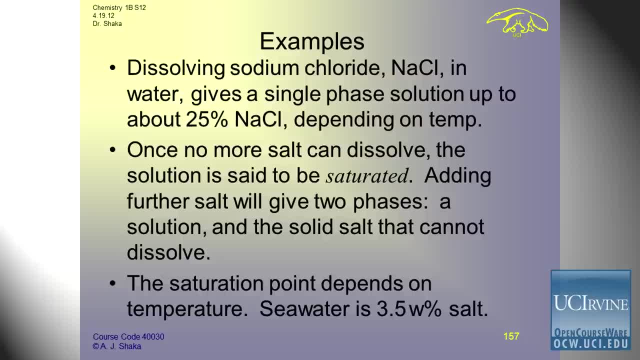 Once no more salt can dissolve, the solution is saturated. Adding further salt will give two phases: The solution which is full of sodium chloride and the solid sodium chloride on the bottom. The saturation point depends on temperature, If we think about that. 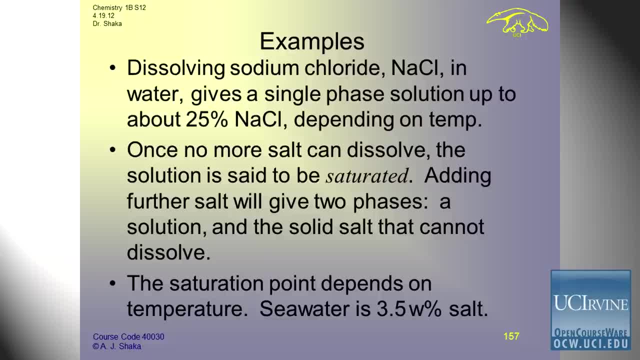 just in general. we know that hot solvents tend to dissolve things faster and easier. They can dissolve more material. This makes sense to us. A surprising note here Before this lecture. I thought sea water was a higher weight percent And just an interesting bit. you know that if you drink sea water normally, 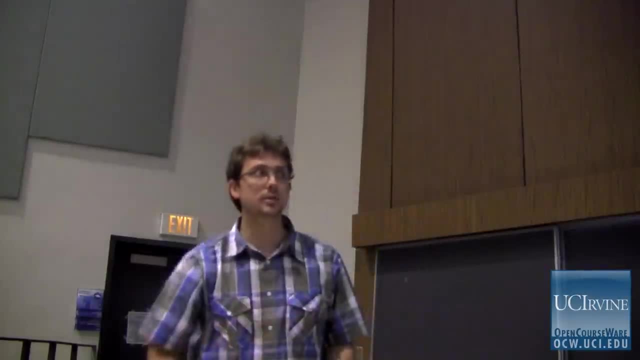 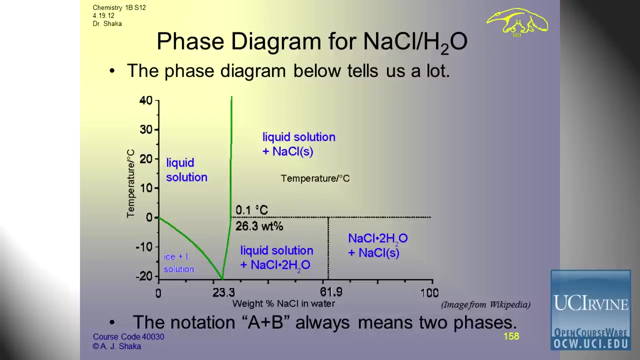 you will die of dehydration And all you have is just that little bit of 3.5 weight percent salt. I thought that was interesting. So a phase diagram. If a phase diagram is not familiar to you, then you should be reading the textbook more. 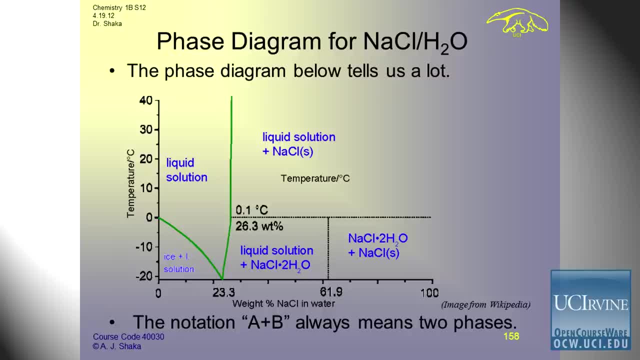 This is a basic phase diagram, But instead of pressure versus temperature, like you may have seen, we have temperature versus the weight, percent sodium chloride in water. I'm going to go through this slowly. So what we're taking is water at 0% here, no sodium chloride. 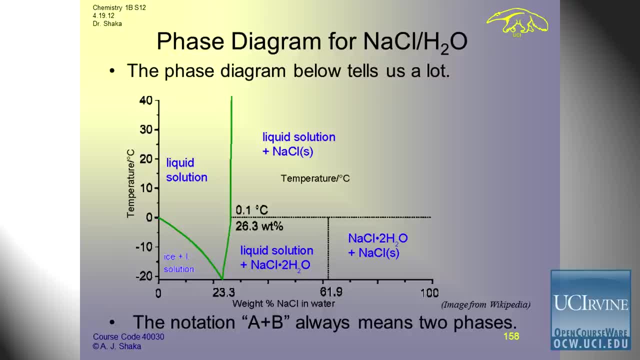 And then we slowly change to 100%. So let's start over here on the left, where we have 0% sodium chloride. Now that's just water, right? So at 0 degrees Celsius, just water. well, that's going to be ice. 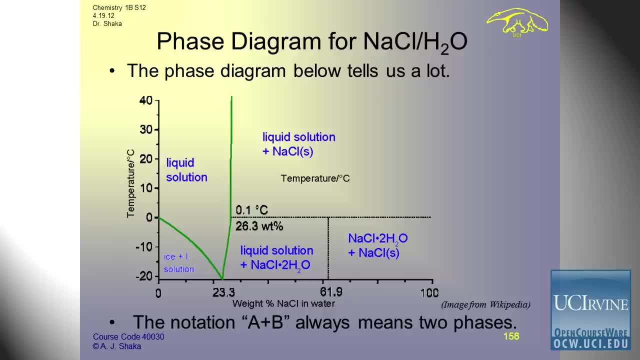 It's going to be frozen And above that it will be just liquid water until you get to 100 degrees Celsius and then it will boil. So you probably have seen or heard about when roads freeze over, like in the mountain passes. it's very dangerous to drive over the ice. 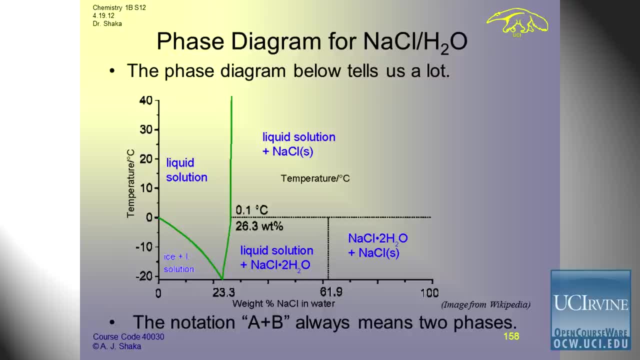 And so what they'll have is they'll come and salt the roads. You may have heard of that before. What they're doing is putting that salt into the water and as a freezing point there's a freezing point of depression. So you can see on this phase diagram. 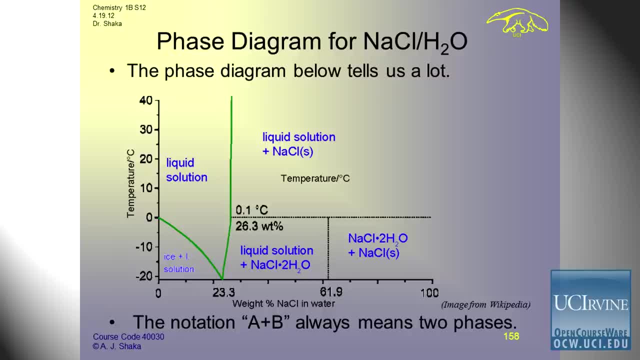 let's start at 0%, and then I put in a little bit of salt. All of a sudden, that freezing point starts to lower and lower and lower down here, And now I see that I can get all the way down to minus 20 degrees Celsius. 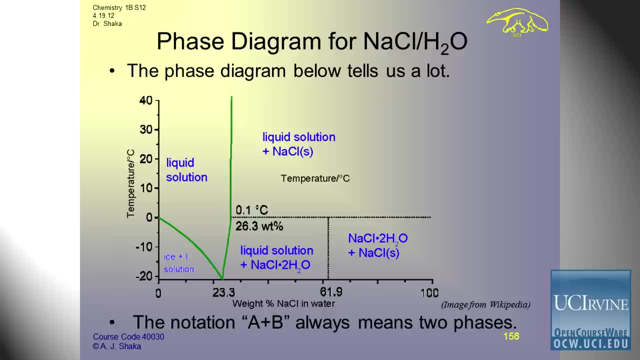 and the solution won't freeze. And this is safe for the roads, because when they put that in there, the ice will melt in general, depending on the temperature, and it's a lot safer to drive on the road. It's a good application. 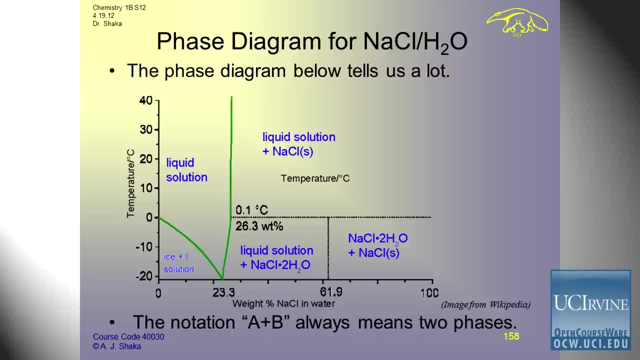 So if we start up in here just as a demonstration, let's say we're at room temperature around between 20 and 25 degrees Celsius. We know that as we add salt then it's going to dissolve. yes, Until we reach this around 25% by weight. 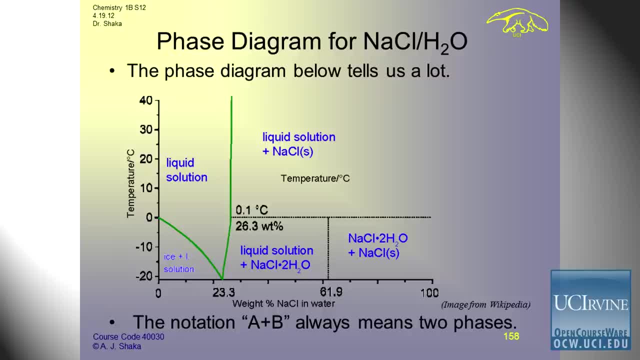 but in chloride. One thing to note here is the bending of this line, So you can see that it's bending slightly to the right. yes, As we increase in temperature, I can see that the weight percent, the total weight percent that I get for liquid solution. 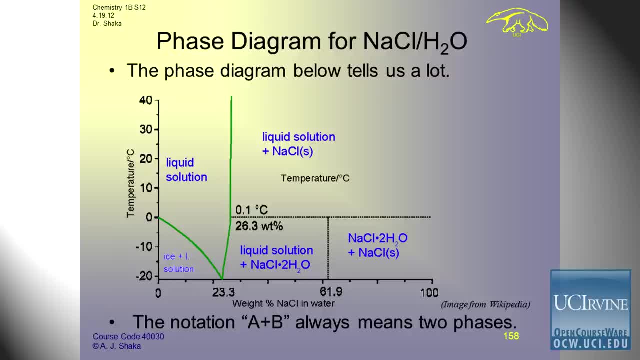 before I start getting liquid solution and sodium chloride, it starts to increase. This is just a visual application to that thought where the hotter we hear, the higher temperature our solvent is at, the more we can solubilize that sodium chloride to get a higher percent. 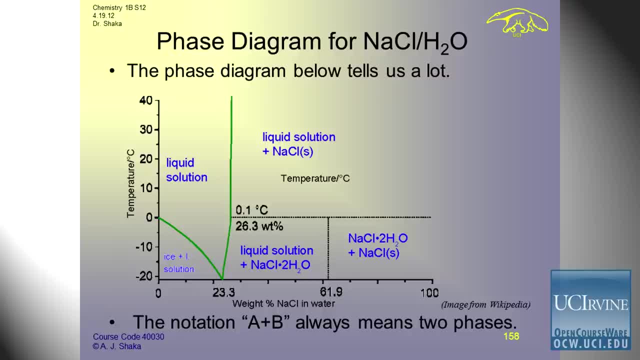 But depending on the temperature we're at, we'll pass into this phase the liquid solution plus sodium chloride. Let me just mix this. So the notation A plus B it's always in these two phases. So in this instance, 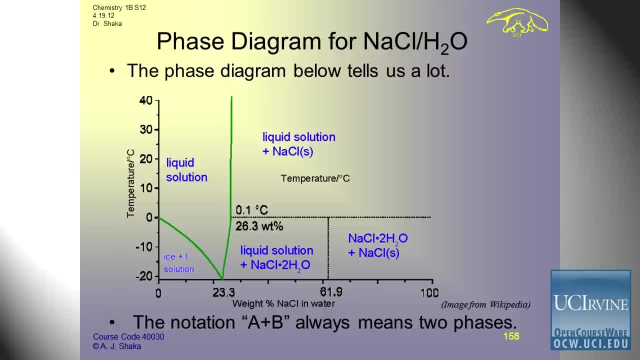 we would have liquid solution as one phase and the solid sodium chloride as another. If we took this liquid solution plus sodium chloride and start to cool it, at one point we're going to get liquid solution plus sodium chloride that's hydrated. It's simple to think. 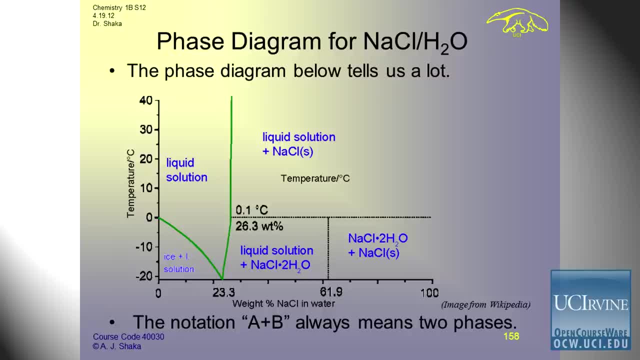 If you're cooling it down, more material is going to crash out. You're solubilizing less, But as you get down to really, really, really cold temperatures, you start putting that water on sodium chloride. So if we think of this in tropics- 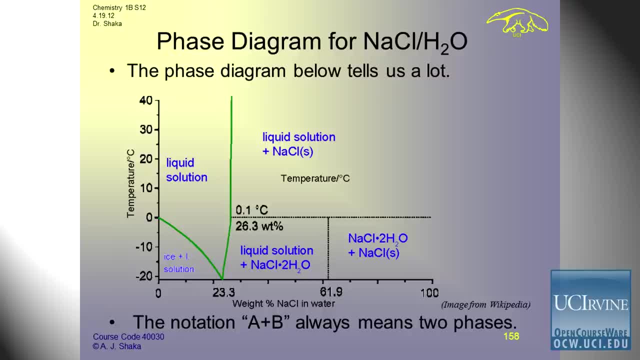 as you cool, as you lower the temperature, it's a lot easier to get things to hit together and stick, So that sodium chloride tends to crash into one of those waters, or rather it's water crashing into sodium chloride and it'll stick. 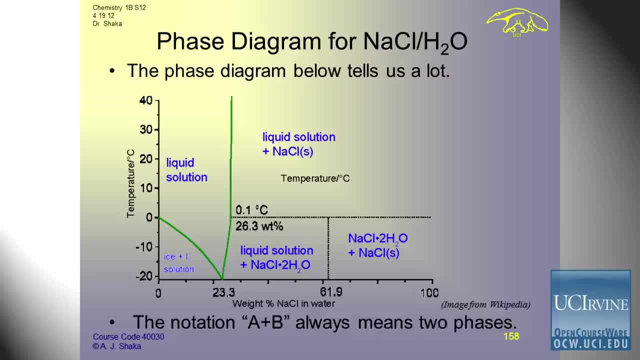 So we get this hydrated form And as we increase the percentage of sodium chloride more and more and more, we see that we get the sodium chloride 2H2O plus just sodium chloride solid. And that's because, if you think of this as a phase diagram, 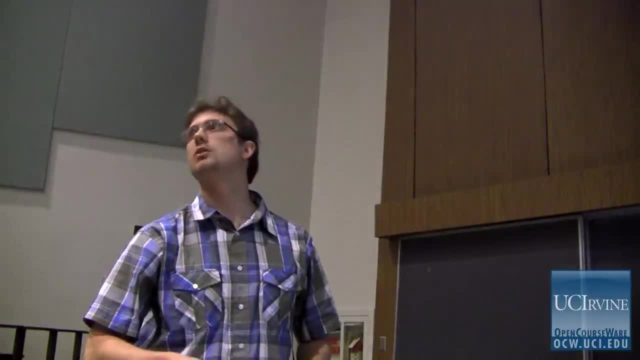 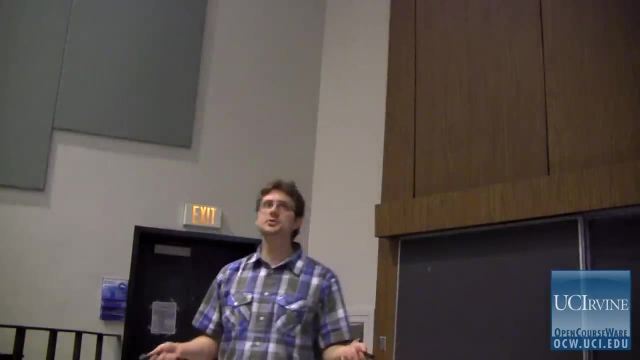 what we're saying is: oh, in this region I have almost no water left and it's almost all sodium chloride. So why do things dissolve? It's the same reason that gas spreads out: It's to fill a container. 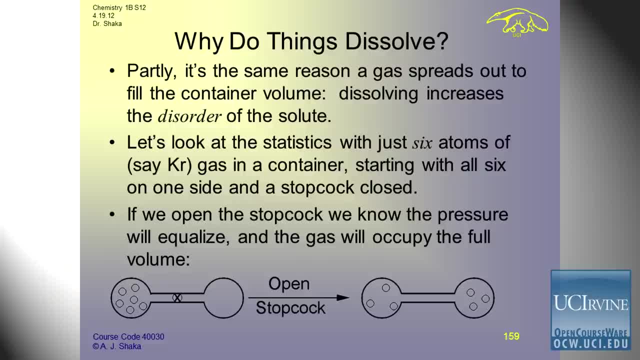 It's statistics. It's hard to keep things in one spot. Things like to spread out. So dissolving increases the disorder of the solute. You can think of it just based on statistics and you don't have to take in a class. 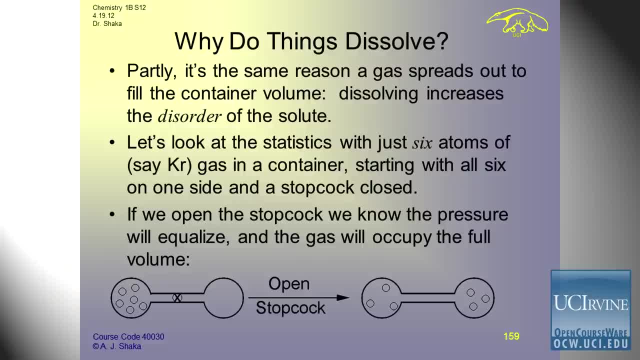 to just think of it with common sense. So let's look at the statistics. with just six atoms, We're just going to say krypton, but it doesn't matter, This is just six particles, It could be anything. So we're taking six atoms of krypton gas in a container. 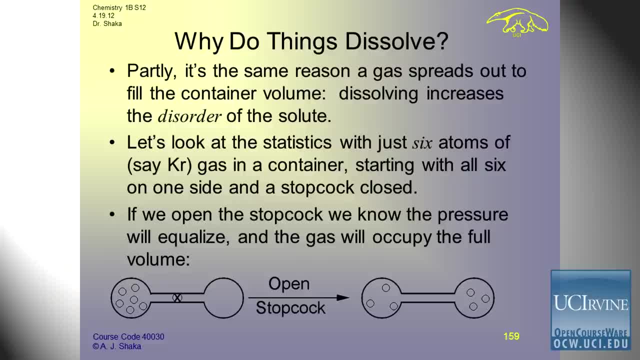 starting with all six on one side and the stopcock closed. There's a picture in just a moment. I believe it's next. Yes, it's next here. So imagine we have this scenario where we have two containers and there's a stopcock here. 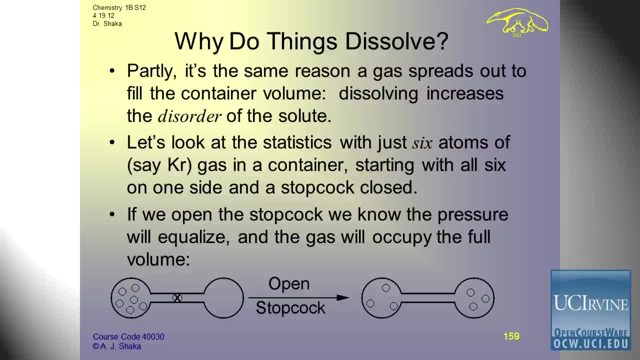 so it can effectively block it off. At one point we put six atoms, which of course just mentally that's an obscurely small amount of atoms. This is just a demonstration: Six atoms of krypton on one side, and then we open the stopcock. 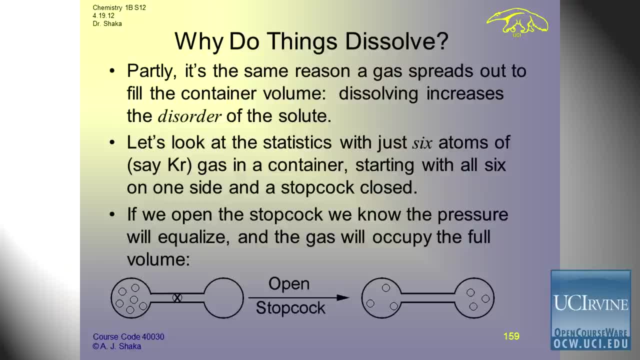 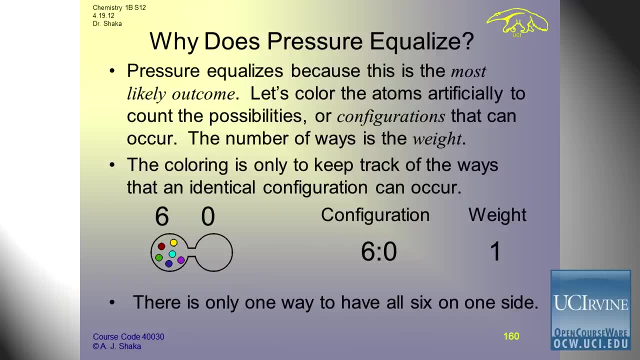 We know just from common sense that that's going to equilibrate until they're on both sides. So why does this happen? Why does the pressure equalize? It equalizes because this is the most likely outcome. If I go back for a moment, 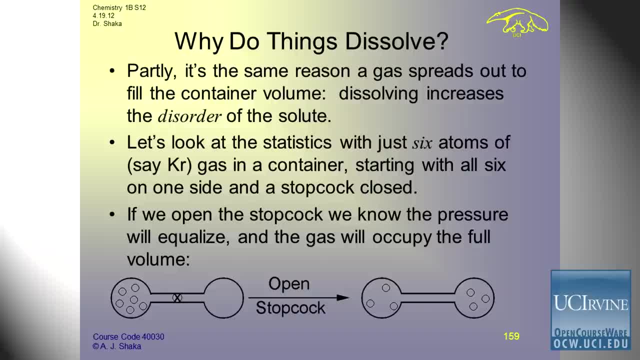 and take the moment when there are six atoms of krypton and then I open the stopcock. what's going to happen? So I've got six atoms that are just crashing around all over the place and I have an opening. Naturally, 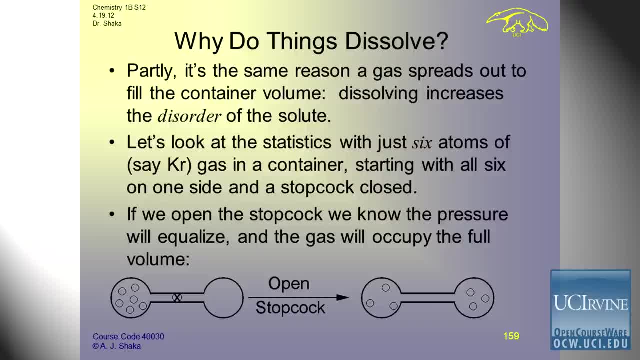 since there's nothing here, it's a vacuum- those are going to statistically start bouncing over onto the other side, And then, once I get onto the other side, they're also going to have a chance of bouncing back, until, of course, 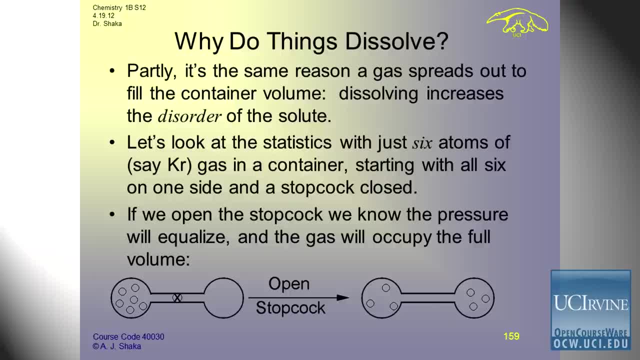 I reach this final state where it's equal on both sides. Now, this is an example with only six, So what I'm going to do is I'm going to start bouncing over onto the other side and then, once I get onto the other side, 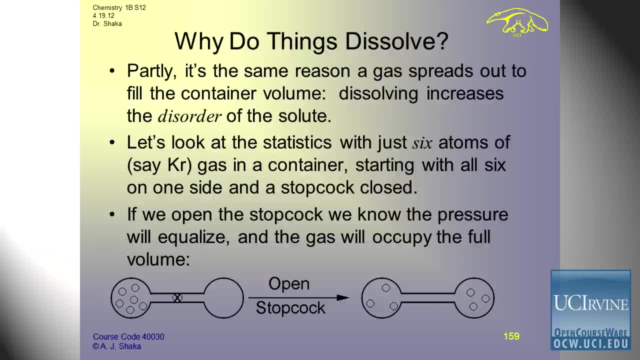 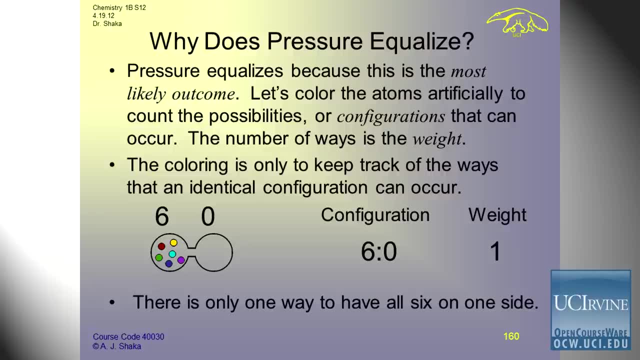 they're also going to have a chance of it not being equal on both sides. So here we've taken these atoms and we've colored them Again. these are just krypton, They're just colors. so you can see a difference in individual atoms. 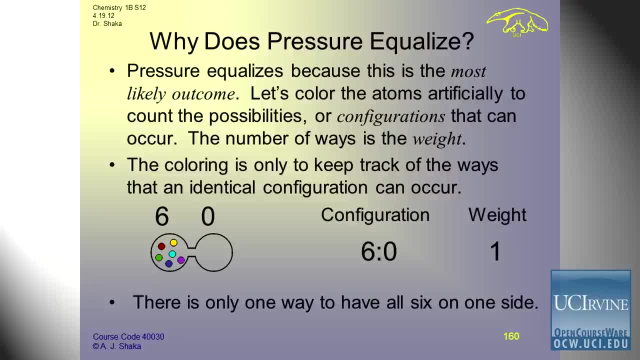 So we take these six different colors of krypton and this is a certain configuration. It's one possibility. And when it talks about the weight, this is a statistical weight, It's not a mass. This is how much does visible energy? 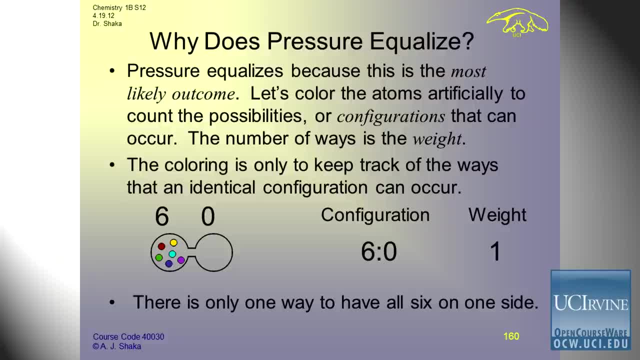 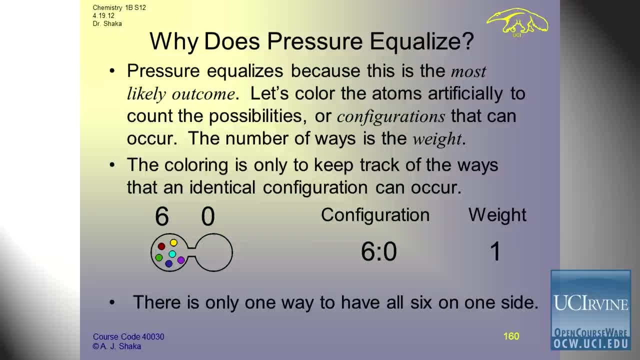 to contribute to the total possible outcomes, and we'll go over to weight in one moment. So we have this scenario where I have six on one side, that's a six to zero. So there is only one way to have all six. 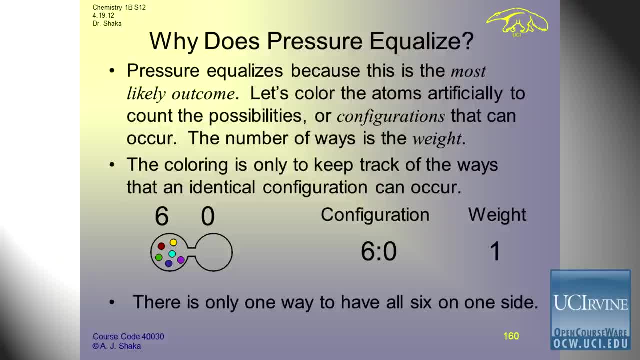 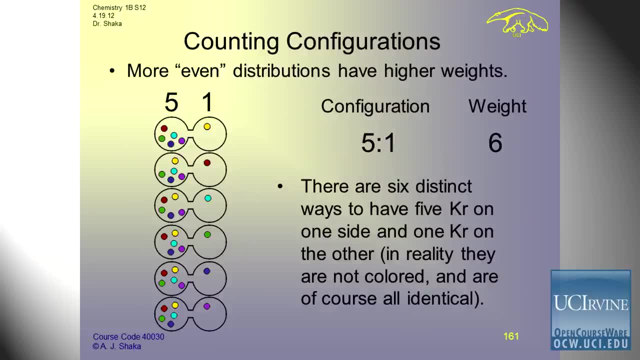 on one side, right That way, right there, all six colors in one hole, nothing anywhere else. So, moving on, if I have, if I change a little bit and bring over one, a more even distribution weight. So before let me demonstrate, we have a weight of one for this. 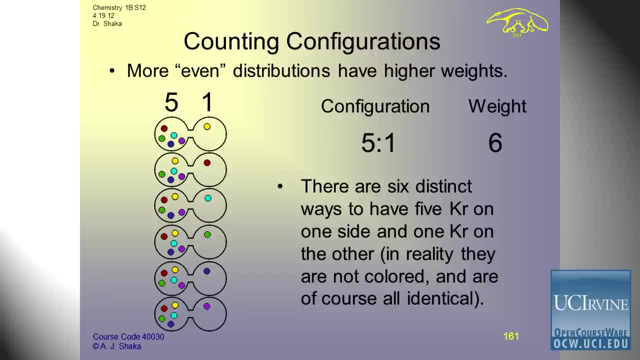 configuration. It has one possible way of happening. When I go to just five and one, I see that I have six possible ways to do this. The configuration of five to one, taking any one of these colors: yellow, red, blue, green, blue, magenta- I don't. 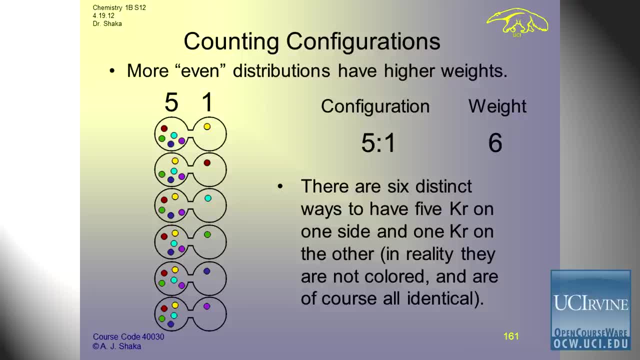 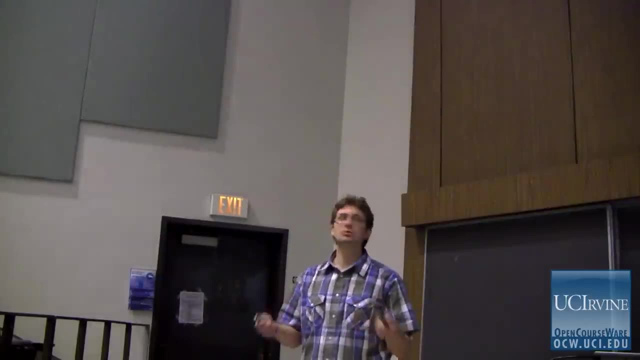 know, taking one out of side. there are six different ways to do this, just statistical randomness. I already said that. So by the time we get to four and two, there are a whole lot more possibilities. We can take them — obviously I'm not to go. 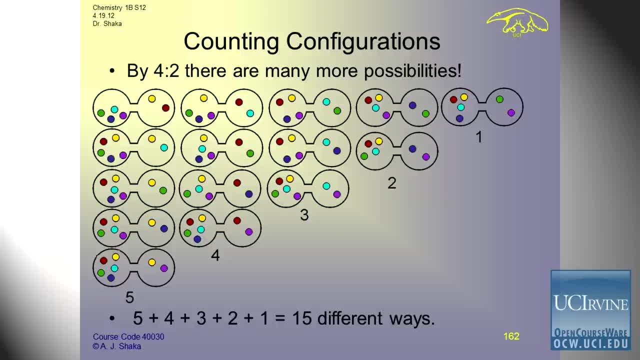 through each one of these — but you can take any combination of these colors, with four on one side and two on the other, and you find that, find that there are 15 different ways. You can see how this grows exponentially And in fact it is exponential. 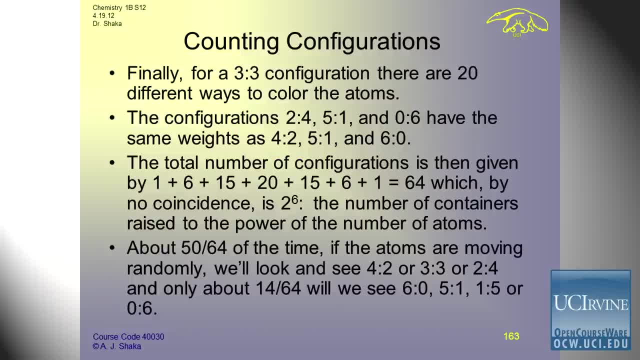 Counting configurations. So, for the 3 to 3 configuration, there are 20 different ways to color the atoms. The configurations 2 to 4,. well, let me go back for just one second. So you can imagine that, with all these possibilities, with 4, 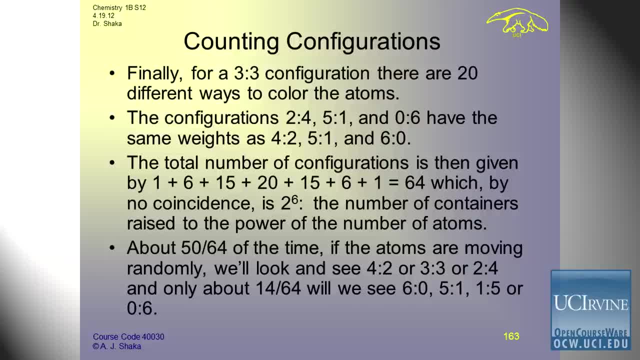 and 2, now we move one more over, And with 3 and 3, there are 20 different ways to color those atoms, 20 different possibilities. And then, remember, we had two containers right, One on the left and one on the right. 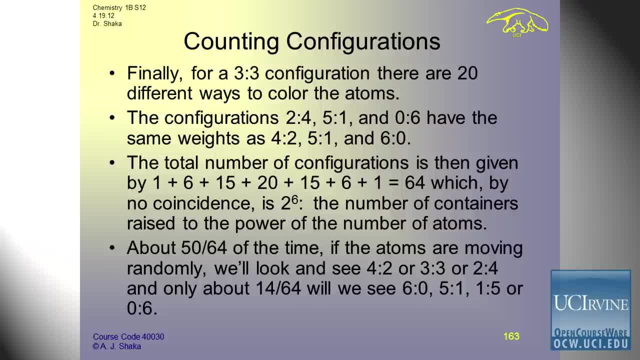 And we were starting with the one on the left being more filled. If you go to the opposite side, the one on the right being more filled, all the statistics are the same. You're just doubling that possibility. So the configurations 2 and 4,, 5 and 1, and 0 and 6. 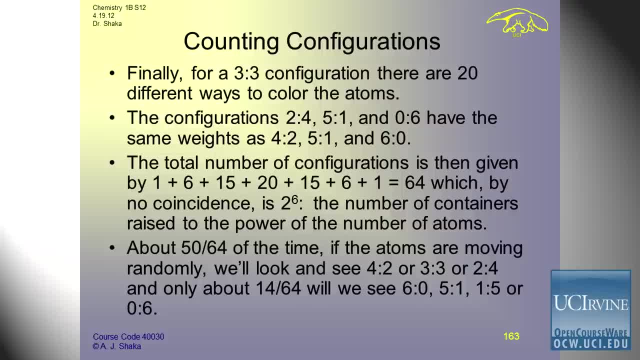 have those same weights as 4 and 2,, 5 and 1, and 6 and 0. They contribute just as much, So the total number of configurations that we have is given by 1 plus 6 plus 15 plus 20 plus 15 plus 6 plus 1. 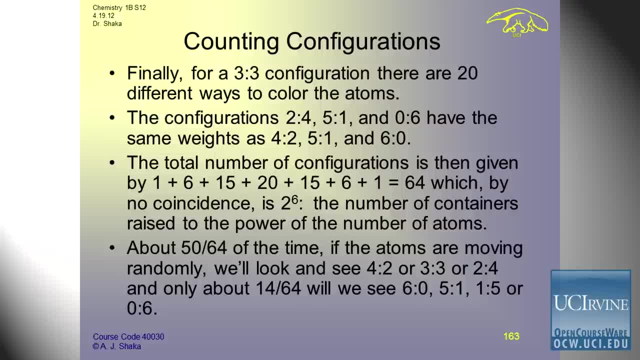 equals 64.. You can see, what we were doing was starting with 6 and 0,, 1,, 5 and 1, and that contributes 5, and so forth until it's even, And then you can go to the other side. 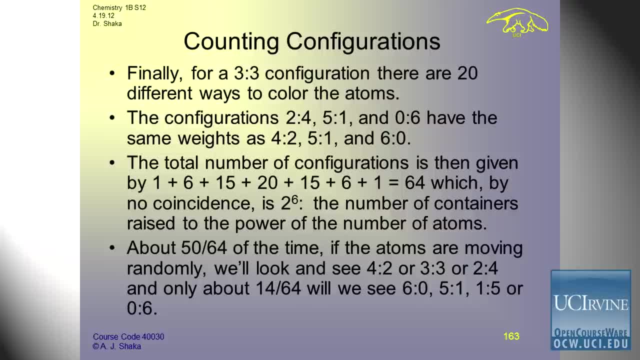 That's how many possible orientations of the system there were And that's 64 total, which, as I mentioned earlier, no coincidence as being exponential. it's an exponential statistical analysis: 2 to the 6.. The number of containers: 2, raised. 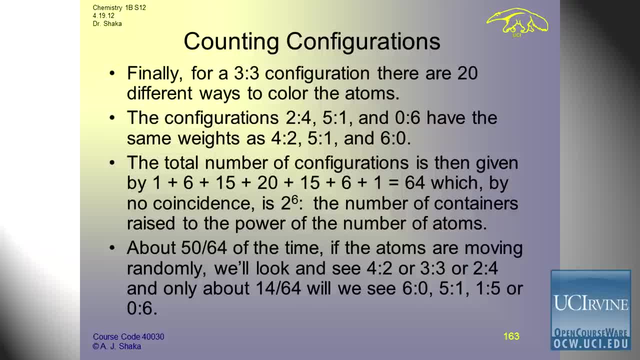 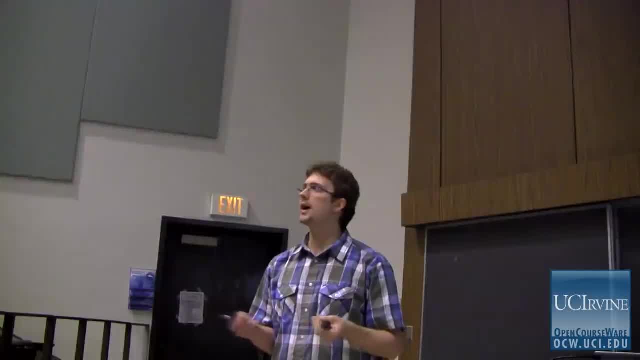 to the power of the number of atoms You'll mention in a moment, and I'll just say it now. you can imagine that with 64 and only 6 atoms, just think of how many atoms are in a balloon. right, If those were, just if those were two metal containers. 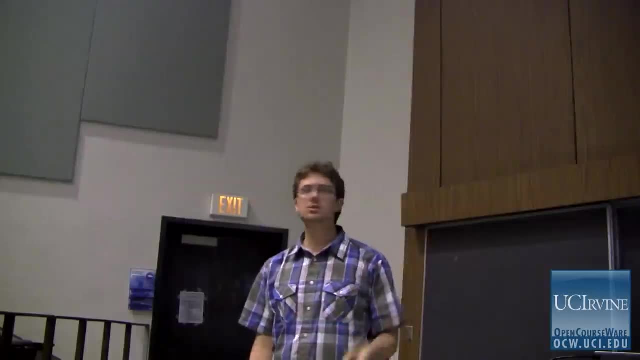 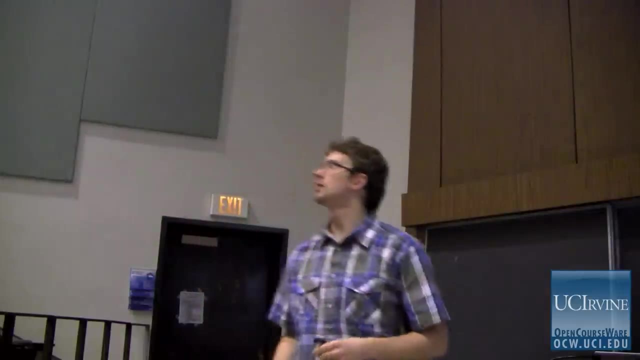 and you had an atmosphere and one and it opened it up. If it's exponential like that, the number of possibilities that include atoms, The number of atoms mostly on one side, they don't contribute anything at all, It's statistically insignificant, it doesn't matter. 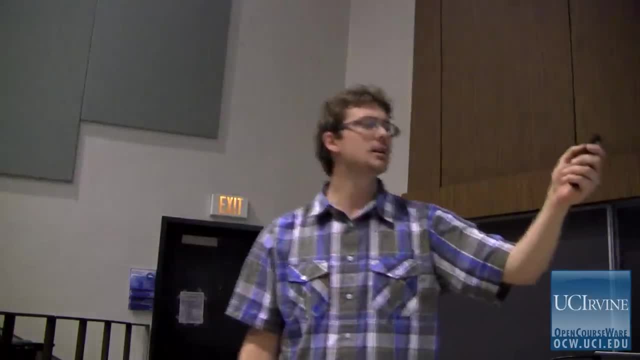 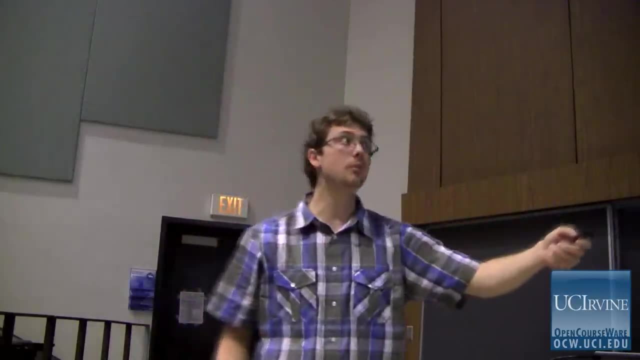 And so by the time you get to any sort of significant amount of atoms, there's no point in even considering a situation where the atoms are mostly on one side. They're equal. They will equilibrate About 50 for 64th of the time if the atoms are moving. 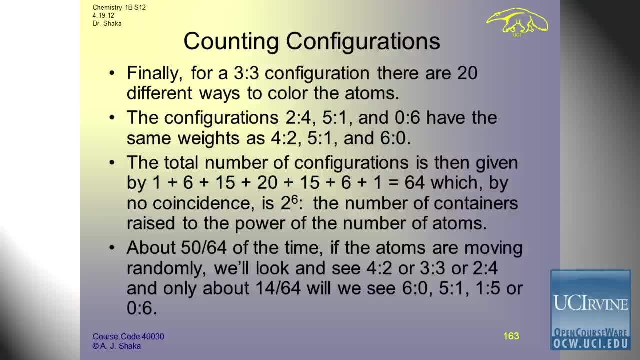 randomly, we'll look and see a 4 to 2, or a 3 to 3, or a 2 to 4. And that's just adding up Those possibilities. okay, equals up to 50 to 64.. 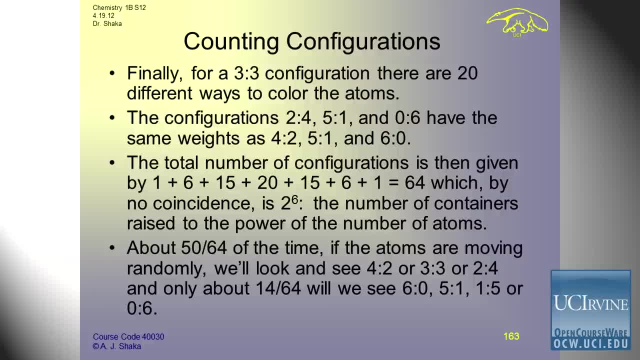 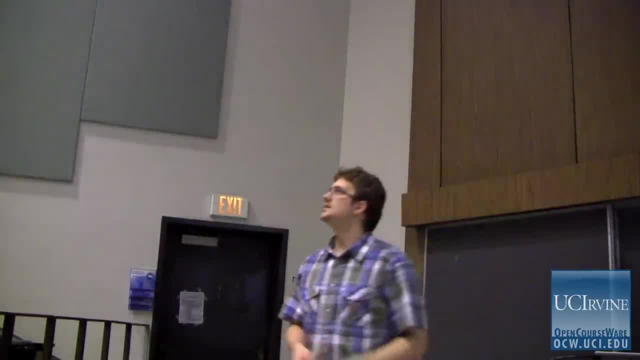 And about 14 of 64 times, we'll see that 6 to 0,, 5 to 1, or 1 to 5, or 0 to 6.. So, like I was saying, if we took that 64 and made it 10 billion, 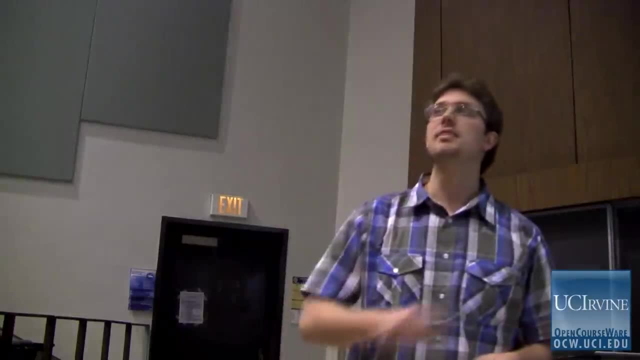 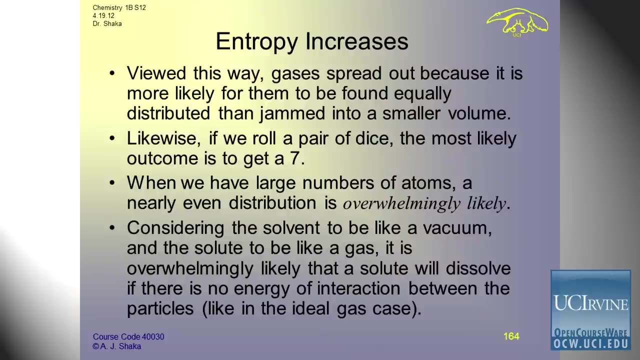 right Avogadro's number, what is it? 10 to the 23, that's way beyond a billion. You're talking about huge, huge numbers now. So when we view it this way, the gas is spread out just because it's more likely. 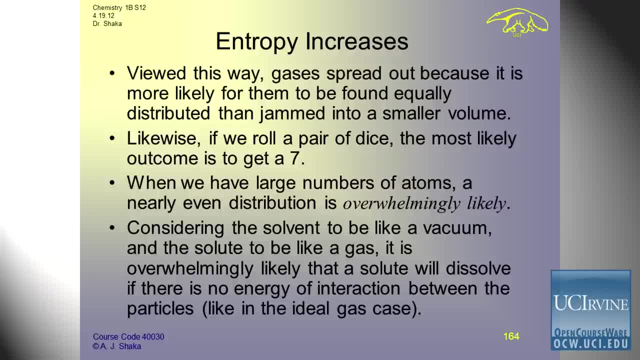 When the first scientists started looking at these systems, they didn't have to have the chemicals. They could just envision what's mathematically correct to first approximations. when you don't consider chemical interactions, Math describes almost everything. It goes into physics. 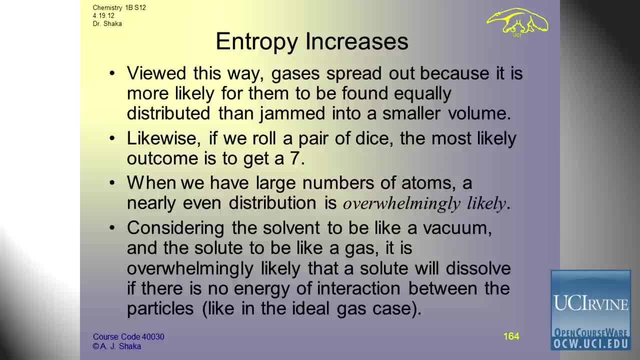 It goes into chemistry, It describes the world. It's only when you start taking exact scenarios where you have to start considering how atoms interact together et cetera. That's fine. So it's more likely for them to be found equally distributed. 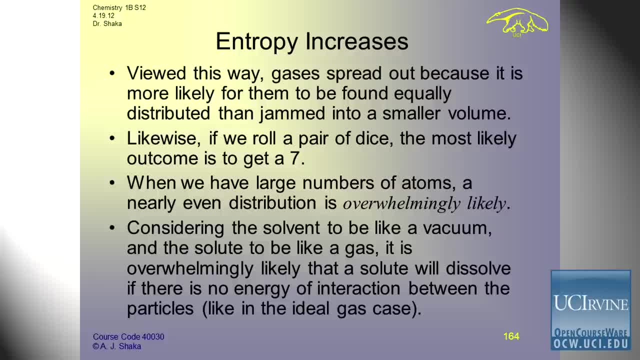 and jammed into a smaller volume. Likewise, and again, it's just going to statistics: if you roll a pair of dice, the most likely outcome is to get a 7. So when we have large numbers of atoms and nearly even distribution, it's overwhelmingly likely. 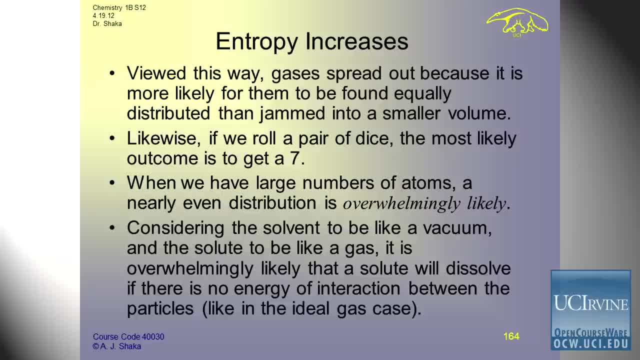 Considering the solvent to be like a vacuum and the solute to be like a gas. so consider for a moment if I had a I don't know, a I don't know- A beaker full of water with solid sodium chloride on the bottom, right before it's dissolved. 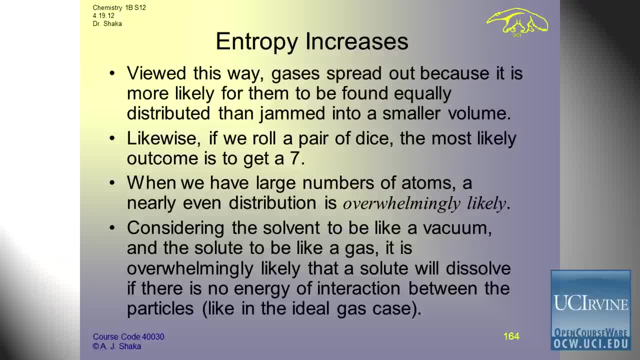 It's just the instant before we stir it and it dissolves. That's like a concentrated one balloon that's concentrated with gas atoms. right, It doesn't like to just sit there when there's room in the solution for the sodium chloride to dissolve. 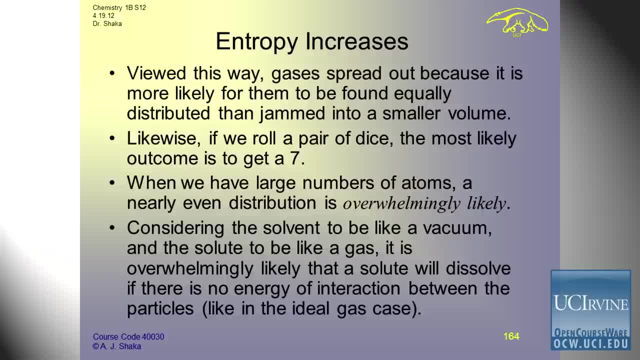 So, considering the solvent to be like a vacuum and the solute to be like a gas, it is overwhelmingly likely that a solute will dissolve if there is no energy of interaction between the particles, like the ideal gas case. So they're saying, in the event, that sodium chloride had no interaction. 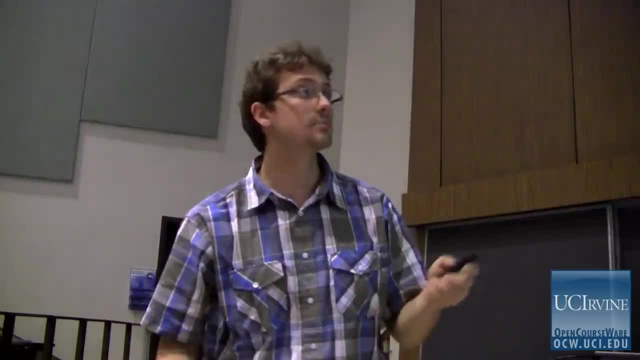 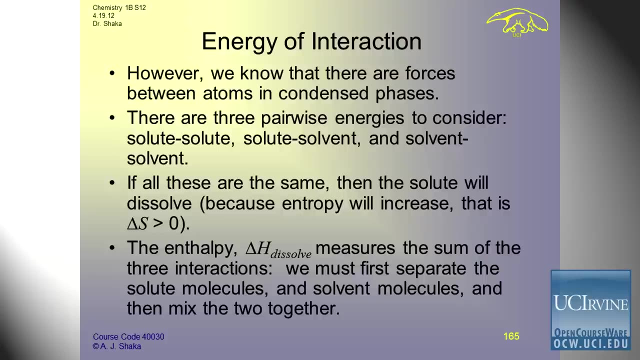 with another sodium chloride. well, it would easily just disperse, just like a gas molecule. So, but we know that this isn't entirely true, right? Just like we know that the ideal gas equation isn't totally true, because atoms can interact together. 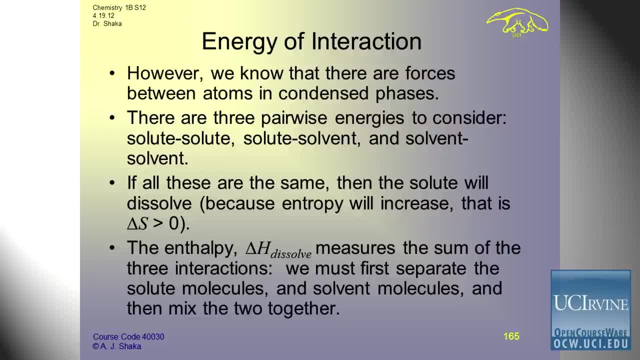 we know that a solute is going to have interactions together. So in sodium chloride, we know that sodium and chloride have that ionic force together. yes, Well, in the crystal there are lots of ionic forces. One, sodium cation, is not interacting. 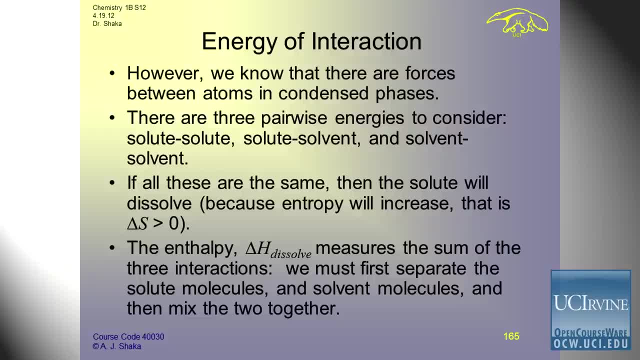 with just one chlorine anion. right, It's interacting with lots of chlorine anions, So there are lots of forces pulling them together. It takes energy to separate one sodium chloride from another sodium chloride. We know that there are forces between them. 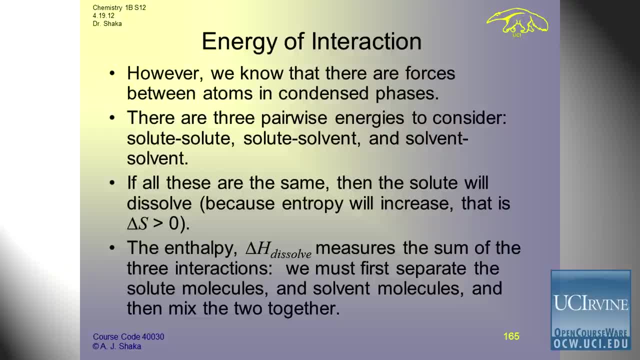 So there are several energies that we have to consider. If I take water and sodium chloride, how do I get that sodium chloride to dissolve? Well, there are solutes, Solute forces, so the solute being sodium chloride and sodium chloride solute solvent forces. 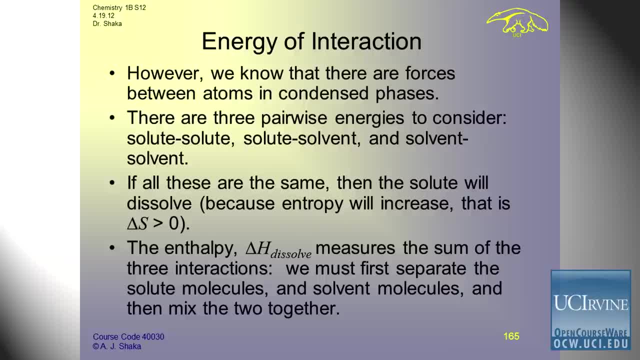 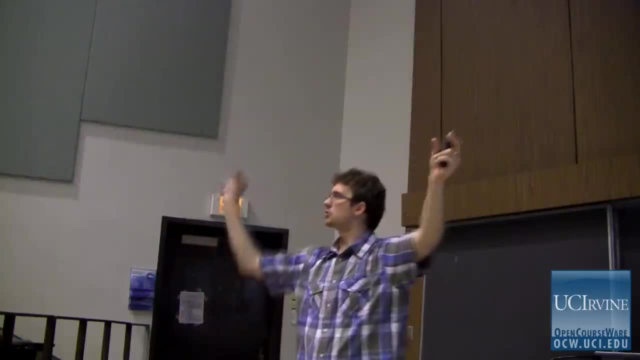 so sodium chloride interacting with water and there's solvent-solvent water interacting with water. For me to get a sodium chloride from another sodium chloride and a water from another water together, I have to break a water-water interaction a sodium chloride-sodium chloride interaction. 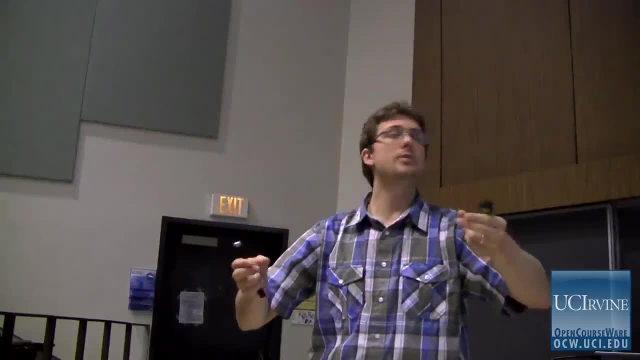 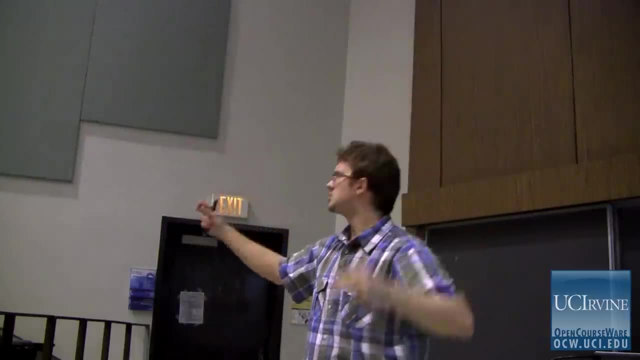 and then put them together. So you can imagine, let's say perhaps for a moment, that sodium chloride and water weren't miscible. They didn't like each other. They do understand it, but they didn't. It would be hard to break sodium chloride, which has a strong bond. 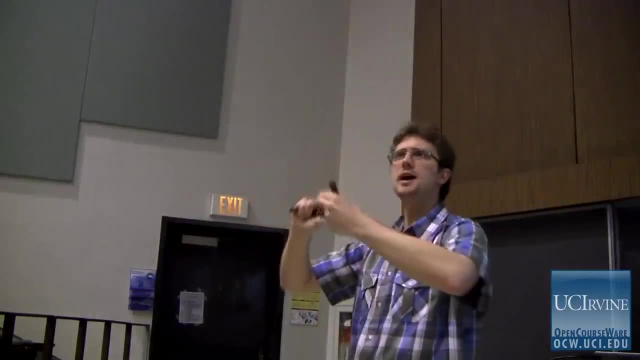 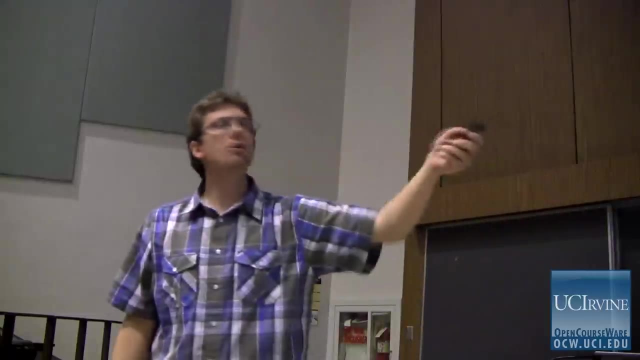 and water, which has a strong bond together, and put them together if they didn't have a good interaction. These are the sort of things we need to consider. So if all of the forces were the same, if water had an equal energy of interaction with another water, 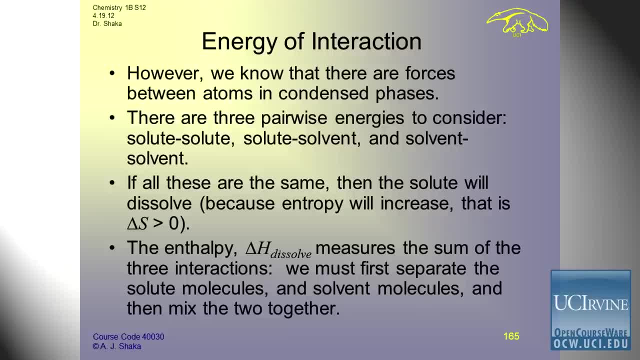 and sodium chloride has an equal energy of interaction with another sodium chloride and they have an equal energy of interaction with each other. then they just dissolve because entropy is increasing. Back to statistics. We have that increase in randomness, So the enthalpy delta H dissolved. 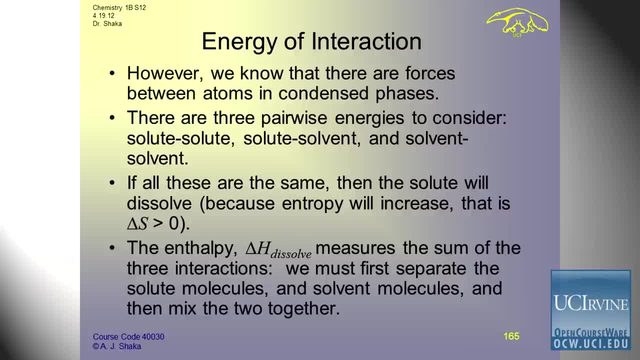 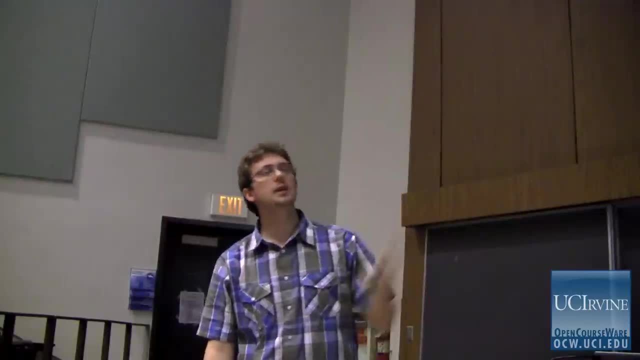 measures the sum of the three interactions. We must first separate the solute molecules, so that sodium chloride-sodium chloride, and the solvent molecules, that water and water, and then mix the two together So water has a network of hydrogen bonds. 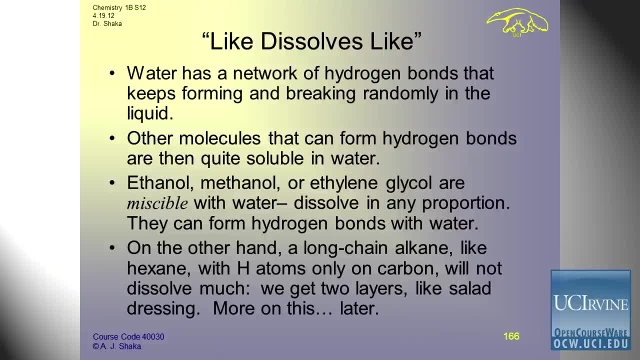 we should know this by now- that keep forming and breaking randomly in the liquid. So that's something I have to consider. When I break that water-water interaction, it's not just dipole-dipole, There's also the hydrogen bonds. 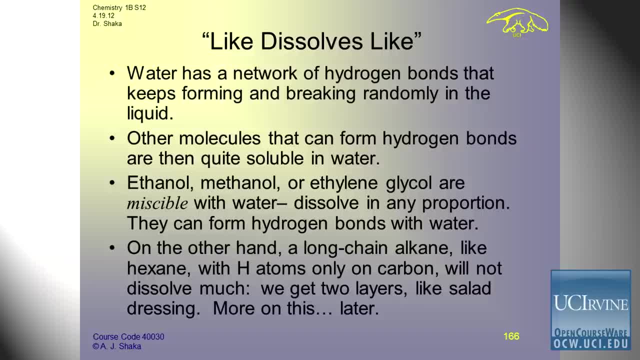 We already know that water has a strong intermolecular force, right, So I have to break that first, and that costs energy. Other molecules that can form hydrogen bonds are then quite soluble in water. So, yes, Can you slow down a little bit? 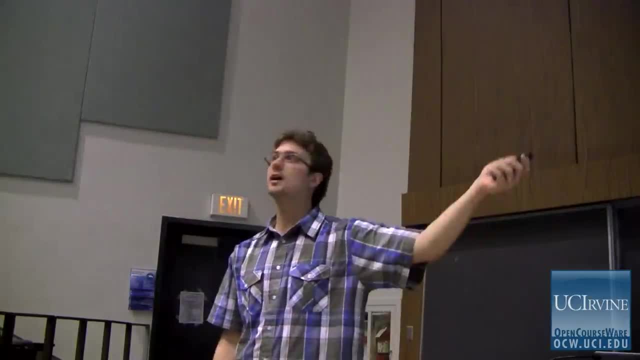 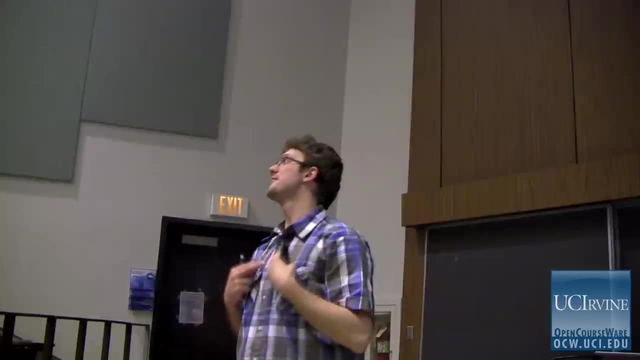 Oh sure, Can I go one or two faster, you guys? Yes, Ah, you want me to back up a few slides? Just tell me when, When, When I heard it. OK, All right, This is my first time. 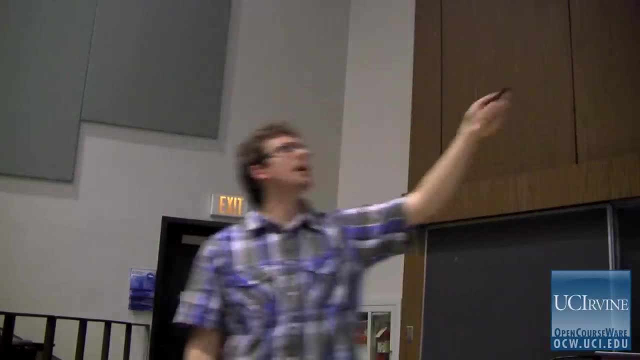 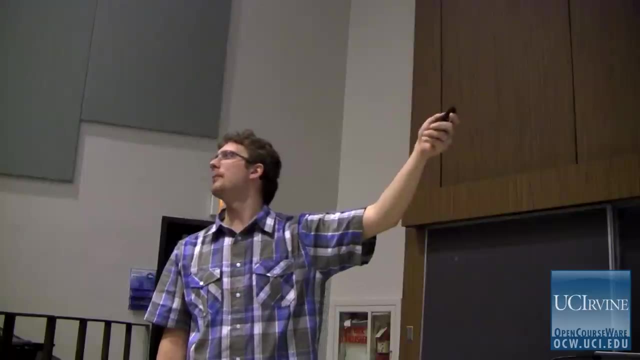 Be gentle. So let's see, We're at energy interaction. Let me go back a couple slides and we'll go through it again. OK, All right. What's funny is I heard Mohamed with you quickly and I was like: not me. 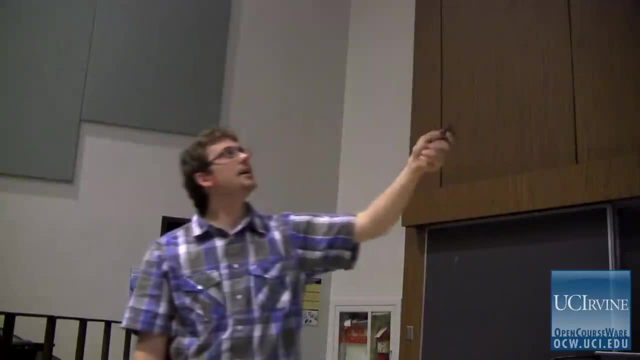 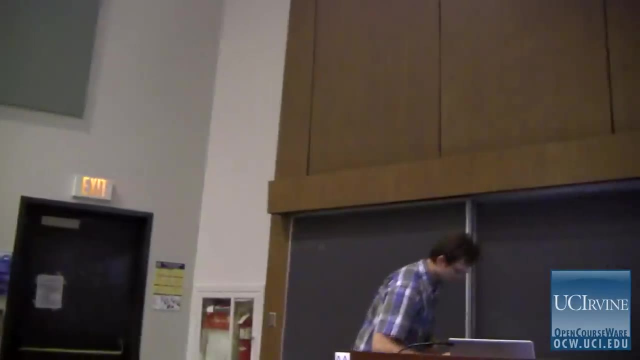 Not me. I ain't going to have you All right This way. That's this way out. Do you want me to? just What time is it? I got plenty of time right. All right, 11.24.. 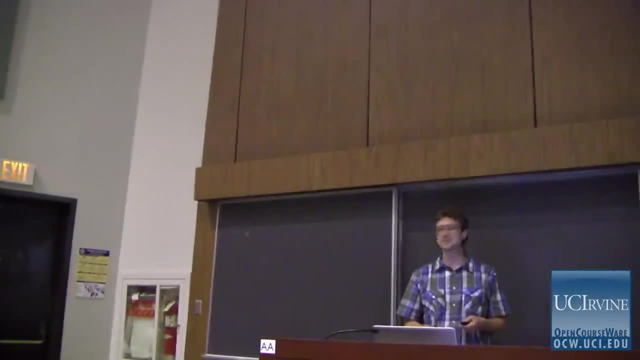 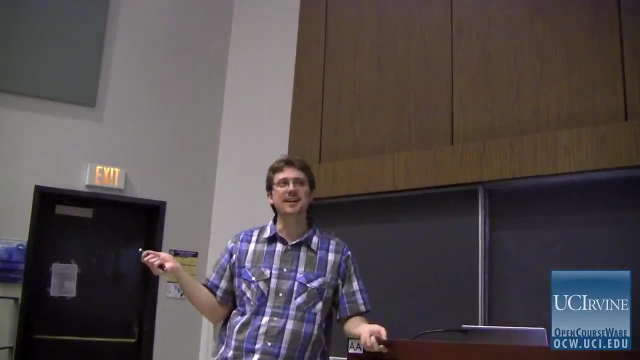 Wow, 24 minutes have passed and I know that's most of the slides. Well, keep it down. So Mohamed went through most of my slides. That's my excuse, But we do have some sample problems. at the end, some review questions for the exam. 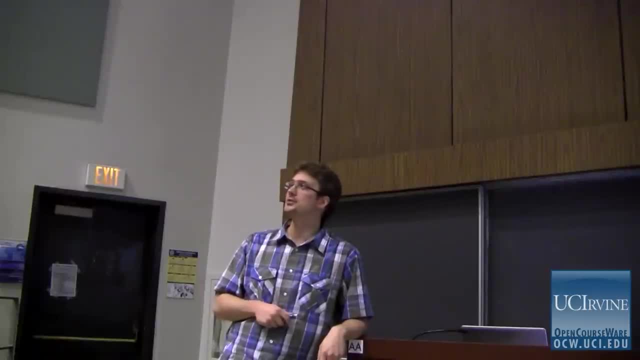 and we're going to go over those as well, And that will take up some time. Or we can just have light conversation. Fine, I'm down for anything. So I haven't been keeping track of the website. Has he gotten the other ones up yet? 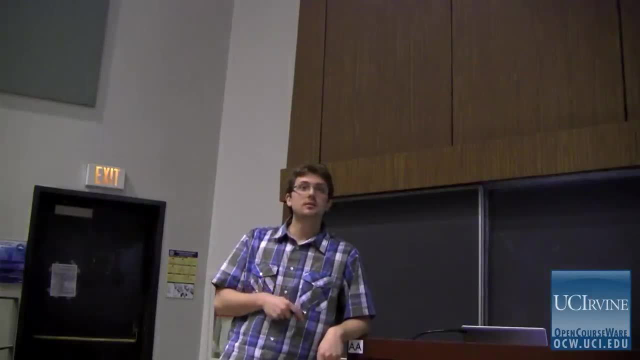 No, Up to lecture four. What was that? So the slides for up to lecture four are on and we're at lecture like six, right With the videos I posted on this. That's true, So he hasn't been here all week. 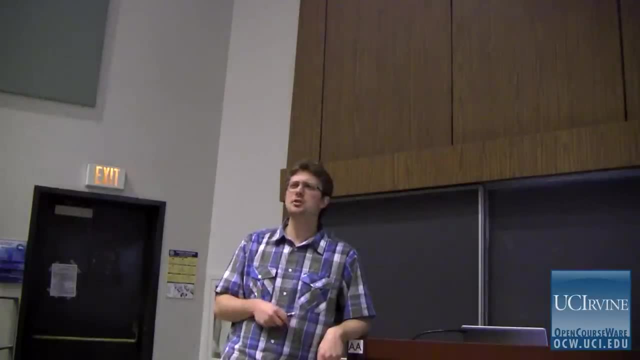 So I anticipate he'll have the slides up. OK, All right, Well, I'll make sure to ask him about it too. Yeah, Good, I'm glad we had this talk. OK, So we have. it's only 11.24.. 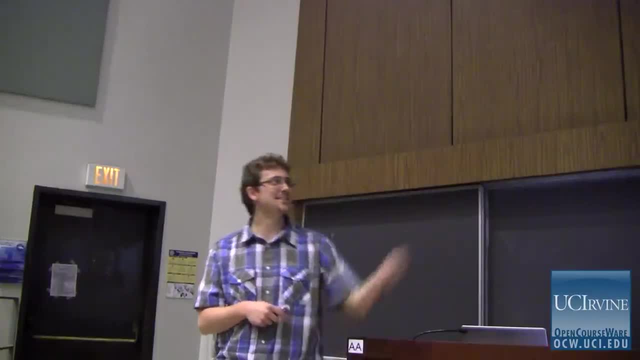 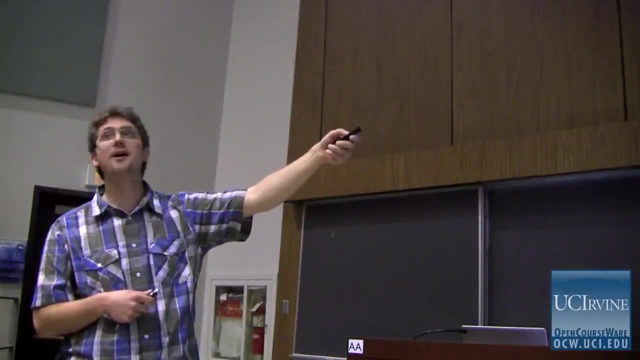 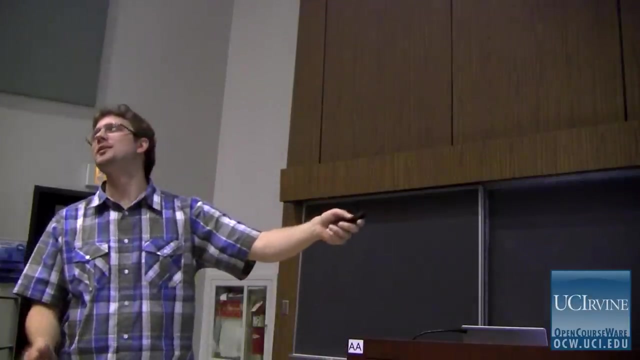 All right, Let's go through this again. All right, OK, Too far. Yeah, You guys are never happy with anything. OK, OK, We're good, We're good, We're good. No, I'm getting mixed signals from everyone. 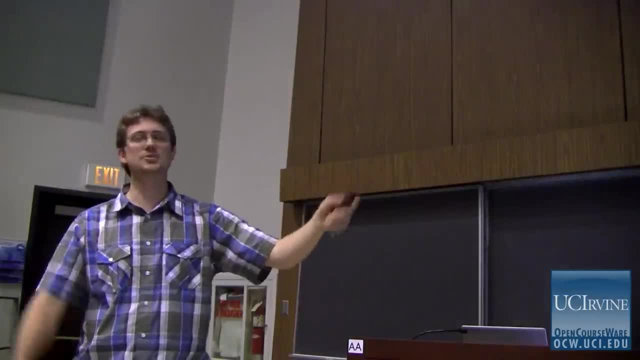 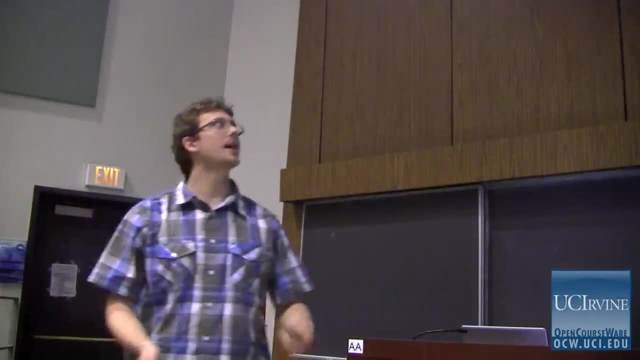 More, More. OK, We're going to start here. Anyone has a problem? get out and leave. OK, We're going to start here. I'll go through it again a little more slowly, All right, OK, So counting configurations. 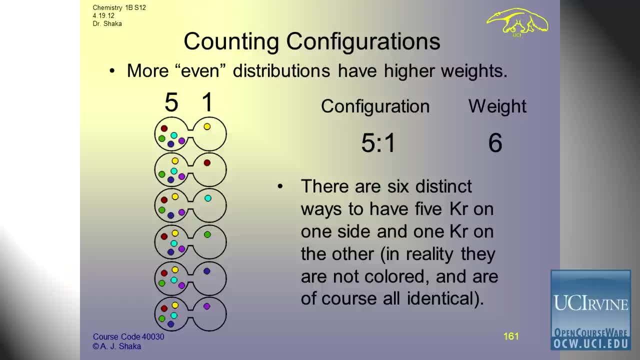 Remember, we're talking about these two containers. Yeah, All right, All right, Yeah, Thank you. OK, This is all on video. You're making me look bad, Anyway, OK, So we have two containers, right? And what did we do? 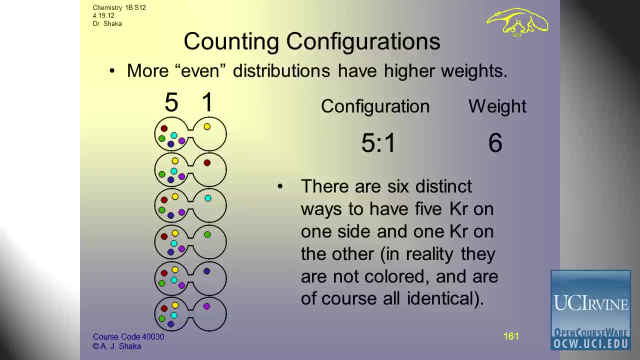 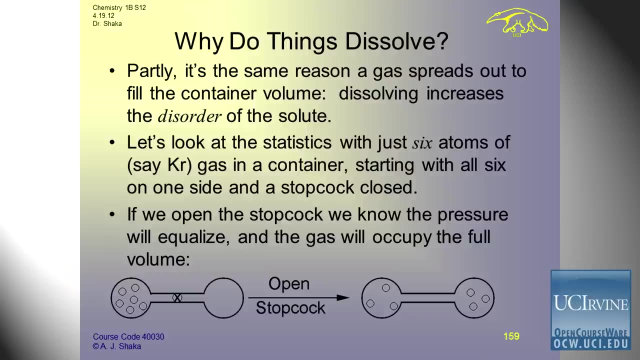 We took one container that had six atoms in it And we opened it up to another container that had zero. Just by statistics, we know that this is going to become equal. As I mentioned before, when we open up this container at first- and we had six on one side- they're crashing around randomly. 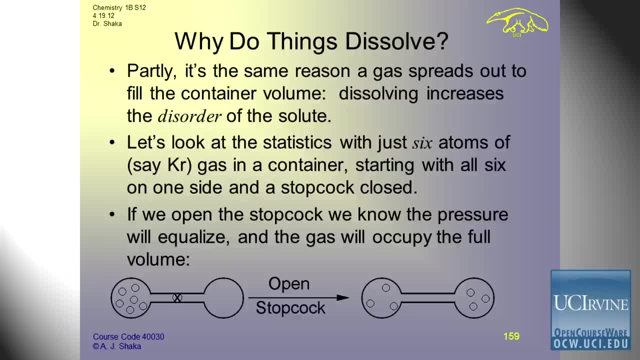 And they're just going to, by statistics, eventually find this hole and make their way to the other side. This is going to keep happening until we have an equal amount going from one side to the other and an equal amount coming from that second side to the first. 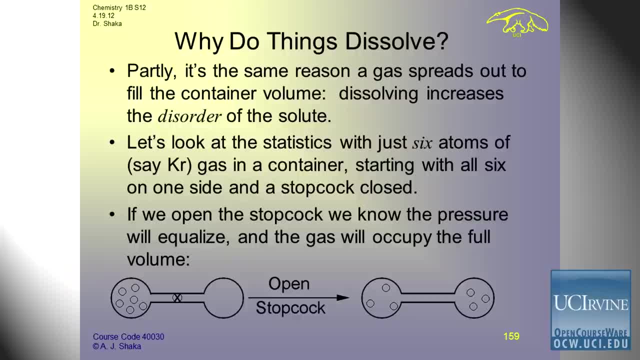 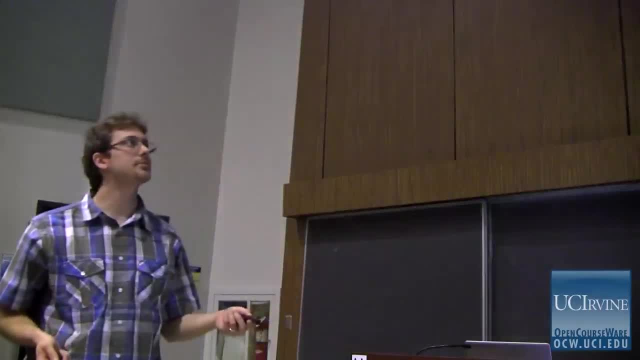 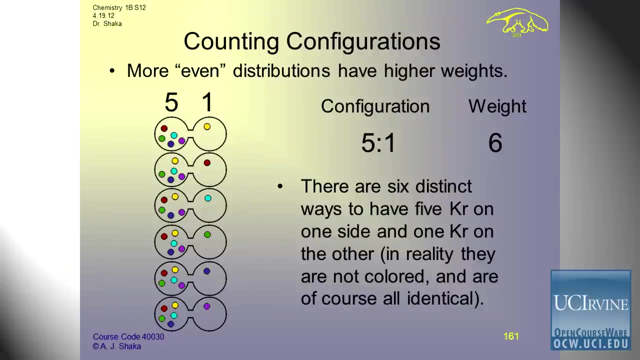 It's an equilibrium. We have three on, each One switches to the other, Another switches back And so forth, But this is only with six atoms. So OK, This is only with six atoms. So in this distribution where we have five to one, 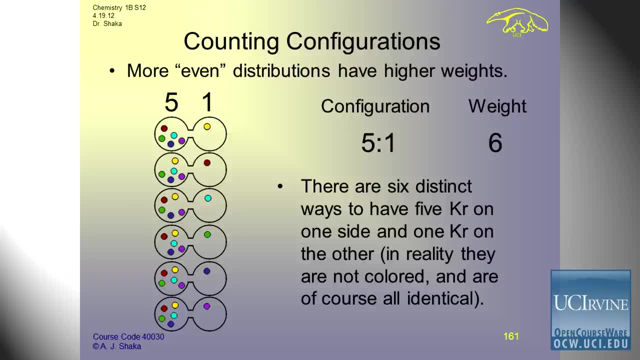 five on one side and one on the other. this configuration label is five to one, Five in the first container and one in the other, And its statistical weight is six. There are six ways that I can put five on one side and one on the other. 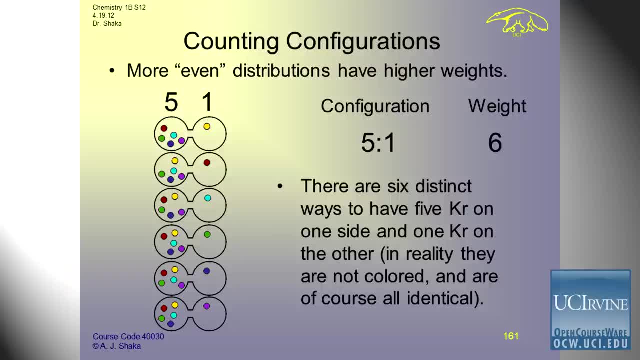 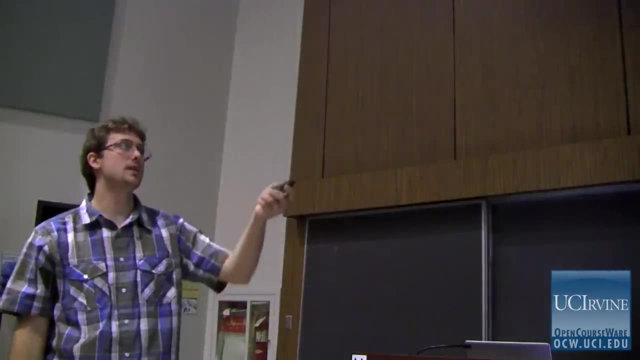 Right And I want to do a one to five. So one on one side, Five on the other. That also is going to have a weight of six, But it will be five on this side and one on the other. So we have to consider what are all the possible ways. 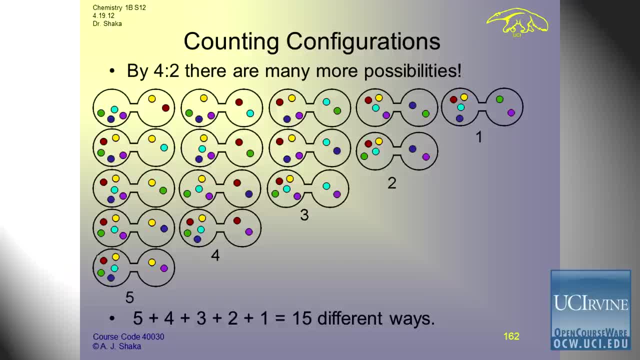 for me to arrange these atoms. So, with four and two, continuing that line of thought, we have 15 different ways where four are on this side and two here. So green, blue, blue, purple, right, Yellow, red, You just switch one of them. 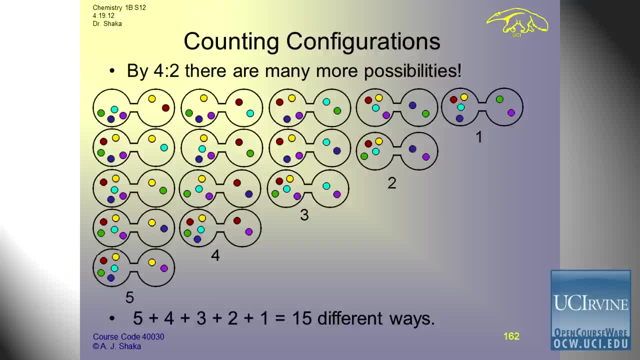 Keep the red on here, But switch the yellow with that light blue one. That's a whole different configuration, A whole other possibility for these atoms when we consider their randomness. Continued on. there are 15 different ways to arrange four or, excuse me. 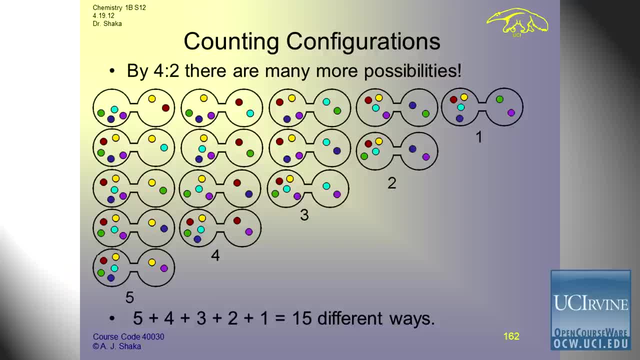 four and two. Those have four, two, That one has one, two, three, four, five, one, two, three, four, five, six, seven. Oh, Error. I'm glad we redid this. I'm sure this is why you were all confused. 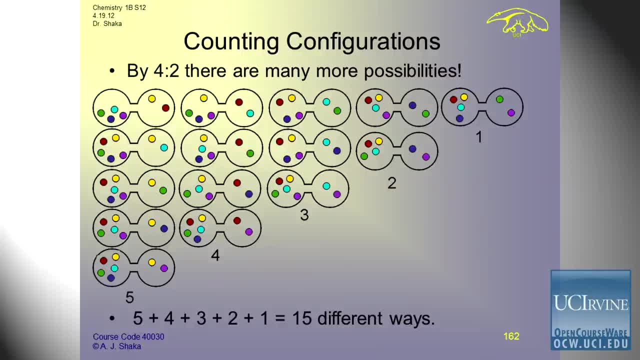 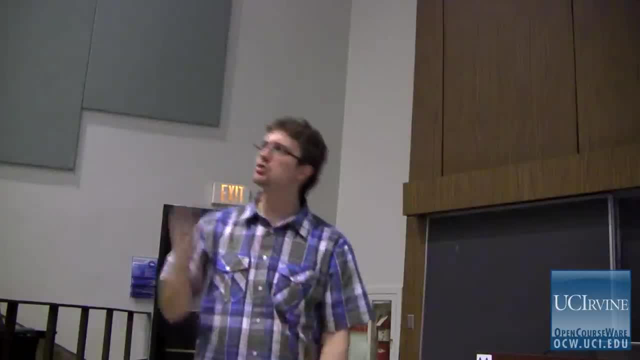 So, in any case, ways to put four and two, 15 different ways, And then for the three and three, there are 20.. You can do this yourself. When the numbers are small, you can just write out all the different combinations and add them up. 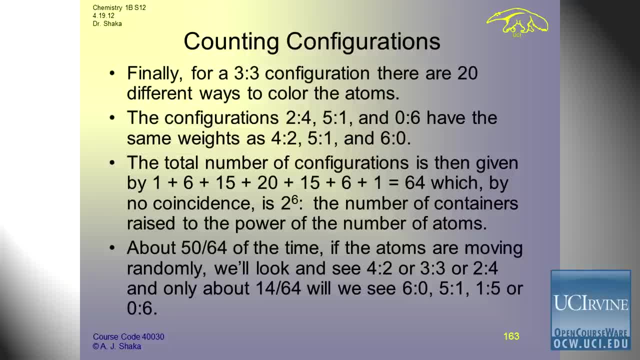 If you like math, I will. So for that, three for three, there are 20 different ways to color the atoms. But then those configurations of two to four, five and one and zero and six. as I mentioned, they have the same weight as four to two, five to one. 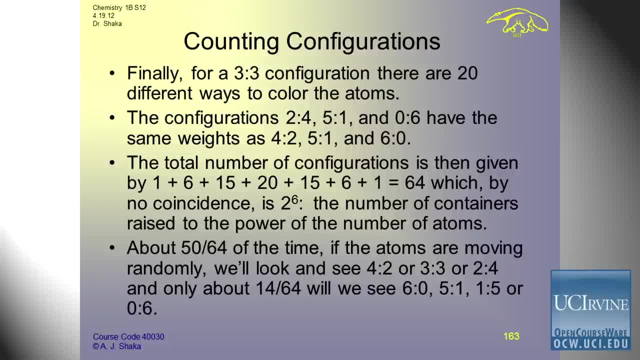 There's another typo, I didn't write this. So two to four and five to one. First container has two. Second container has four. That has the same as the first container having four and the second container having two. This one five and one has the same as one and five. 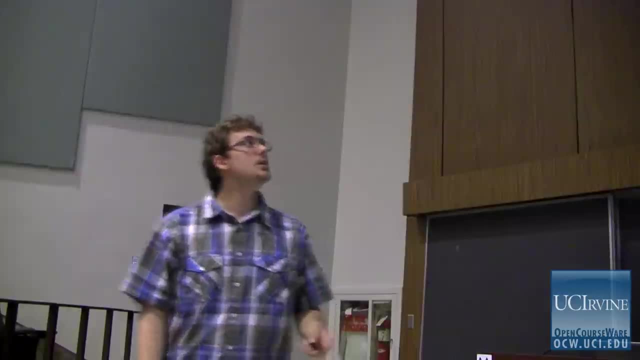 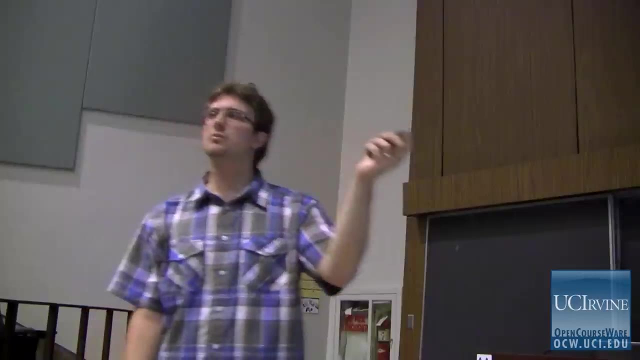 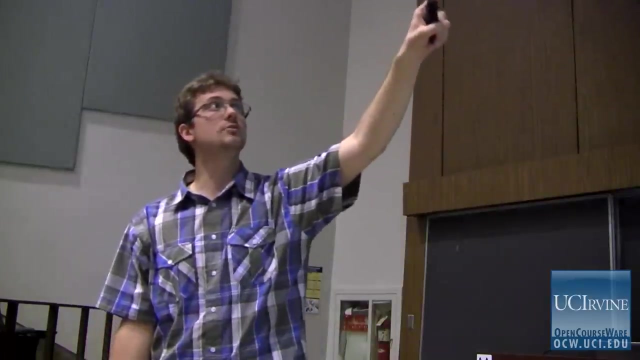 And then zero and six, Six and zero. Why wouldn't each one have the same weight? Let's go back So two and four, five and one, zero and six. right, Why don't each of two and four, five and one, zero and six? 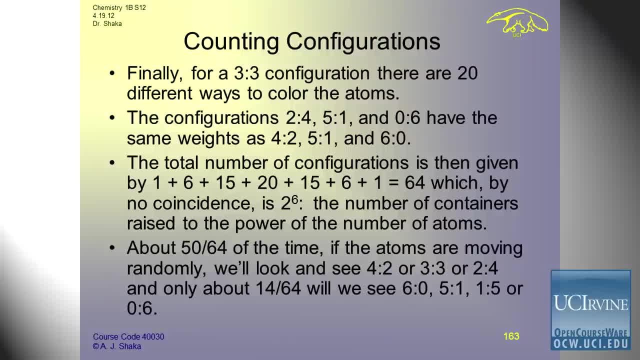 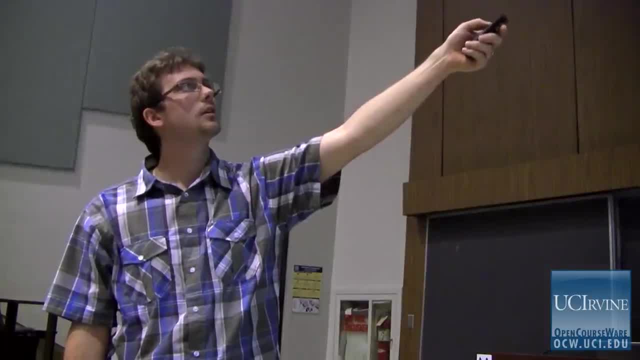 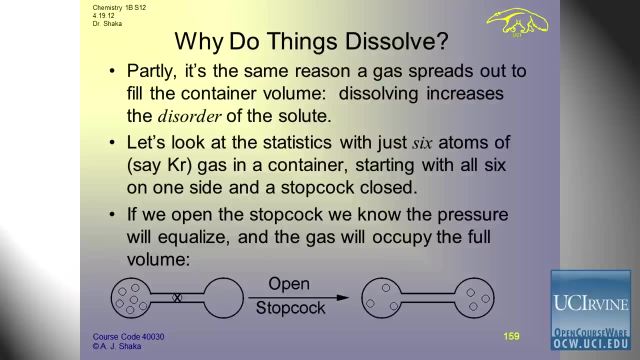 have the same weight. Yeah, they're all six atoms. So let's go back to the images. So compare six to zero. If the atoms are moving around totally randomly, there's only one possible way for me to have six and zero. 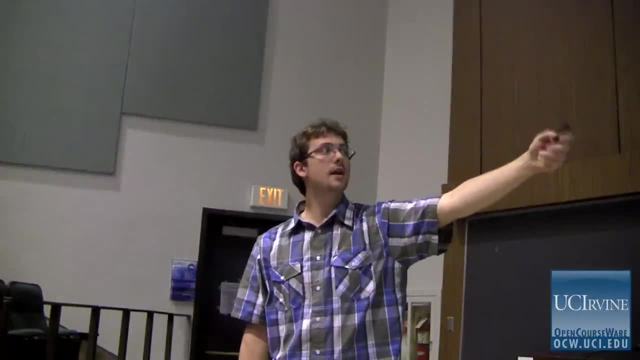 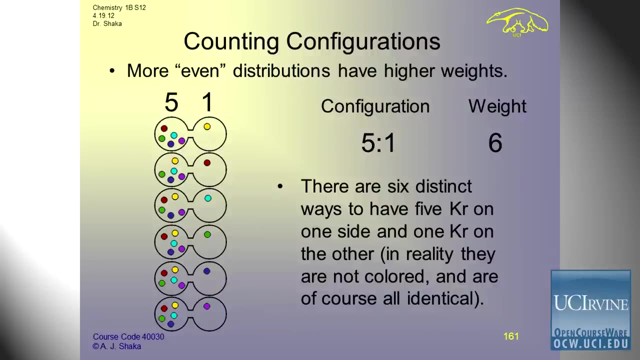 with six in the first and zero in the second. If I go just to five and one and we'll go back and forth between this, there are six different ways to do this. So if I just take a snapshot of this gas- totally random- 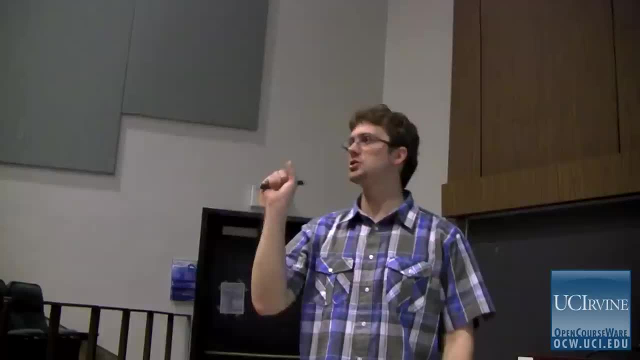 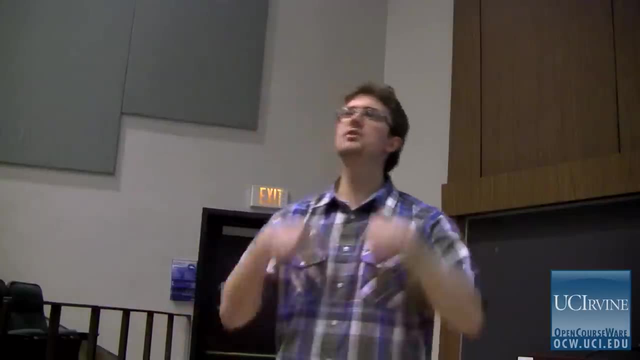 if I took a million snapshots, I'm going to get a statistical distribution between whether my snapshot sees zero and six or five and one. If it's totally statistical, based on what the chances of me seeing six and zero or five and one? I know that six times more often. 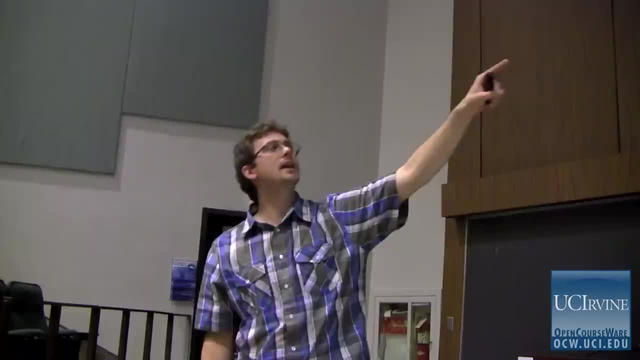 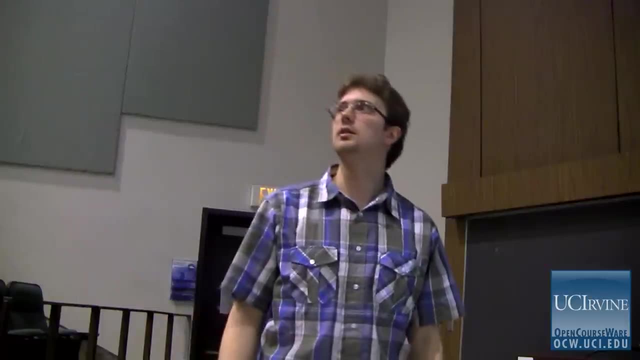 I'm going to see five and one, just because that is more likely. There are more configurations for this than for six and zero. So I think- kind of going off this question, that they don't mean actually the weight as in the traditional sense we mean it. 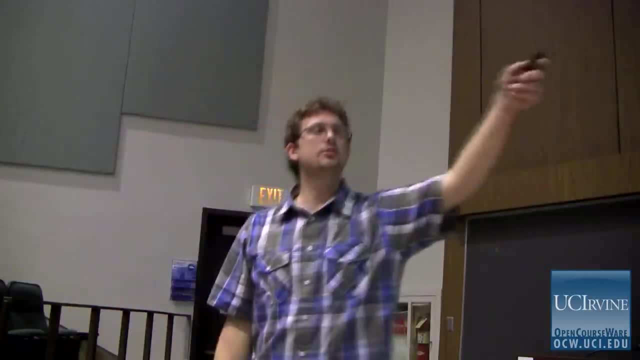 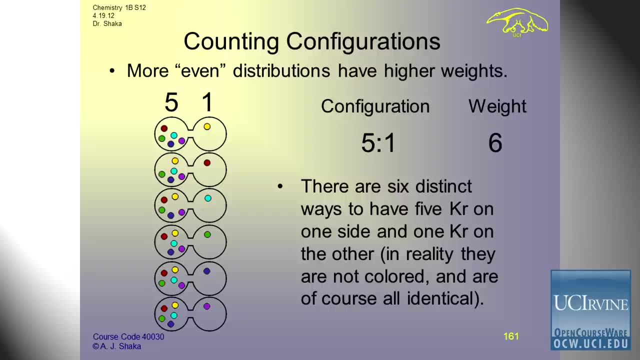 It's more like this in this case. Yeah, I must have said it quickly earlier. This weight is not a mass. Yeah, sorry, I was blazing through before. This weight is not a mass at all. This is a statistical weight. 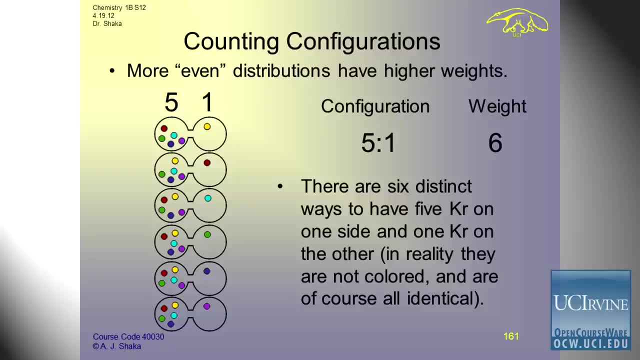 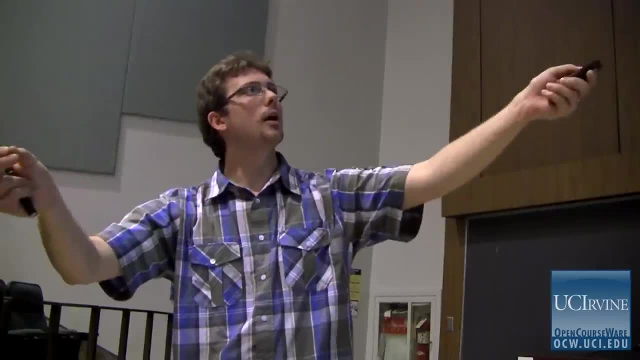 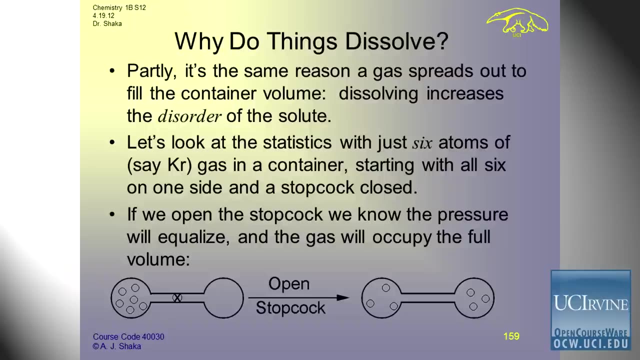 It's saying contributed to all the possible configurations. this is just a number that represents. what chance do I have of seeing this situation? So, going back by one, this has, this has a weight of one. There's only one chance of having six and zero. 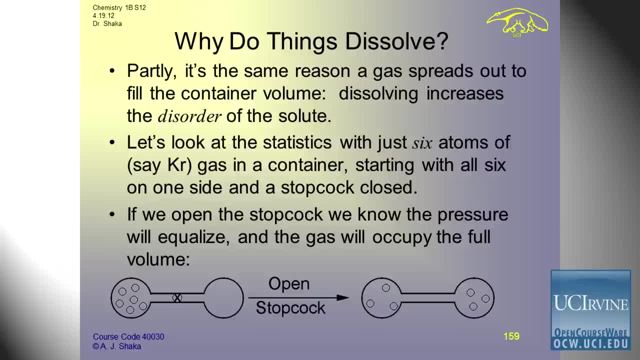 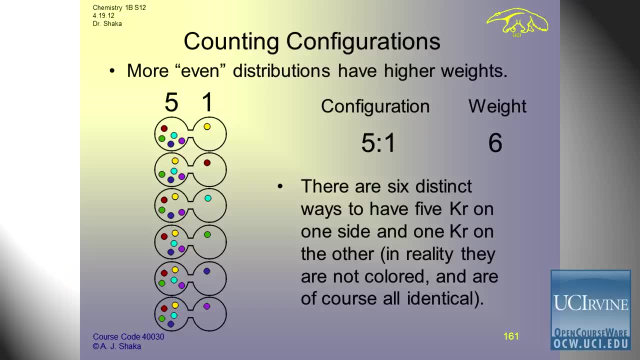 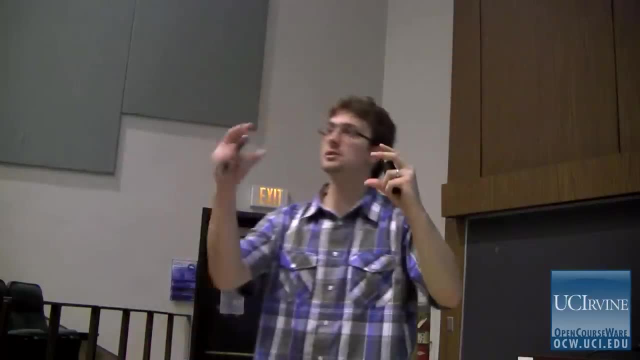 One possibility Going on to the next. I have five possibilities of having five in the first and one in the second, And so this has a statistical weight of six. It's six times more likely to see this than six and zero. Okay, does that answer your question? 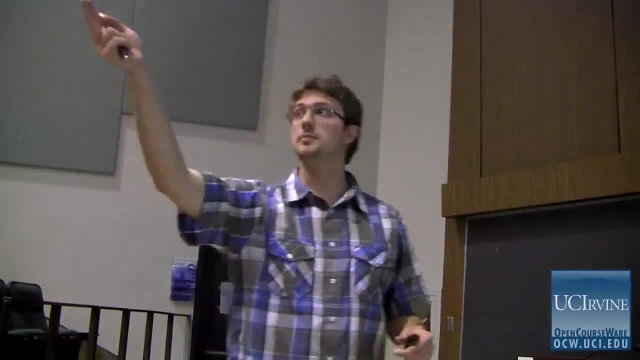 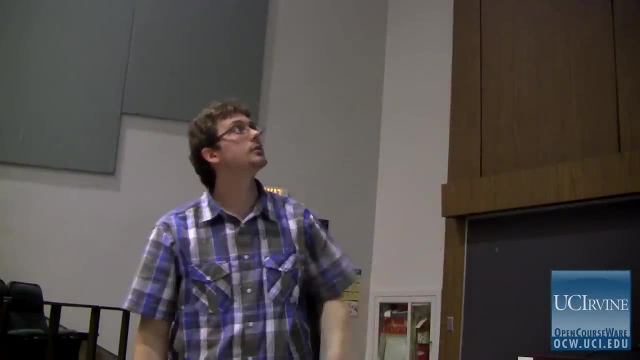 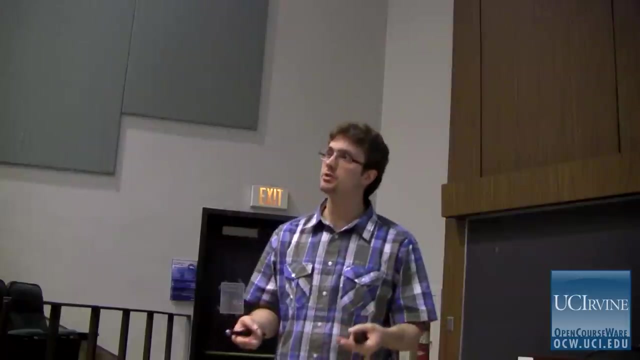 Yes, Okay, Thank you for bringing that up, That people have missed that. The weight thing. So four and two. So you can see, as we were just talking about, U of five is one, right, There's five possible configurations. 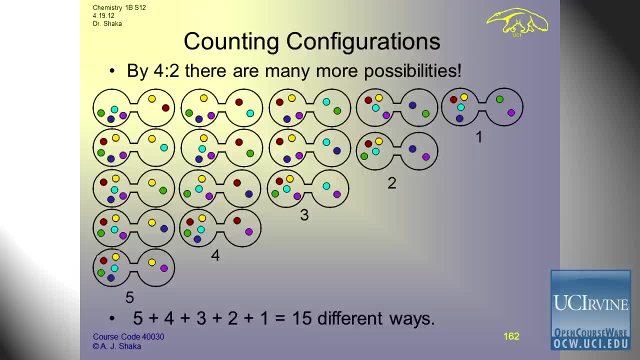 Take that a step further, Go to four and two. Here are all the possible ways for me to write four and one and two. in the second There are 15 different combinations. So if the atoms are totally at random going to have some configuration. 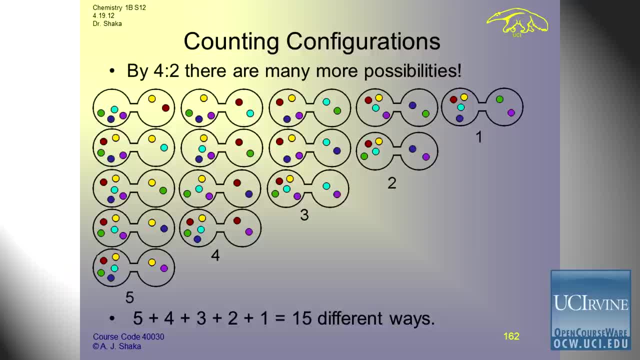 I have 15 different ways that show me this exact arrangement. Remember these atoms, all the different colors, they're still just one atom. They're all just krypton. So if I took a picture of this right now, I wouldn't be able to distinguish. 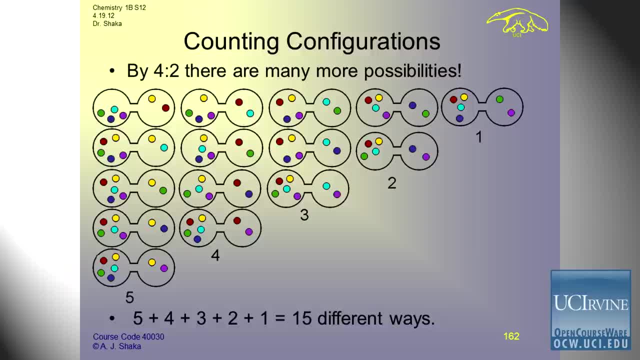 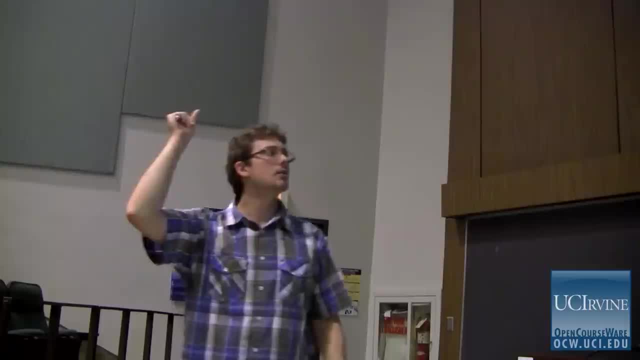 the top left, from the bottom, from any ones in the right, They would all look exactly the same to me, And so I would count that as another one of my four and two. That's a second count, And if I keep doing that, 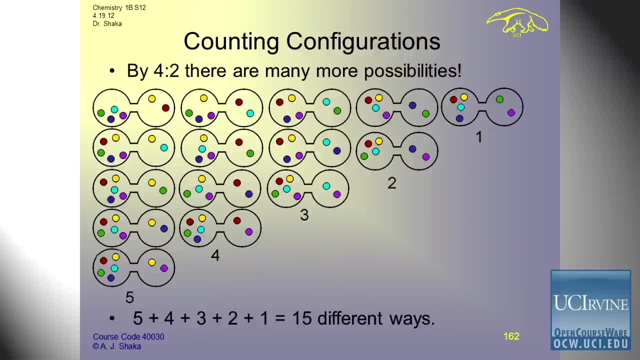 snapshot, snapshot, snapshot, over and over again. I'm going to have 15 different possible ways to see four and two, but only one possible way to see six and zero. And that's where this comes from, That's where the statistical reasons. 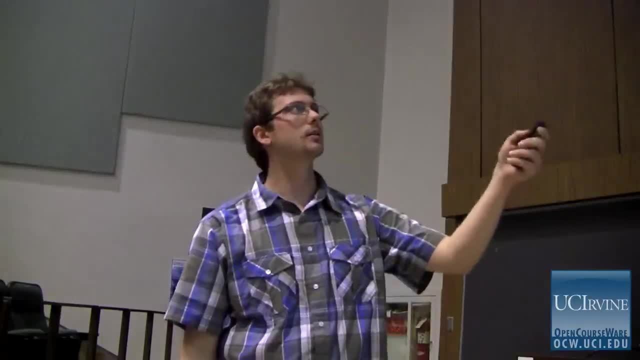 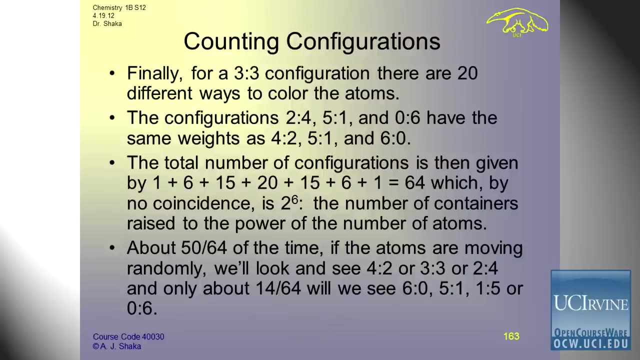 for equilibrium come from. So for that three and three, which is taking the same thing to the next configuration, there are 20 different ways to color those atoms. And then you were asking why they don't have the same weight. So the configurations. 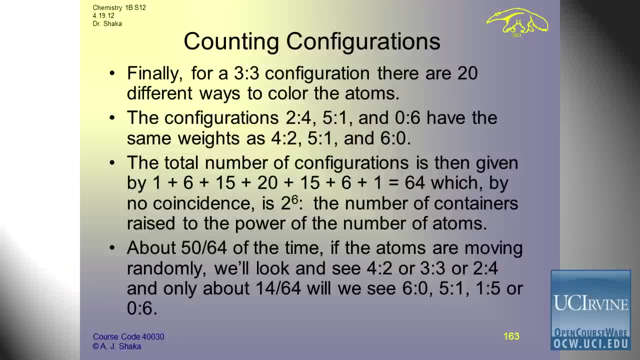 well, no, I already answered that question fully, I suppose. So the configurations two and one, four and the other, five and one, one and the other, and zero and one and six and the other, those have the same weights as flipping your diagram. 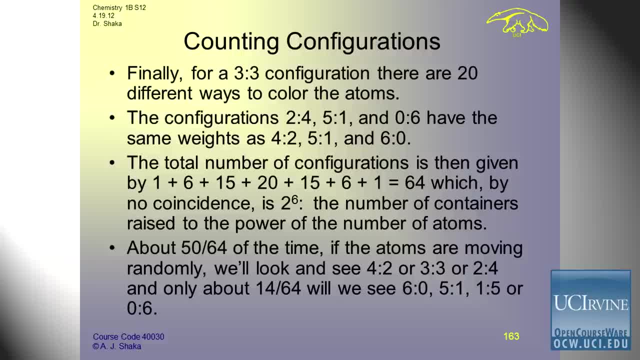 So six and zero has one possible configuration, And zero and six has one possible configuration. Together. I have two possibilities of ever taking that image and seeing six in either with zero in the other. So the total possible, the total configurations that are possible, are 64.. 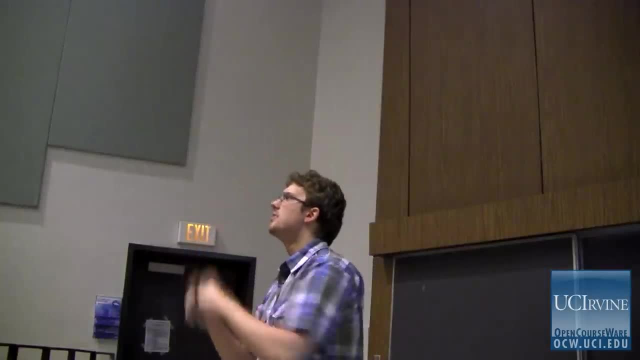 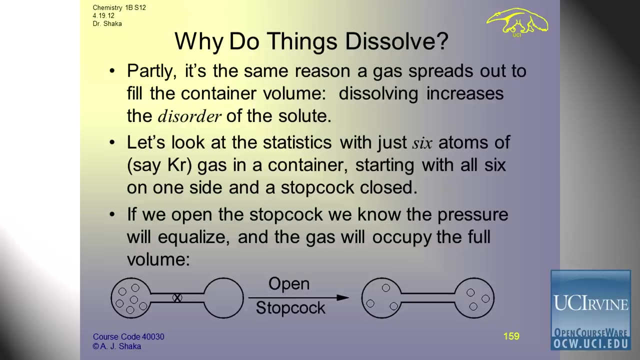 So let's think about that six and zero. I take a snapshot. There are two in 64 chances that I will take a snapshot with six and one and zero in the other. It's very small And if I have I'll go to the next page. 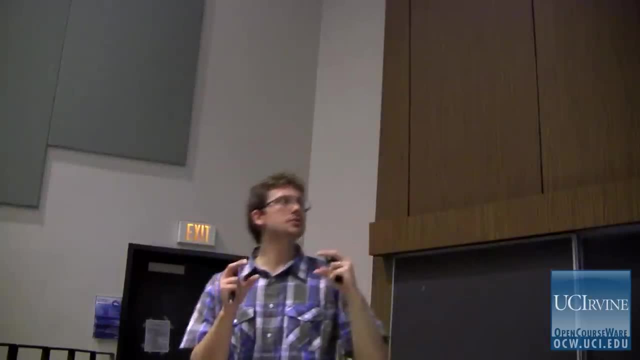 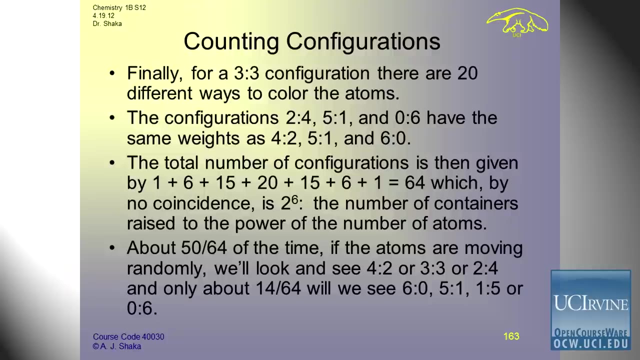 Here we go, And 50 out of 64 of those times, if the atoms are moving randomly, we'll look and see that four in one and two in the other, Or three in one and three in the other, Because what I'm doing 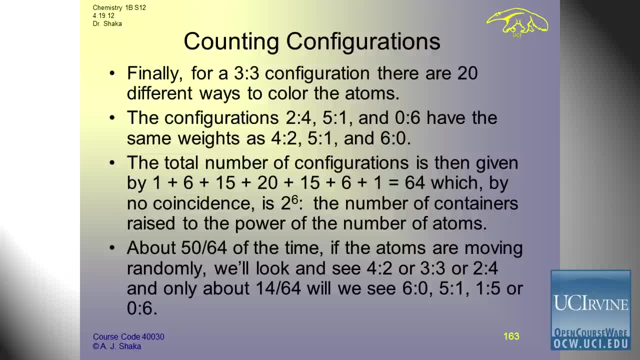 is adding the 20.. So remember, 20 corresponded to three and three. right, So three and three, plus the chances to see four and two. So four and two, that was 15, right, So four and two, 15.. 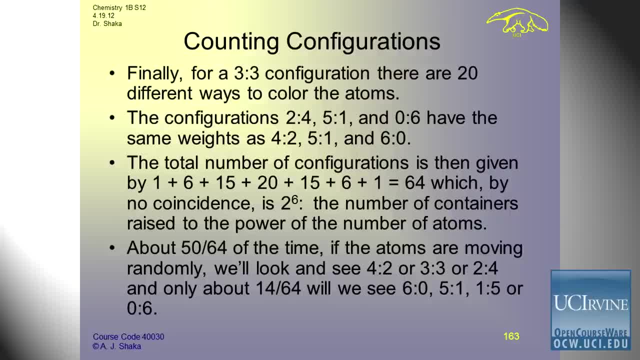 Three and three, that's 20.. And two and four, which is another 15.. That's how many, right? That's the sum? Four and two, 15.. 15,, 30,, 50.. 50 out of 64 times. 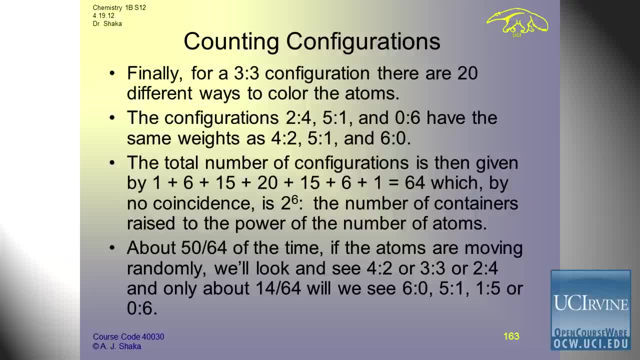 I'm going to see one of these, And 14 out of 64 times we'll see six zero five, one one five or zero six. So the six and the zero right That contributes one. 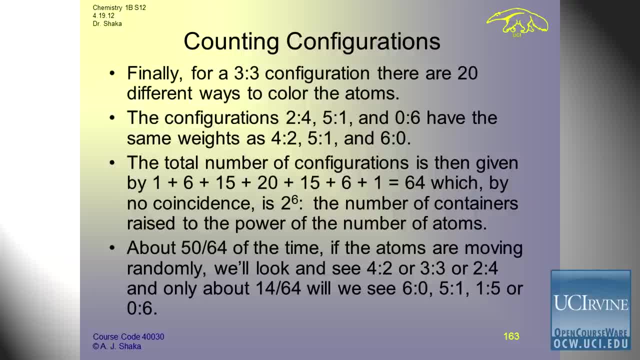 The zero and the six that contributes another one, The five and the one that contributes six, The one and the five that contributes six. Total 14 out of 64. So the chance of me seeing very few on one side. 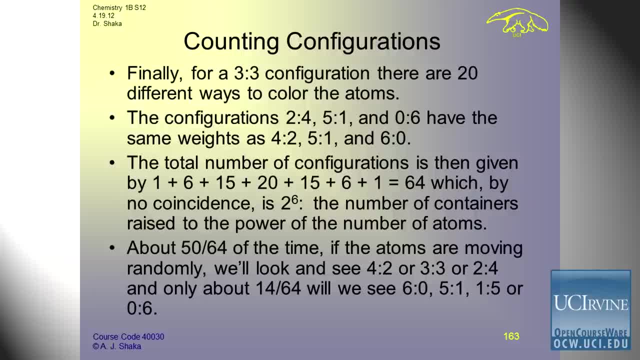 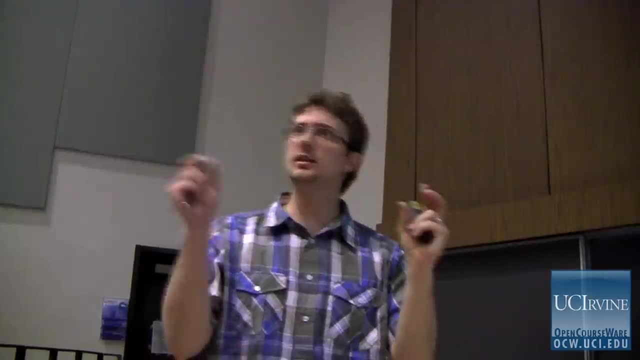 and more on the other is very small, Only 14 and 64, when I only have six atoms. Since the number of possibilities increases exponentially, the chance of me having most of a gas on one side and little gas on the other. that becomes completely insignificant. 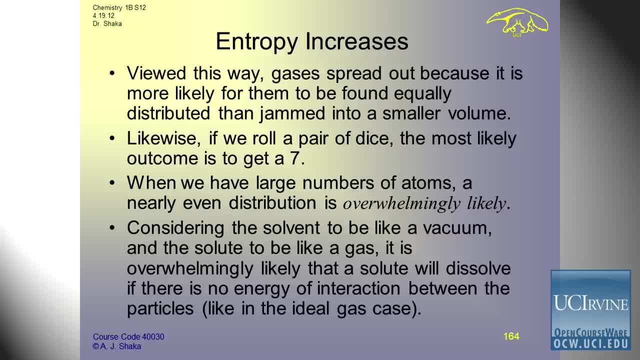 and we don't even consider the possibility. So they spread out because it's more likely for them to be found. equally, If I take a million atoms, the chances of me seeing a half a million on one and a half a million on the other. 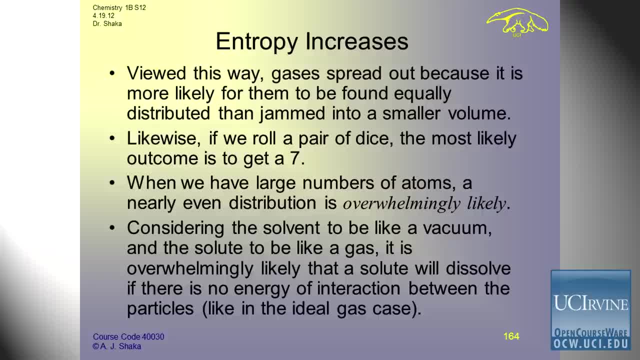 that's incredibly high. Of course, you know, give or take a couple atoms. Likewise, if you're a gambling person, we roll a pair of dice. the most likely outcome is to get a seven Quick tangent. Went to Vegas for my first time. 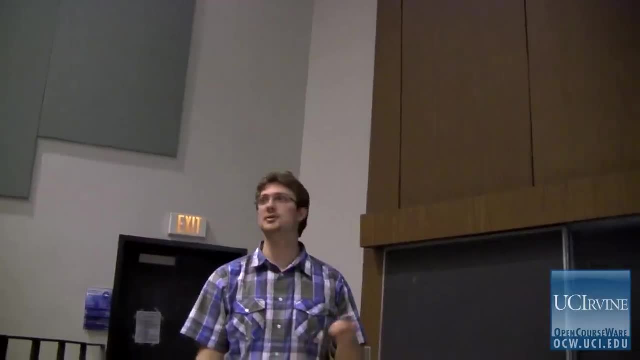 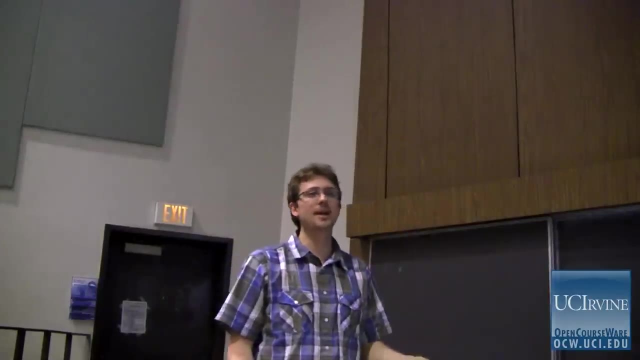 a few weeks ago for my anniversary, Bet $100.. Lost it all. Never do that again, Thank you. I know It was roulette. I'm stupid. I know Who plays the roulette table. you're going to lose. I was up 60. 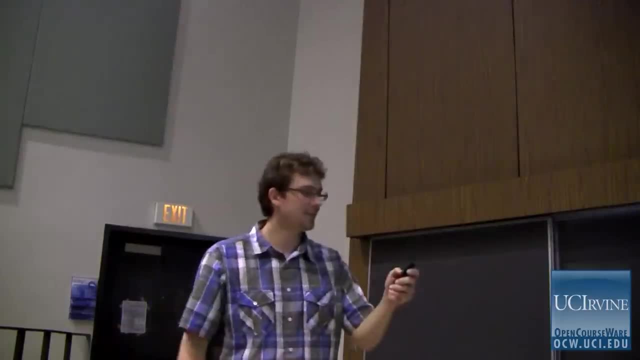 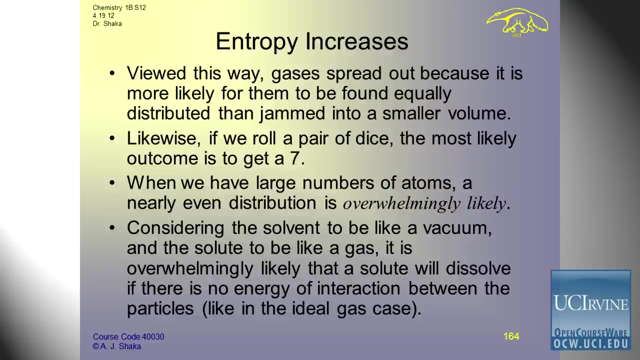 and then 10 minutes later, I'm down 50. I don't know how it works When we have large numbers of atoms. a nearly even distribution is overwhelmingly likely. So considering that solvent to be like a vacuum, as we were mentioning before, 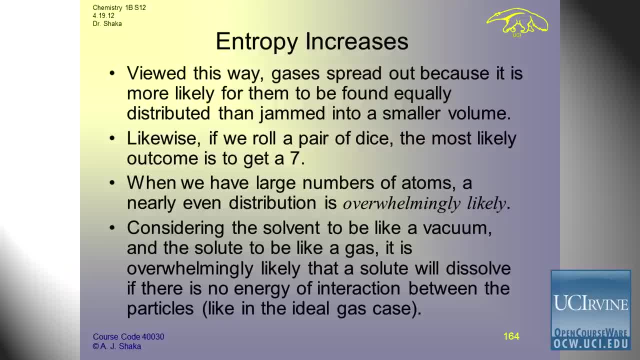 and the solute to be like a gas. it is overwhelmingly likely that a solute will dissolve if there is no energy of interaction between the particles, like in the ideal gas case. So let's picture this again. I have that beaker of water. 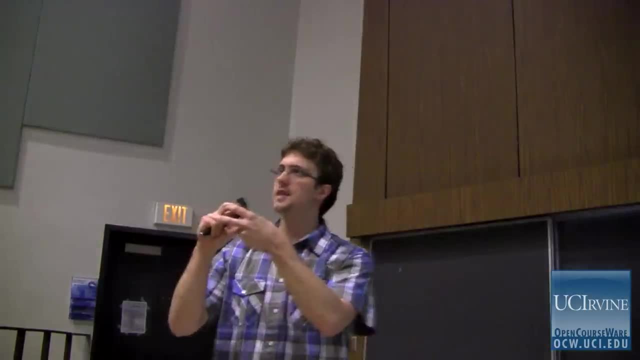 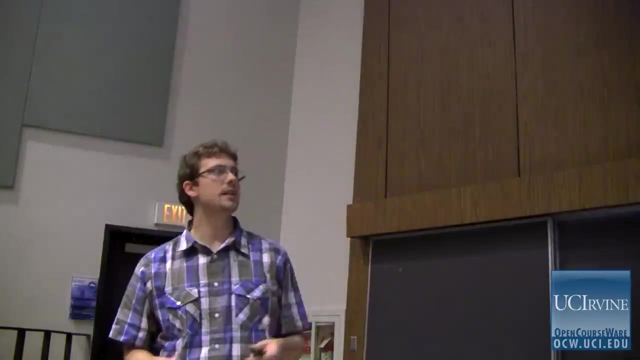 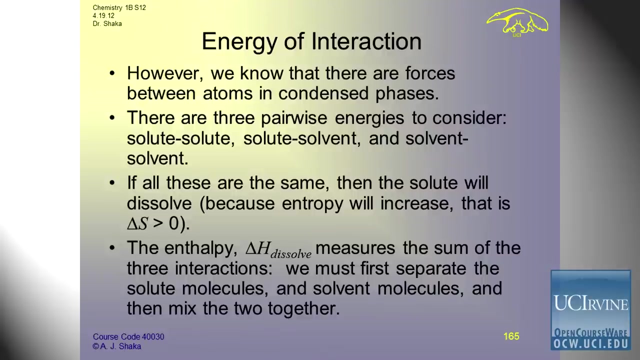 with a bunch of sodium chloride just sitting in the mass. It's not likely for that sodium chloride to just sit in the mass as long as those interactions are the same, like in the ideal gas case, No energy of interaction for sodium chloride. However, we know that there are forces. 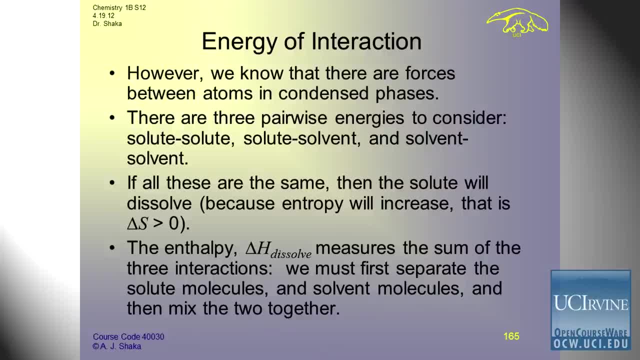 between atoms in condensed phases. As I was mentioning earlier, we know that sodium chloride has an interaction with the atoms And we know that in a sodium chloride crystal, that sodium chloride is interacting with several other sodium chloride And it's hard to break them apart. 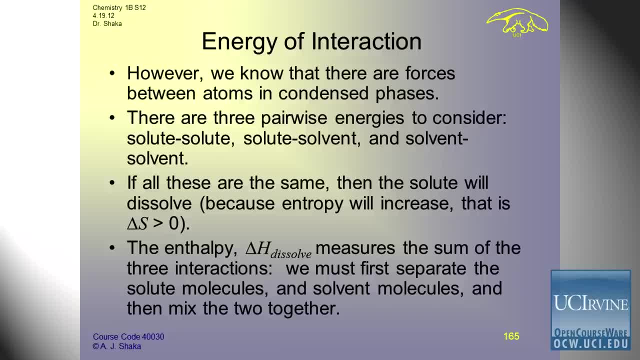 They have strong ionic forces that require energy to break one sodium chloride from another sodium chloride. So there are three pairwise energies to consider Solute-solute. that's the wa- oh, excuse me, sodium chloride in this case. So breaking apart sodium chloride. 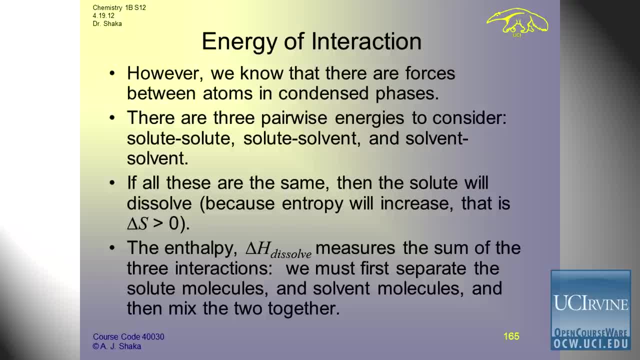 from another, sodium chloride, that takes energy, The solute and solvent. when I take that sodium chloride and water approaches, then we have interacting forces And in the case of water and sodium chloride, that's a positive energy, it's favorable. 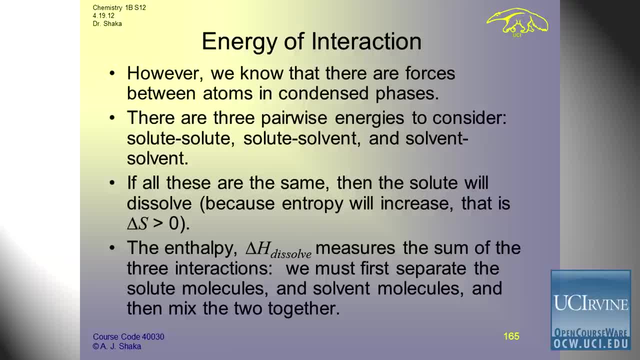 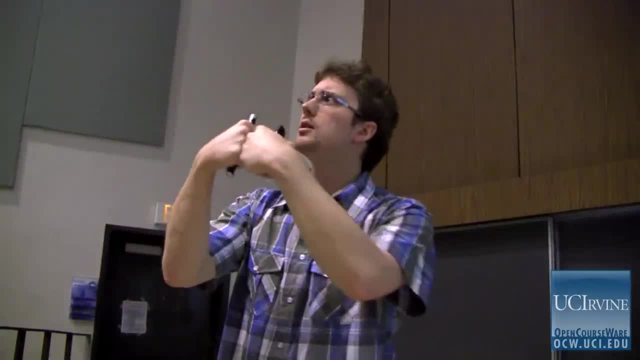 So those attract And I have solvent-solvent. so water and water. Like I mentioned before, water, we know, has very strong ionic forces, So I have water. it takes energy to break that apart. So I have two unfavorable energies. 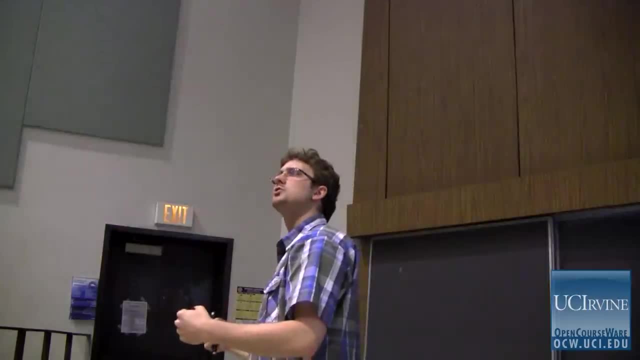 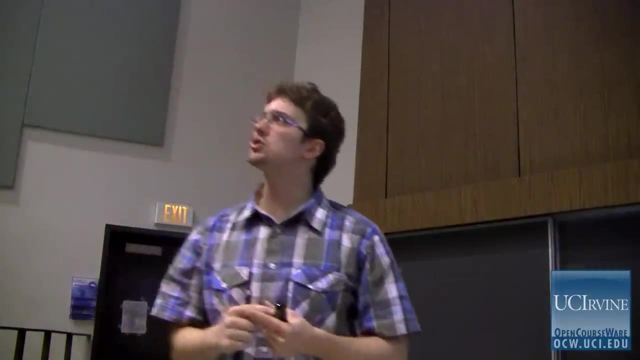 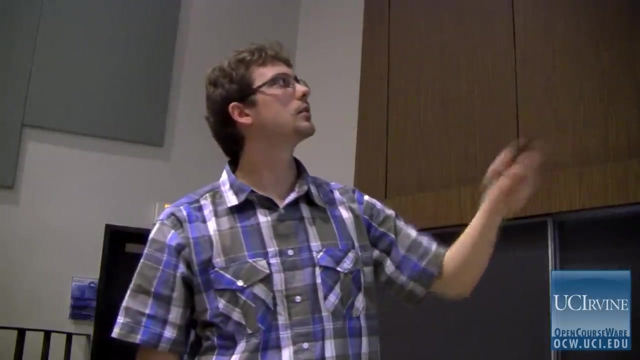 breaking water away from water, breaking sodium chloride away from sodium chloride and I have a favorable energy Taking sodium chloride and interacting with water And if that interacting energy is strong enough, it can overcome the energies that I'm having to break. So if all of the energies 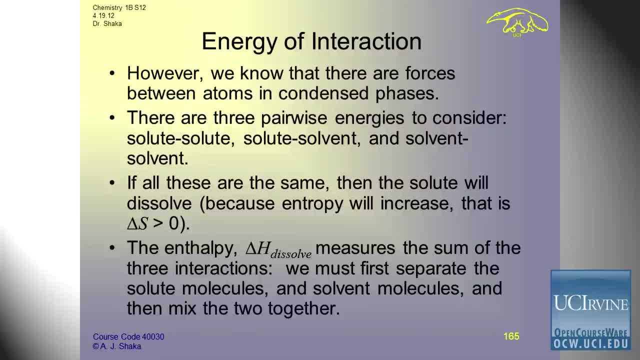 are exactly the same. then, breaking a water apart from a water and replacing it with sodium chloride, well, that's no different energy-wise right If the interaction of water with water I break it apart, but then that sodium chloride comes in. 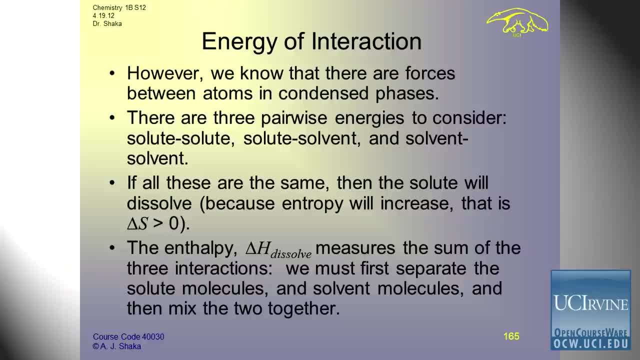 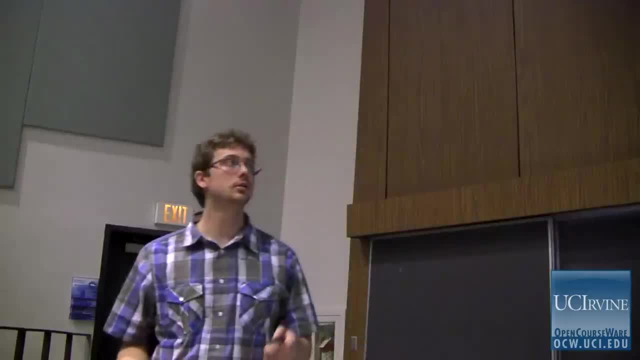 and I get that energy back. well then, it doesn't matter and it's just going to be statistics and it's going to dissolve because we're increasing that entropy. delta S is greater than zero. If this were the first time going through it. 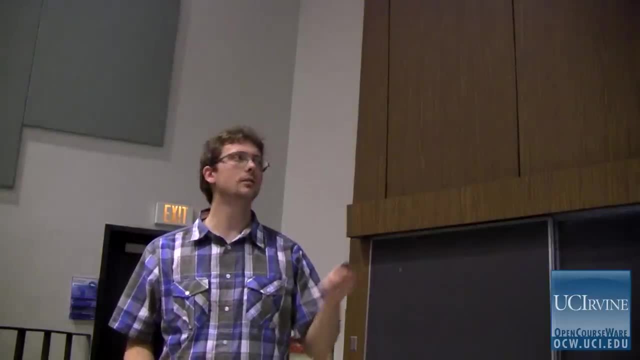 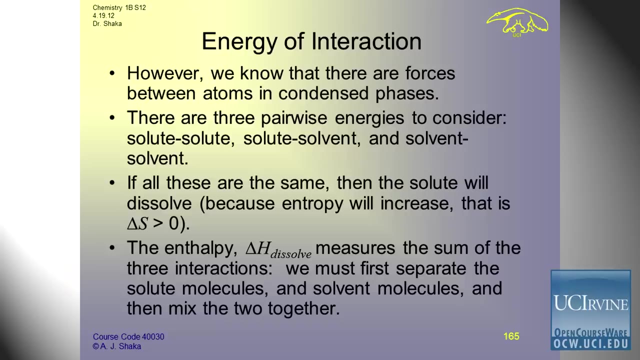 would that be a good pace? Better, Okay, alright, I'll keep that in mind. So the enthalpy delta H of dissolving measures the sum of those three interactions. We must first separate the salts from the solute molecules. 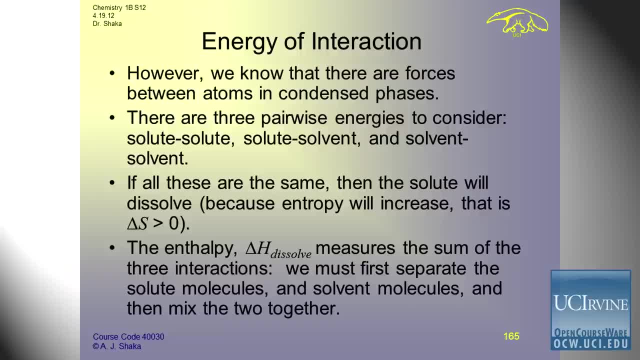 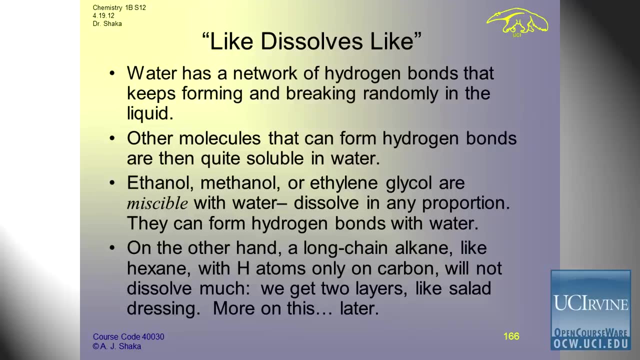 and the solvent molecules and then mix the two together. And if that is a good energy, it will happen naturally, And if it takes more energy to do that than to not do, it's not going to happen. So water has that network of hydrogen bonds. 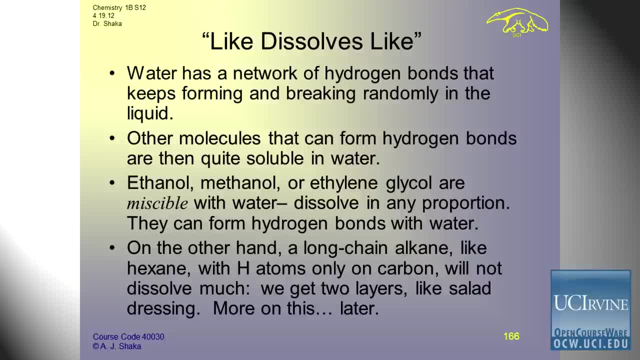 that keep forming and breaking randomly in the liquid. Other molecules can also form those hydrogen bonds and then are quite soluble in water. Let's say a moment ago: I have to break water from water and I have to break something else from something else. 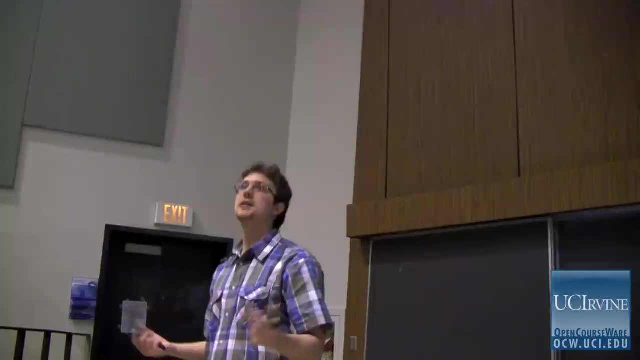 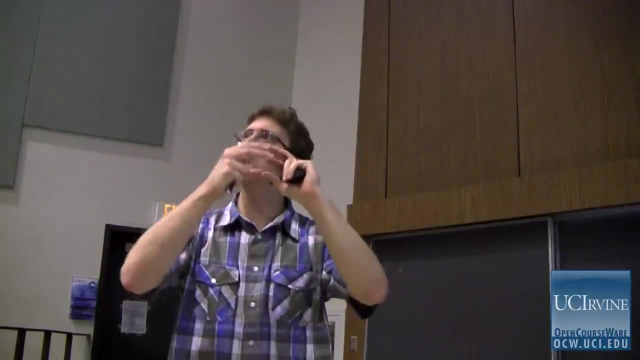 Let's say ammonia, NH3.. Well, I know NH3 has hydrogen bonds, right. So when I take that ammonia and bring it closer to water, I know they're going to form strong hydrogen bonds. This increases that interaction between water and that solute. 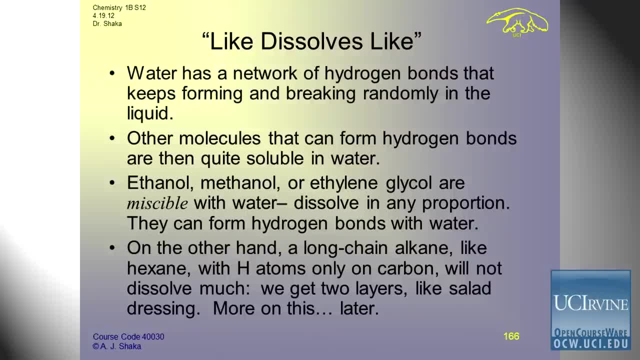 so I think it would be more likely to dissolve. In this case it would, as long as it was soluble in water. So ethanol, methanol, ethylene glycol, they're miscible with water, right? What do they have? 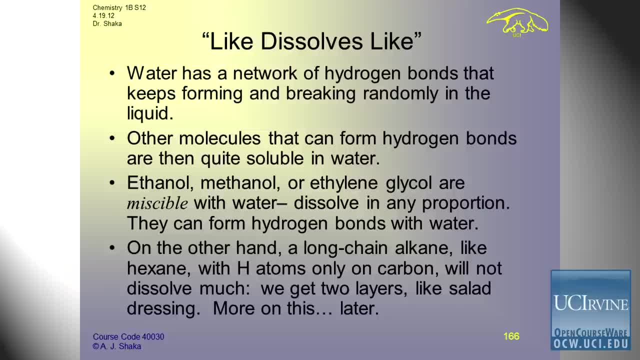 Ethanol has a hydrogen bond. Yeah, it has an aliphatic region, but it also has that OH group right, And that forms hydrogen bonds with water And so it can dissolve. Same thing with ethylene glycol and methanol. 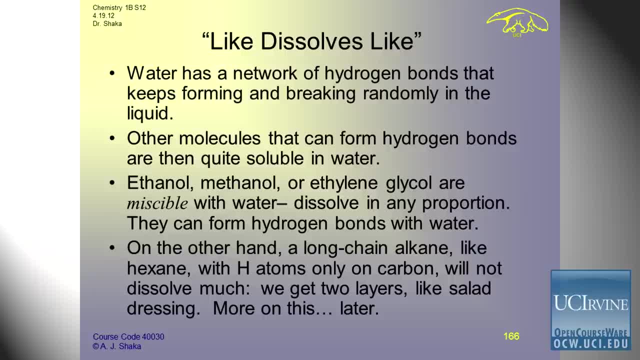 forming those hydrogen bonds. On the other hand, a long-chain alkane like hexane, with H atoms only on carbon, it's not going to dissolve very much. We get two layers right, Like salad dressing or if you're just in your lab. 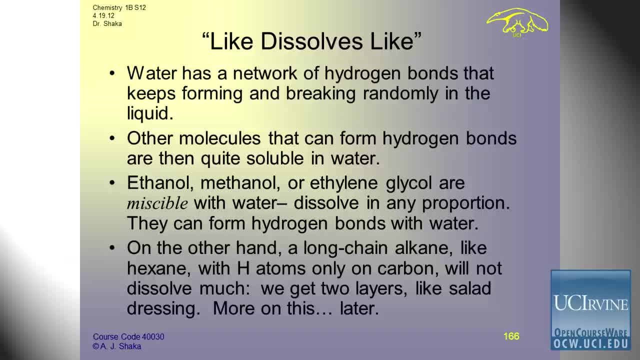 and you have oil and water, right. So let's talk about this for a second. then, If we have oil, we'll just say it's hexane. okay, Hexane and water, They don't mix. We all know that. 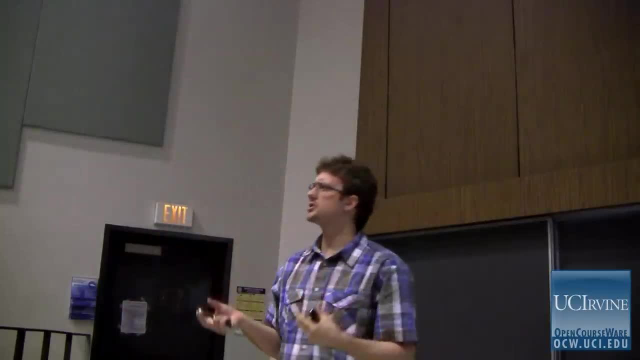 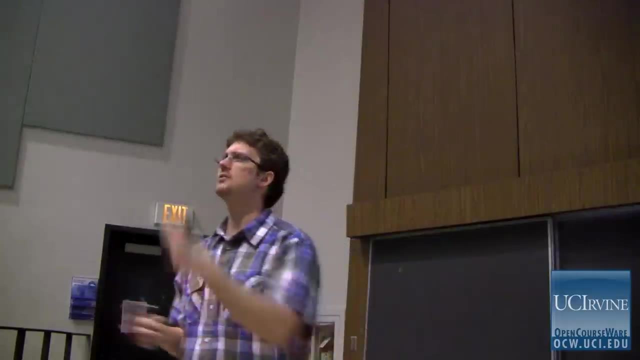 Why don't they mix Hexane? what kind of forces does it have? Intermolecular forces, I mean right, Just dispersion, mostly right. It doesn't have any H bonds, It doesn't have a dipole, It doesn't have any ionic forces. 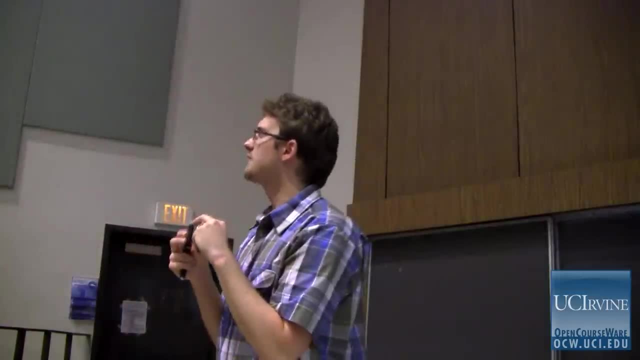 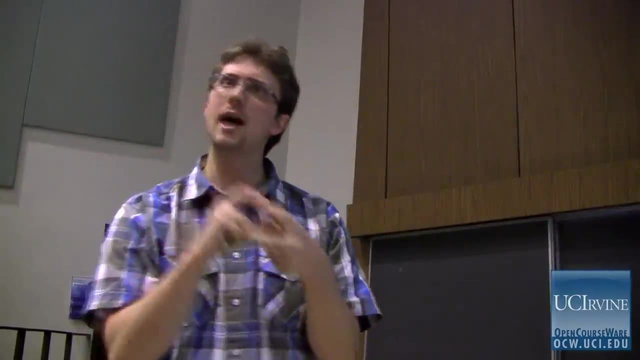 It's just dispersion. Hexane doesn't hold together very well. That's why it has such a low boiling point. Water, however, holds together very powerfully. It has strong hydrogen bonds. It has dipole-dipole forces. It holds together. 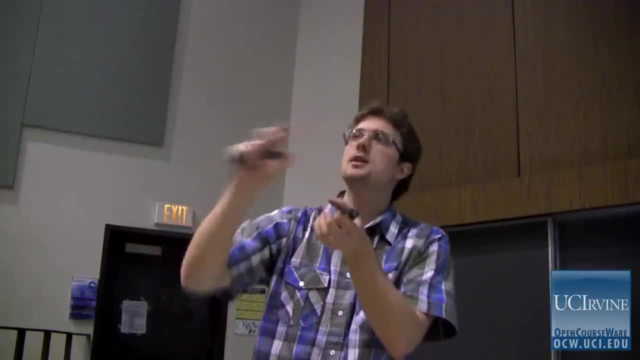 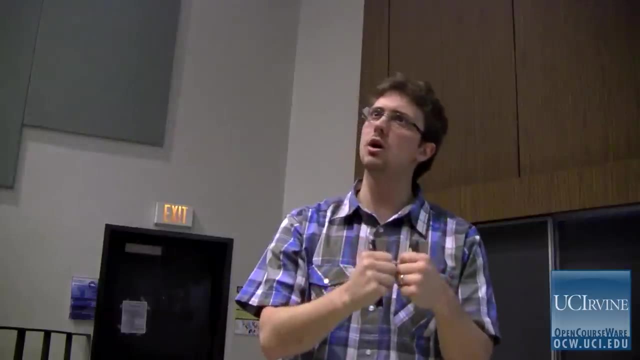 So when I try to put the two together, I have to break a hexane-hexane interaction. That's easy because its dispersion forces aren't very strong, But I have to break a strong water-water interaction. Now, if the hexane-water interaction were powerful? 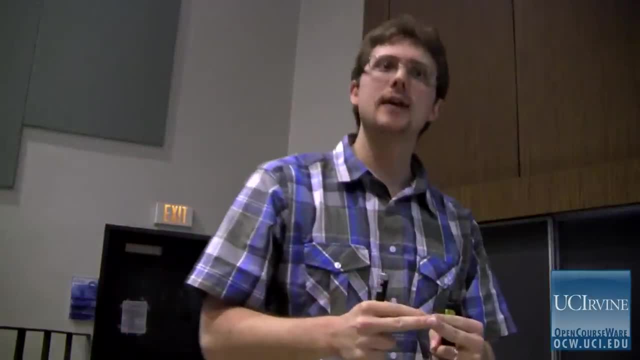 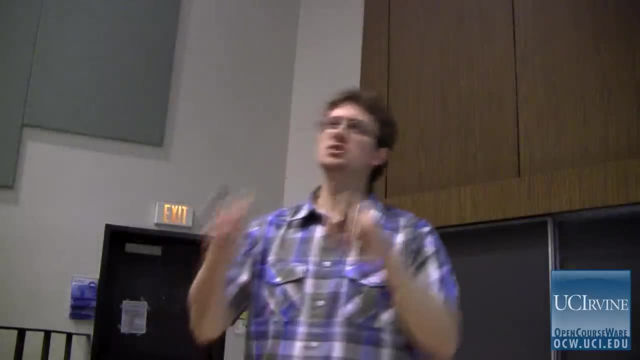 that would be okay, But it's not. Hexane doesn't have any hydrogen bonds that can get through water. It's not a dipole, so it can't interact with water's dipole very well. It's just sort of like dispersion forces. 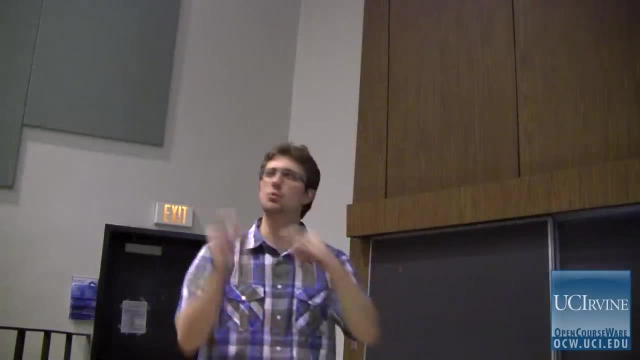 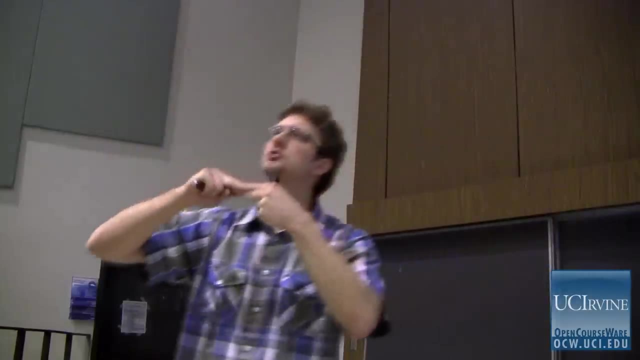 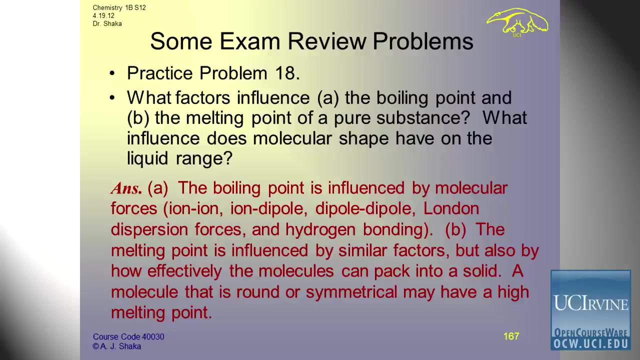 or an ion-induced dipole, that sort of thing. It's a weak interaction And so you're not going to break apart strong water with weak hexane, because their interaction is also weak, So they separate. So we're on to some practice problems. 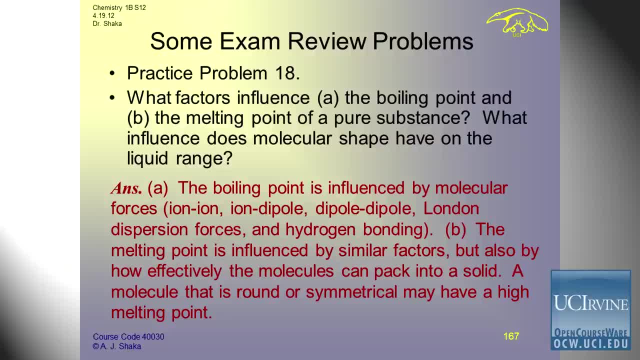 Exam time is next week. Remember what Dr Shaka said. Oh, it's not time to leave. We have some problems. I mean, you can leave if you want. I'm not keeping track, But let's see here What time. 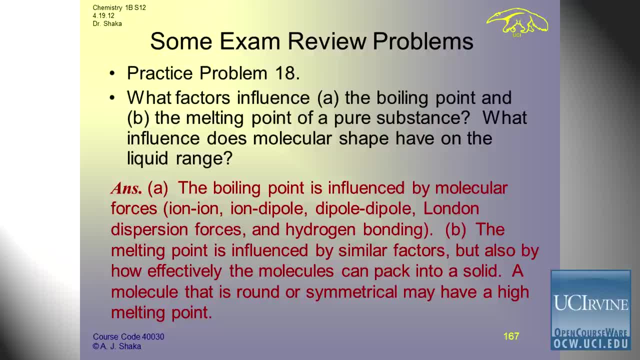 We got 1143. So we got plenty of time. There are about five questions here And the exam is Tuesday. It's going to cover chapters five and 11, plus the review one through three, But he'll probably focus on five through 11,. 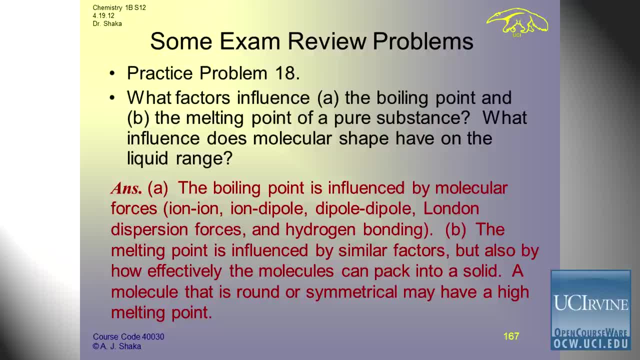 I'm sure, But just in case you need to know one through three. So we'll just go through some exam questions right now- Well, not exam questions, some review questions And we'll see how it goes. What factors influence the boiling point? 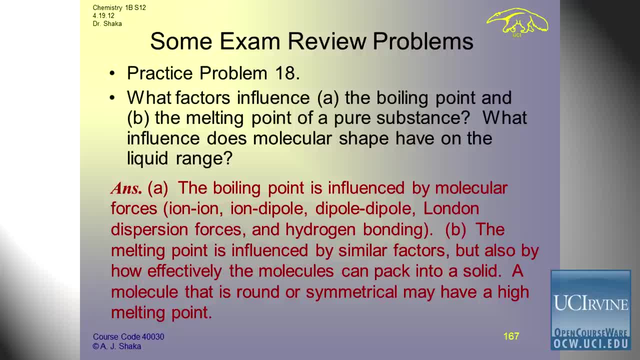 and the melting point of a pure substance. What influence does molecular shape have on the liquid range? So I think what I'll do for these problems, especially because we have plenty of time, is I'll just give maybe 30 seconds for you guys to think about a problem. 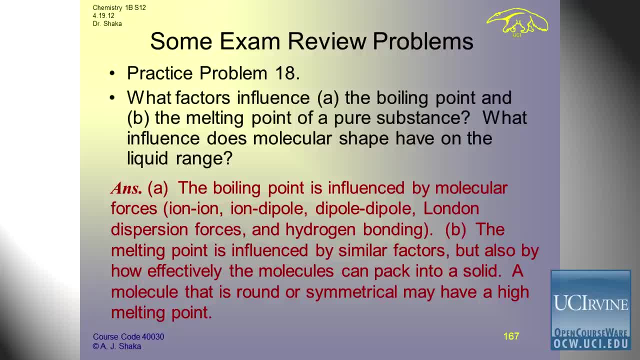 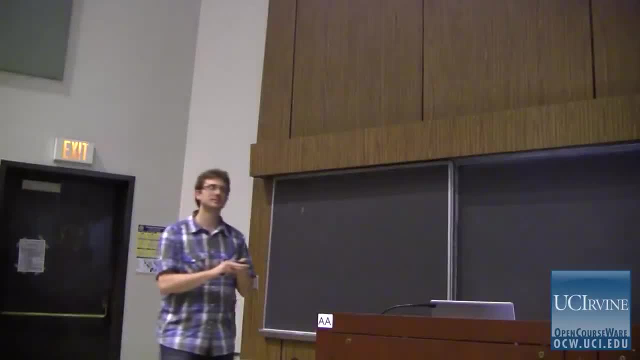 and then we'll go over it together. All right, So go ahead and just think about this for about 30 seconds. I'll try to keep quiet. It's very hard for me. I like to talk, but I'll try. It's very hard. 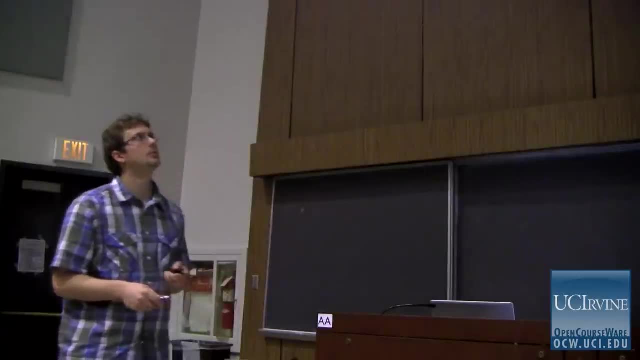 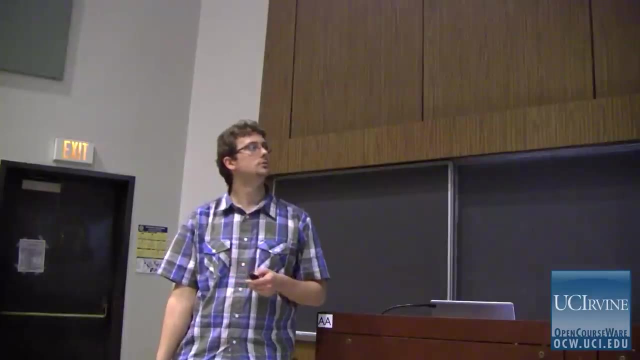 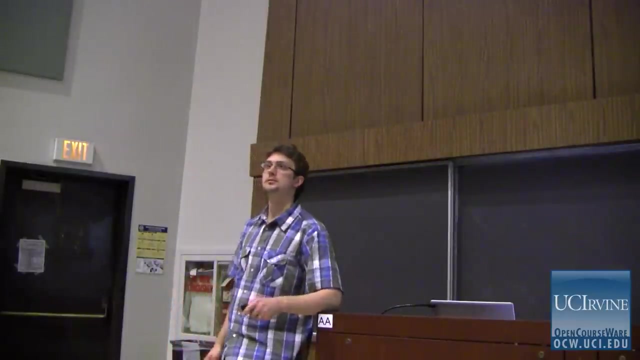 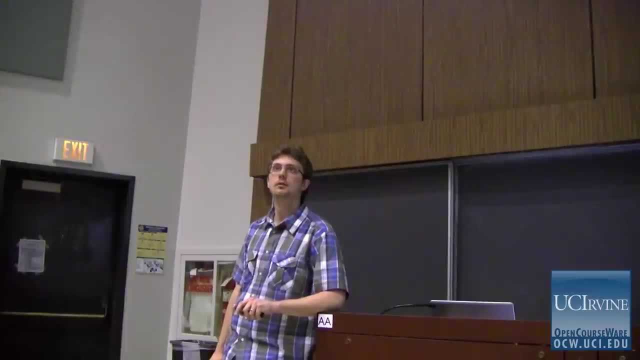 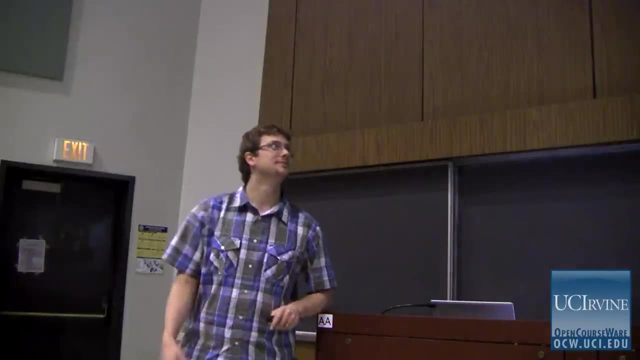 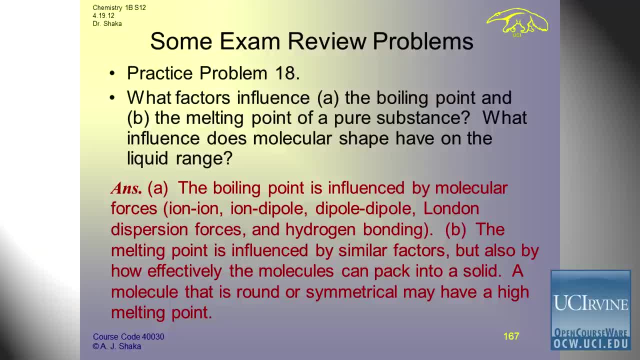 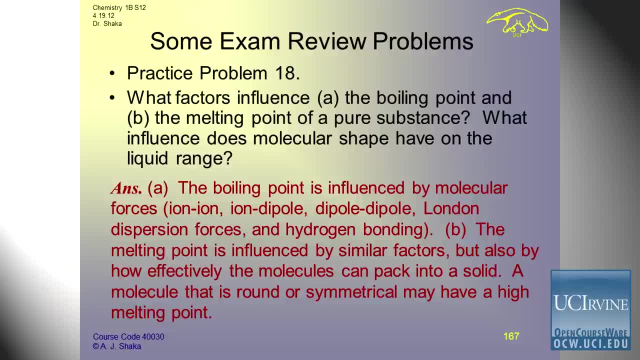 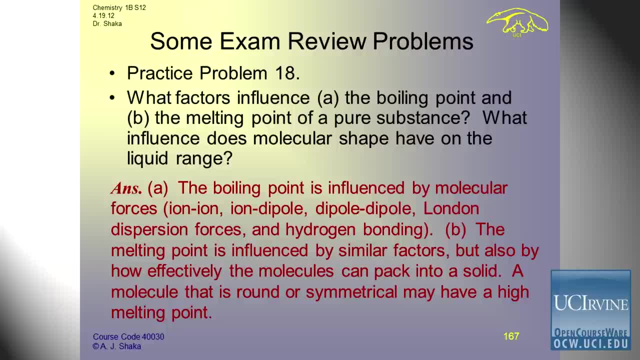 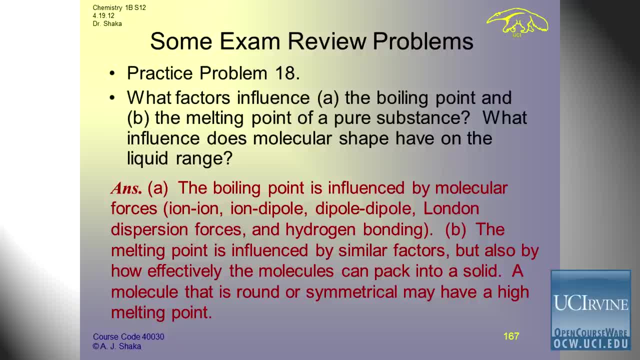 All right, All right in his lectures, But how well layers and layers of your cloud count, fit together, influence, how closely they can get together and how strong that interaction is. So we know that if I just took an ion-ion, like a positive and a minus charge, the closer I bring them together, the harder 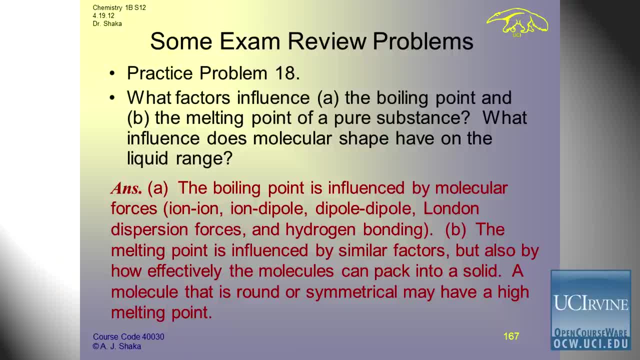 it is for me to pull them apart. Same thing with solids. If I have things that pack really well together, then when it comes time to try and break them apart to go from the melting point to the liquid phase, well, it's going to be harder to pull them apart into the liquid phase. 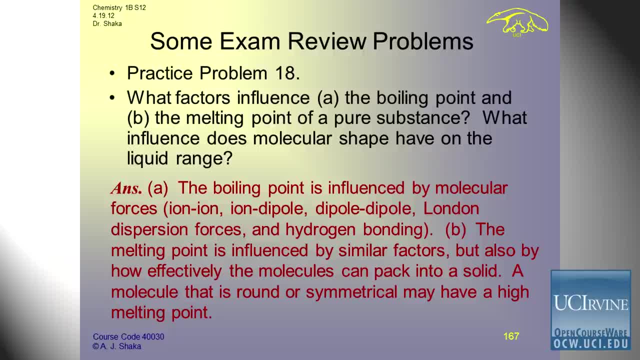 if they're packed really tightly together. If something doesn't fit at all well, it's not as able to interact as well and you can break it apart a little bit easier, and that's going to lower its melting point. So a molecule that is round or symmetrical may have a high melting point. 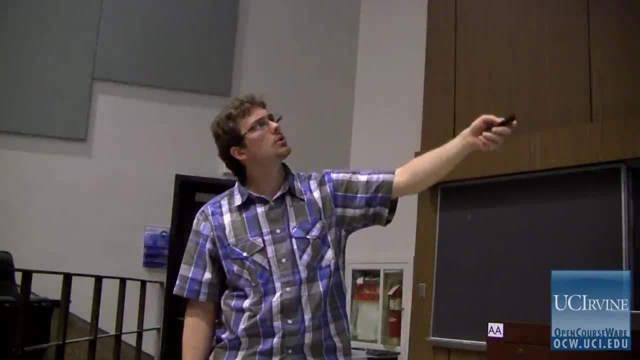 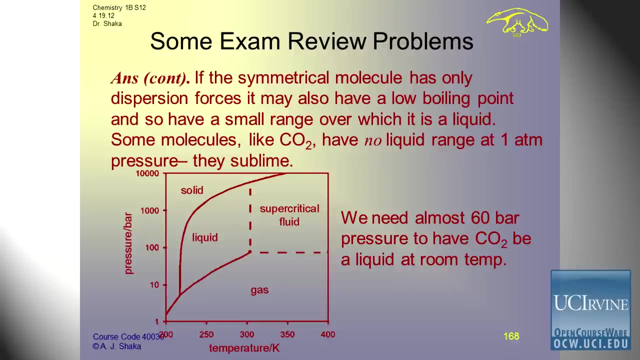 because it fits together well. So if a symmetrical molecule has only dispersion forces, it may also have a low boiling point and so have a small range over which is a liquid. Some molecules, like CO2, have no liquid range at 1 atm. 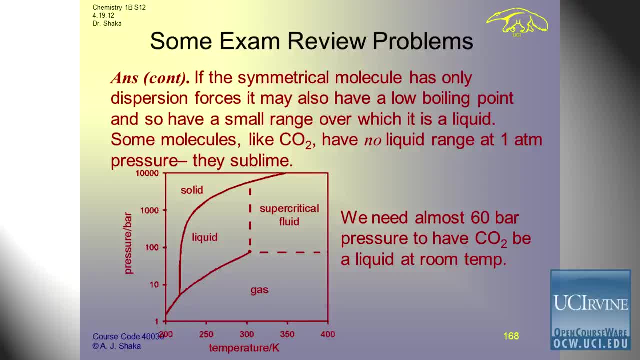 pressure. They sublime Again a phase diagram. you should be getting very familiar with these Pressure versus temperature. We know that with dry ice, with CO2, that's minus 78.5 degrees Celsius. That's at about 195, right in that range. 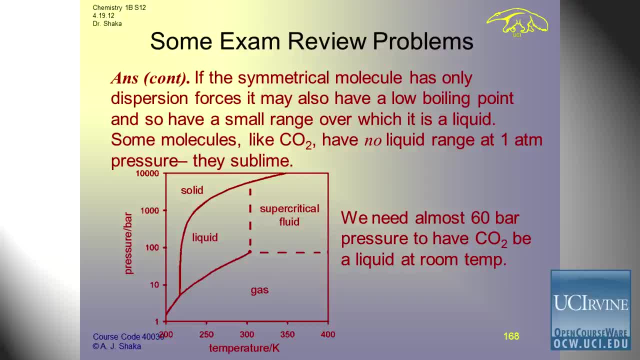 So it's unfortunate this graph doesn't show that, But here we're in the solid form: dry ice, right. So at 1 bar is around 1 atm, At a temperature of around 195 Kelvin. we're in this region, right here. 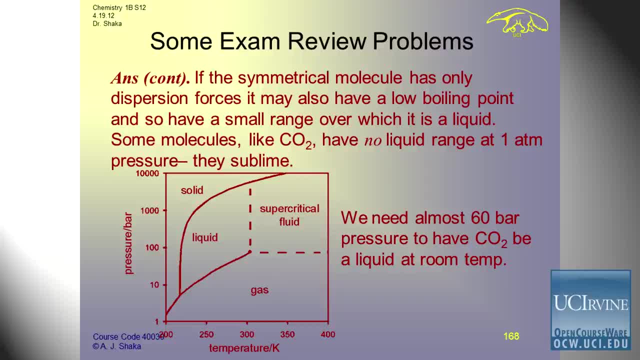 where we would be a solid. And as it warms up we enter right into the gas phase instead of the liquid phase. So we need almost 60 bar pressure to have CO2 be a liquid at room temperature. So if I increase this pressure right, let's say I'm at 100 bar. 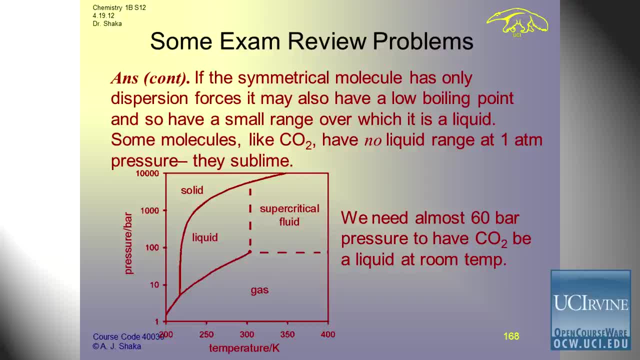 And then I increase the temperature, Then I'll enter into the liquid phase And eventually I'm in the superconductor. Yes, What was that? Can you just slide out a question from the other line? What do they mean by a? 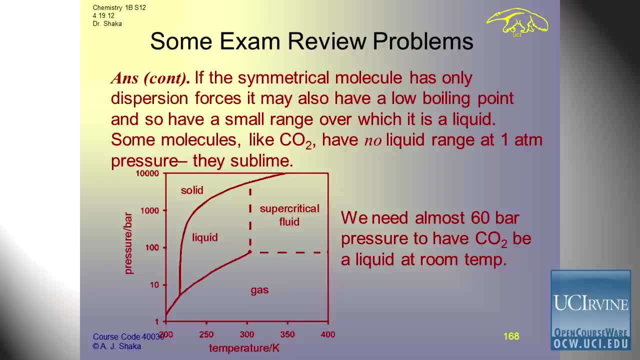 Wait, just slide it over in front. Yeah, this one. Okay, What do they mean by still having a small range over which is a liquid? So if somebody has a melting point of 0 degrees Celsius of water right and a boiling point of 100 degrees Celsius, 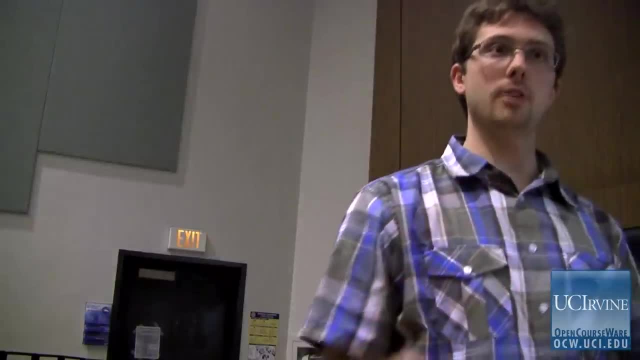 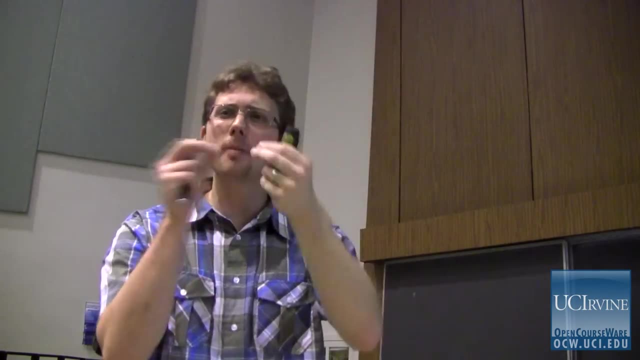 that's 100 degrees Celsius. That's 100 degrees Celsius range. okay, That's not a big range if you're liquid. They're saying that when things have very, very, very small amount of forces, sometimes it can't even stay as a liquid. very well, Once you melt it, it goes into the gas phase pretty quickly, So you would have a very small range, let's say at 10 degrees- I don't know what. well, for CO2, there's no range at all, right. It doesn't stay a liquid. But they're saying there would be a much smaller range of 10 degrees Celsius, something like that, over which it would be a liquid. I can't think of any examples that have a really small range, but except for this one maybe. 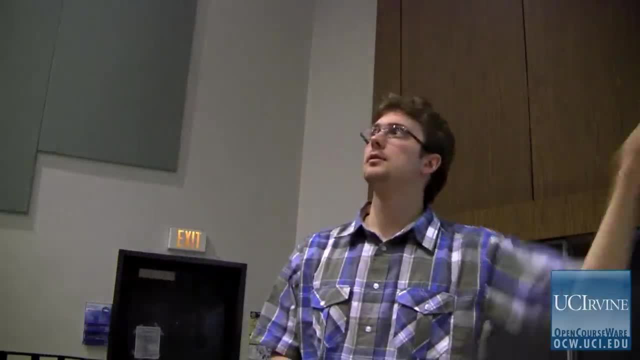 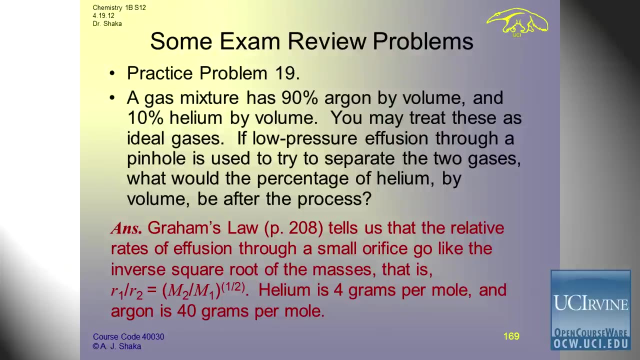 So are there any more questions on our problem? All right, I don't see any more questions. okay, So a gas mixture has 90% argon by volume and 10% helium by volume. You may treat these as ideogases. 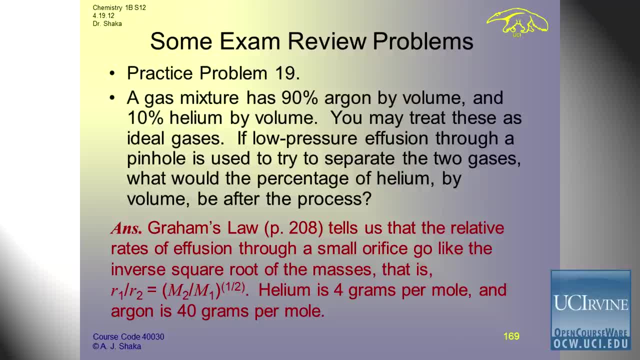 If low pressure effusion through a pinhole is used to try to separate the two gases, what would the percentage of helium by volume be after the process? Now, we're not going to sit here while people work out the whole problem. Take a minute to think about it, write out whatever you want. 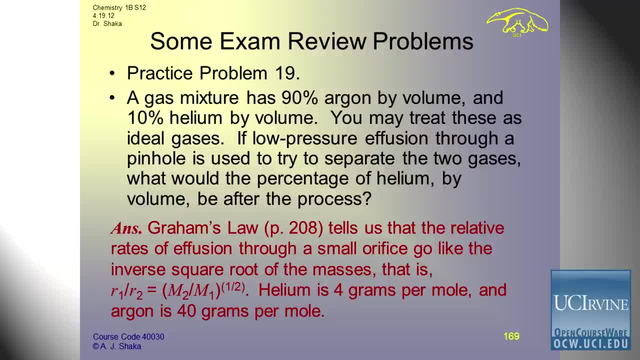 think about how you can address this problem, and then we'll go over it together. okay, Okay, Thanks, All right, we're going to do this from one end and then be off a little bit about the other end, trying to figure out basically what kind of 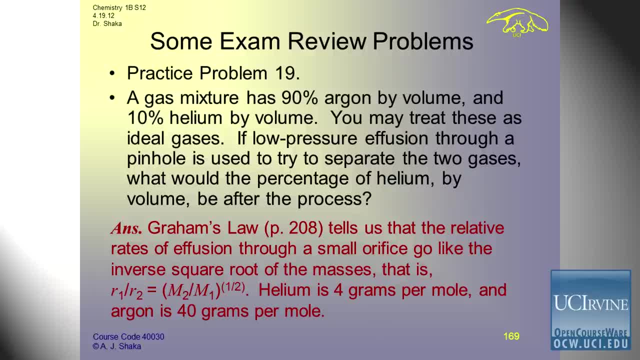 ITE background- And I'm going to take a minute to answer both umpires- and if I'm thinking about the duodenal system, the urethane rijmidon system and then the purposely pic Rings, understand qua rigidly rein fraction. Okay, 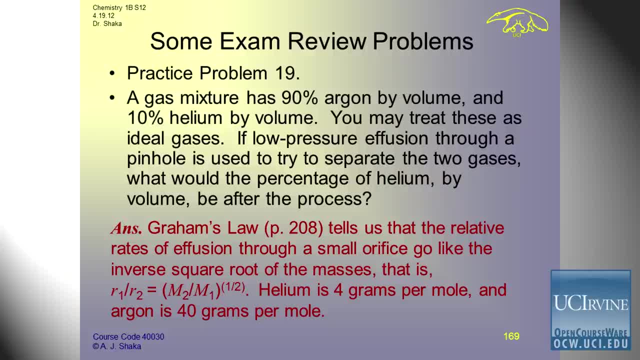 Okay, Okay, Good, All right, I'd like to stop the recording here so I can go on to this. All right, So we're using Graham's Law, page 208.. It tells us that the relative rates of effusion through a small orifice go like the inverse: 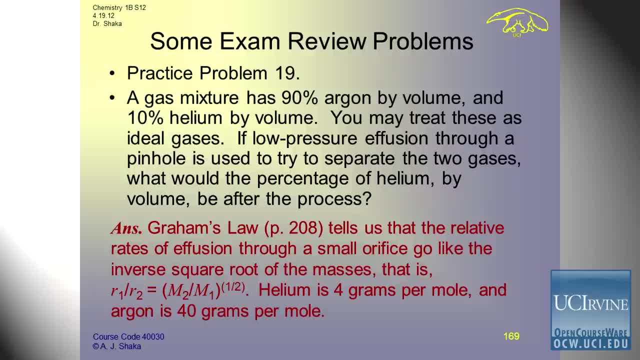 square root of the masses. so we'll look at this for one moment. that is R1 over R2.. Those are rates, not radii. The rate of the first thing going through a small hole divided by the rate of the second thing going through a small hole equals the mass of the second thing over the mass of. 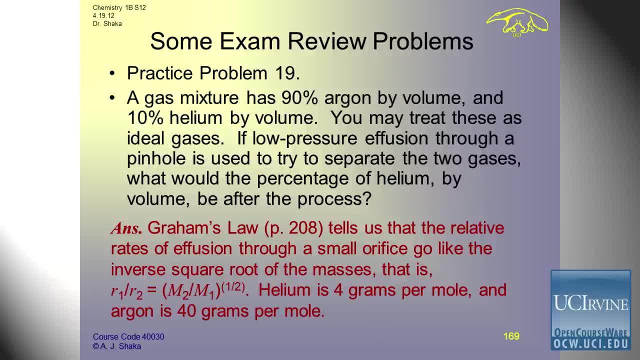 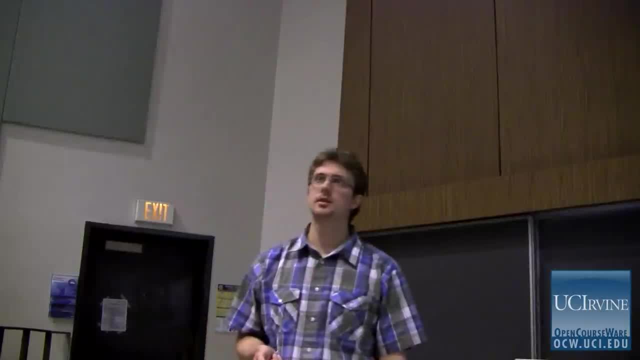 the first take the root, So let's talk about it for one second. Does this make sense? I have argon and helium. Argon is very heavy, helium not so much. I put them into a container with a small hole, right. 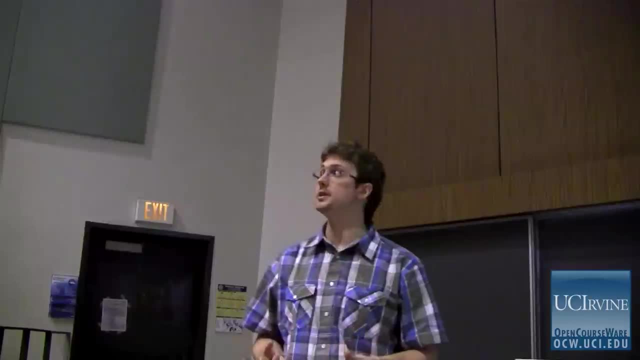 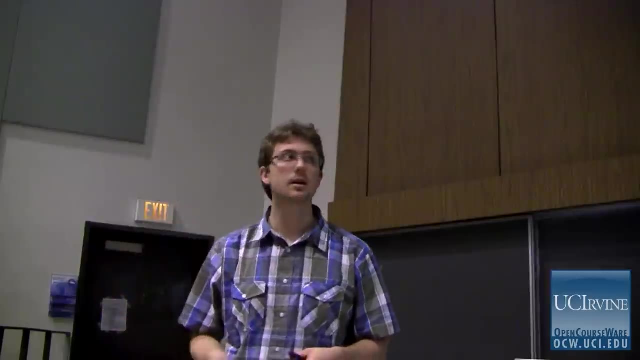 If they're at the same temperature, which they should be. which one's moving faster? Helium right, And we have our own equations that tell us that Helium's moving very quickly, It's bouncing around very, very fast. 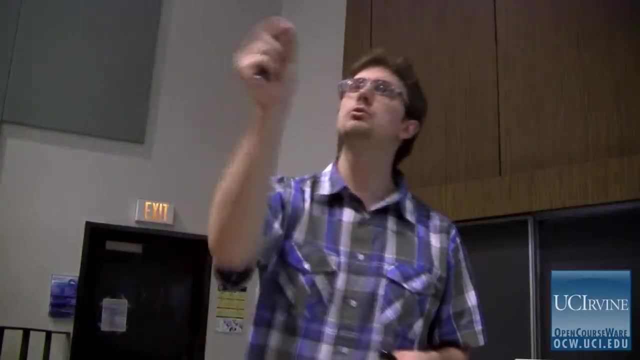 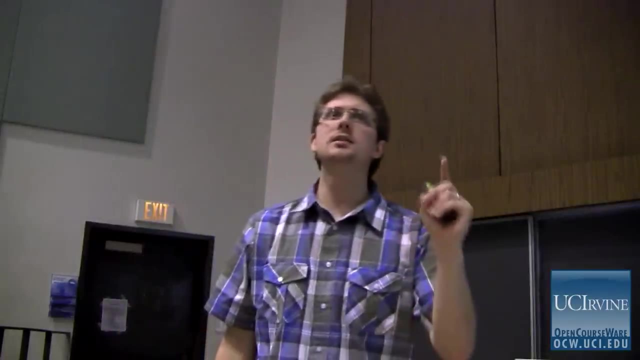 Statistically, it has a better chance of getting through that hole because it's still moving, It's moving, It's moving. It's going to hit that hole more often, right? The size of the hole doesn't have anything to do with the difference in size between. 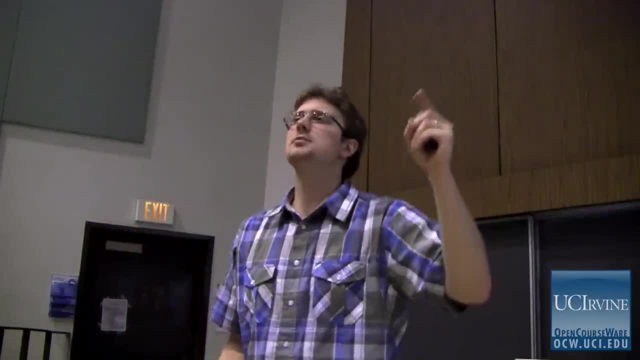 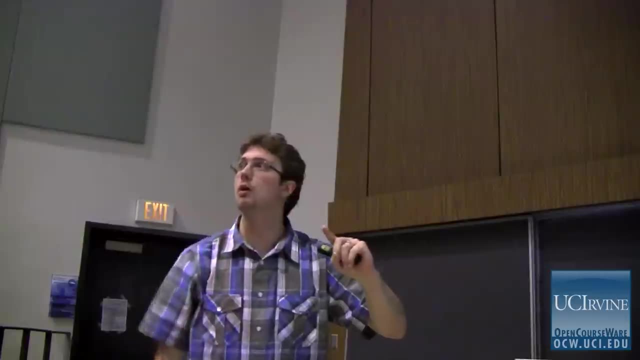 argon and helium. right Argon is still infinitesimally small compared to the size of the hole, so it's only based on the mass. Helium is bouncing around. It's going to hit that hole more often and get through. 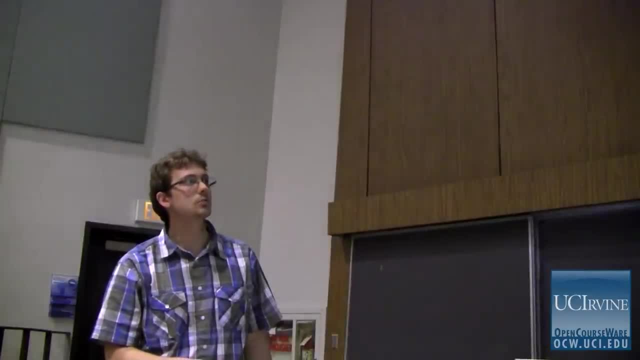 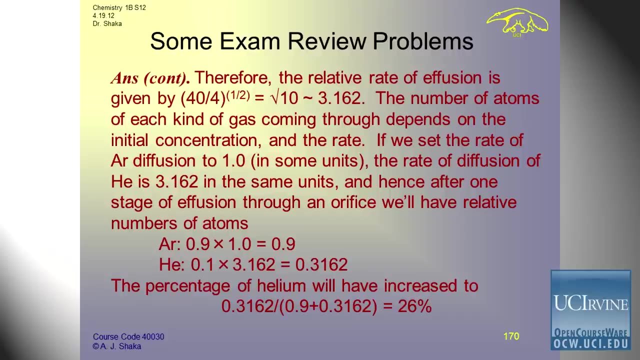 So if we take this and we plug in those masses and take the rates, we can find out the ratio of the rates. We can't solve R1 and R2.. We're taking the ratio: Helium's 4 grams per mole and argon is 40.. 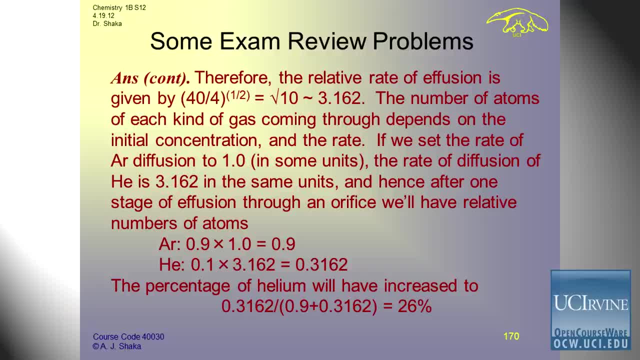 And so what this means is that the ratio, that relative rate, and remember that's R1 over R2.. The ratio is 3.162.. That's where we're saying helium will go through that hole 3.162 times as fast as whatever. 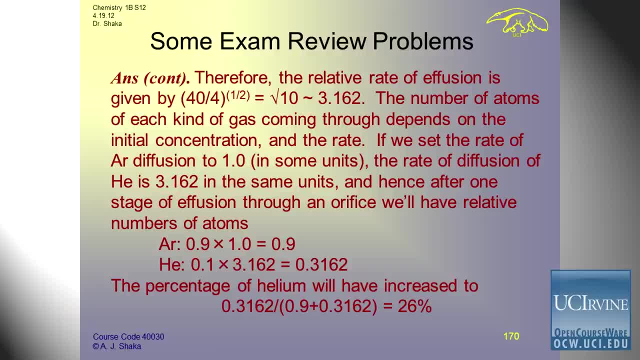 argon does. We haven't insisted, We haven't insinuated any kind of rate or a time. We're not saying how long this happens for We're saying that for one moment the rate is going to be 3.162 times the rate of argon. 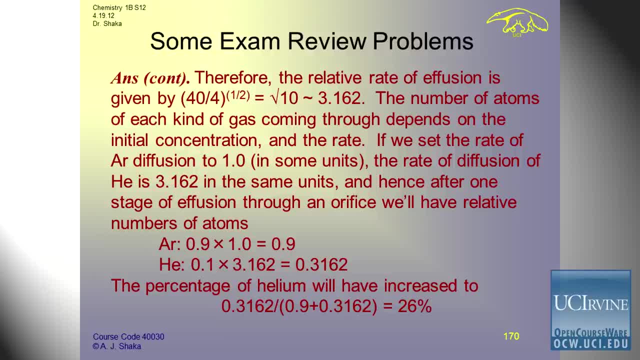 And so if we set that rate of argon diffusion to 1 in any units, we know that the rate of diffusion of helium is going to be 3.162 times, whatever that rate is, And hence after one stage of a fusion. so we could have this in seconds or hours or 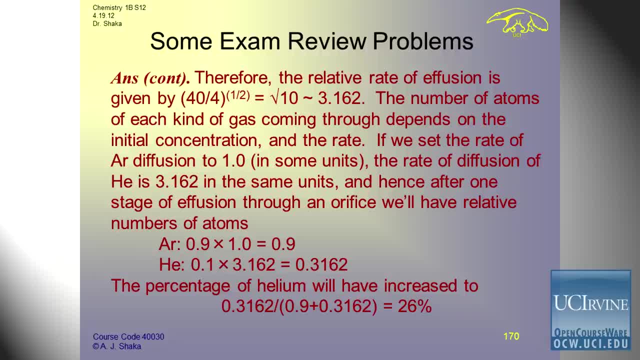 hours, whatever. it depends on how accurate you want to be. after one stage of a fusion through an orifice, we'll have relative numbers of atoms, So argon at some rate, going through. I'm going to have 0.9 of. whatever my units are. 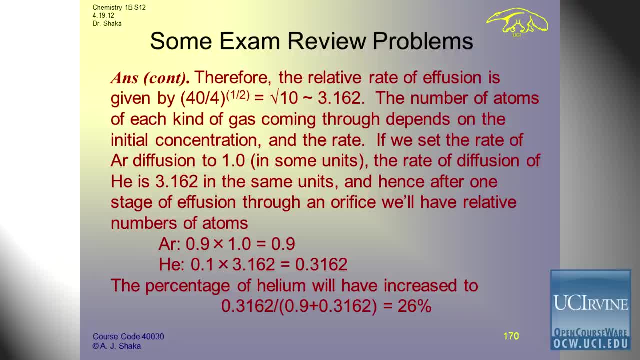 going through Helium. there's only 0.1 worth of helium versus argon. Remember it was 90% argon and 10% helium, And so the 10% of helium at three times faster a rate is going to be 3.162 times the rate. 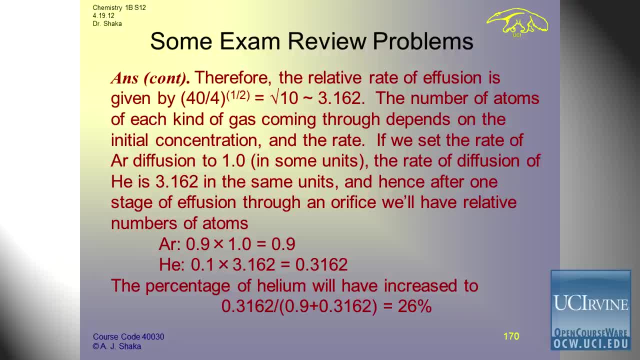 of argon. So I'm going to have 0.3162 amount of something coming through, And so what happens is total: I have the 0.9 plus the 0.3162, that's how much got through And this is how much helium there is. 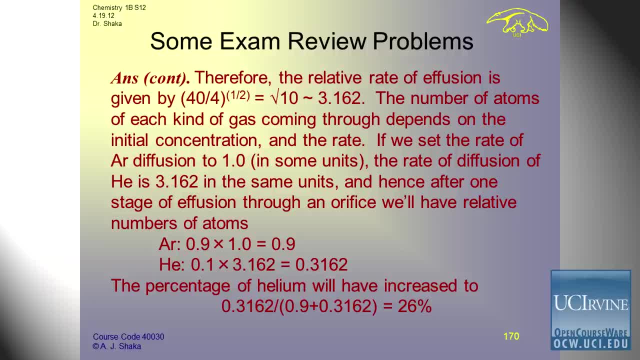 That's now 26%. So we increased from 10% helium to 26% helium. I believe that Dr Shaka used uranium as an example for this in the first lecture on ways to separate things. Again, I'm going to have 0.3162.. 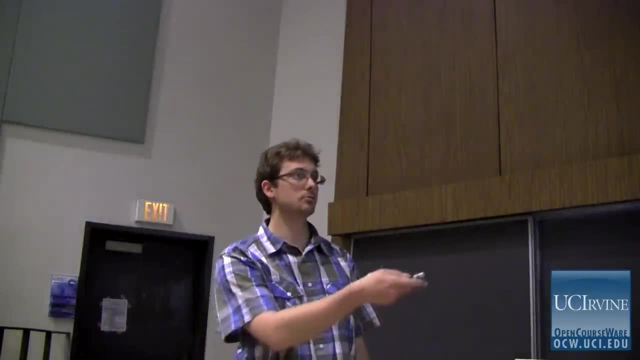 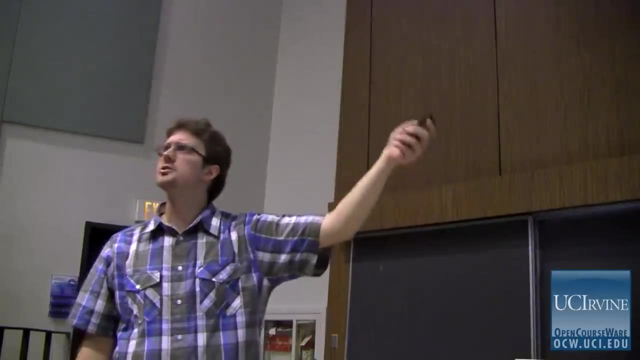 It can be quite useful, although they don't use uranium isotope separation by the method very often anymore. they use centrifuges. So, oh, any questions? I didn't realize that was the answer to that. Say again: Yeah, yeah, sure. 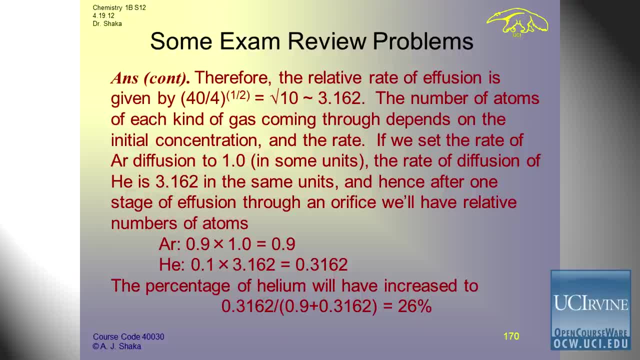 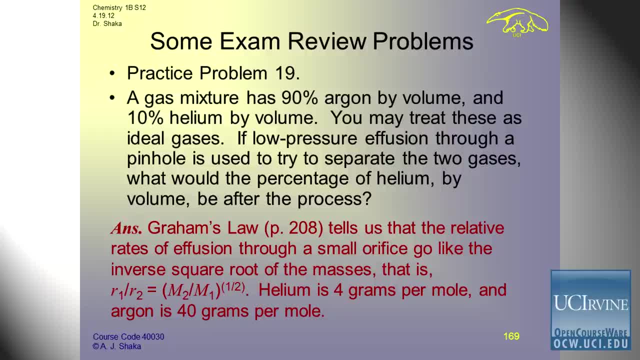 Yeah, Yeah, We let the five law sections know, We let you're right: 26% over the school and 20% helium And success rate. Yes, So it is 26%, Yes, 26% of the generation. 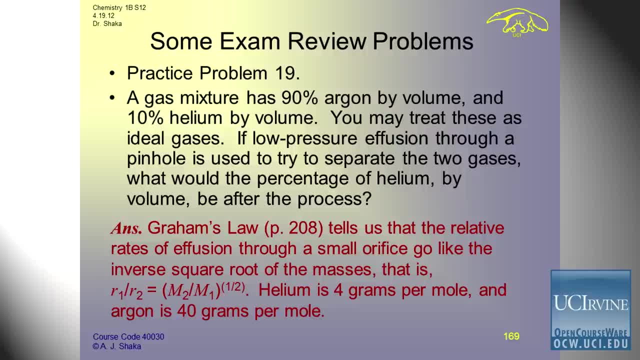 Yes, Yes, Yes, 26% of the. So we have one chamber and then another In that second chamber. What? Why is it important? That means that in the first container I now have even less helium by percentage than I did before. 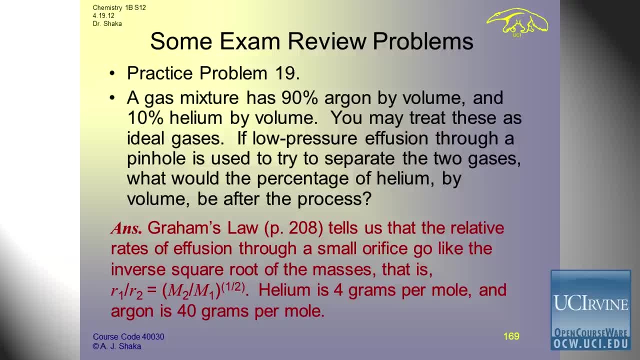 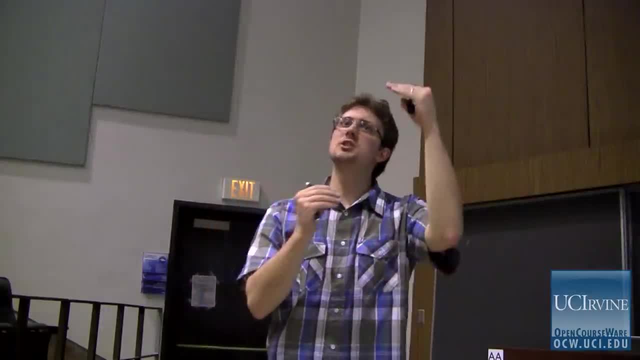 I had 10% before. Now, whatever the amount is, it's going to be less than 10%. So if I keep letting that going, the differencing rate, which was 3.162, that's going to start decreasing. 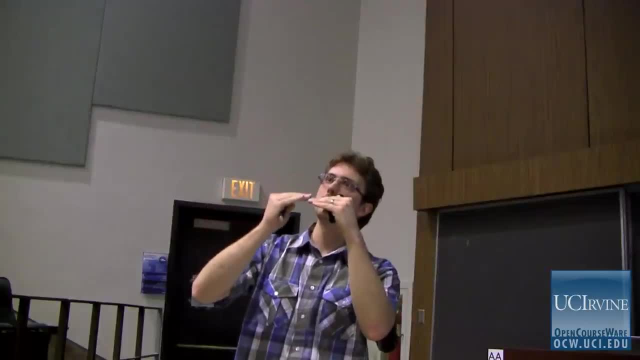 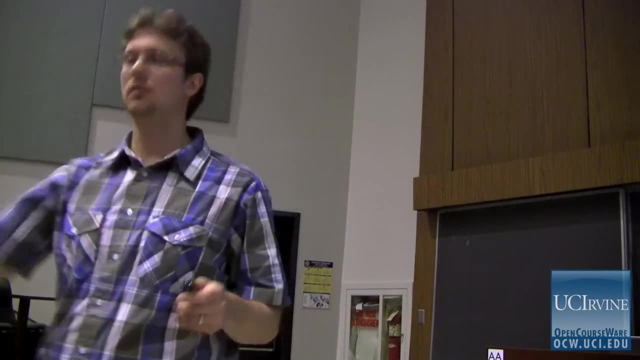 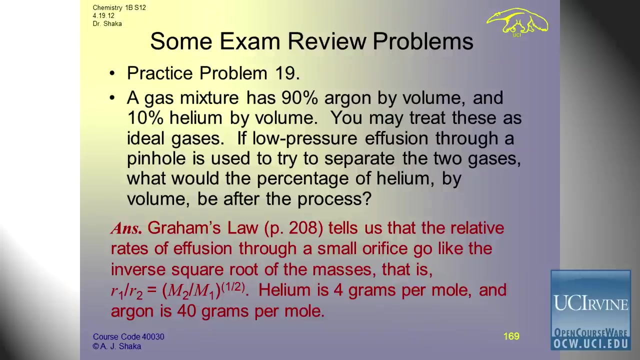 Because as I get closer and closer to there being almost no helium, there's going to be more argon going through than helium. Your question asks: what would the volume of the original container be after the process? Gas, two gas bins. What would the percentage of helium by volume be after the process? 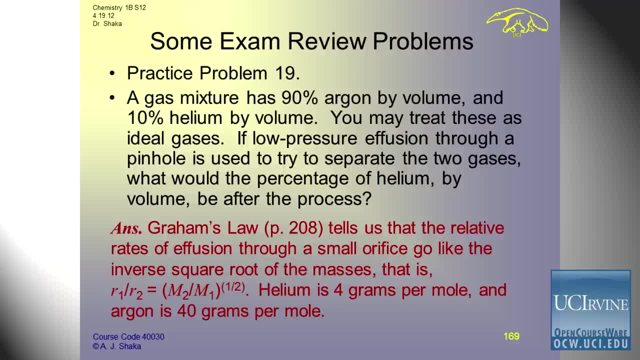 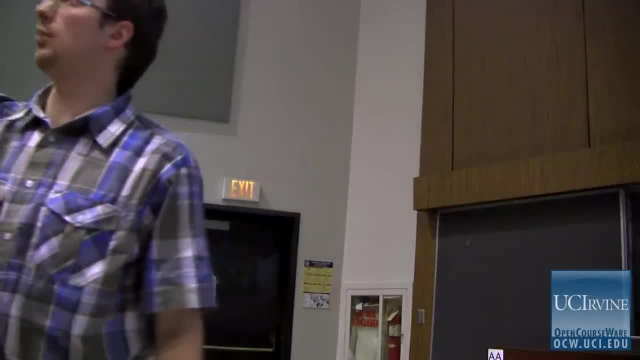 What were you looking at? Because are you the last line? Yeah, Oh, it was saying the percentage of volume is going to be 26%. That's the new container. That's the new container. Whatever went through is now 26% helium. 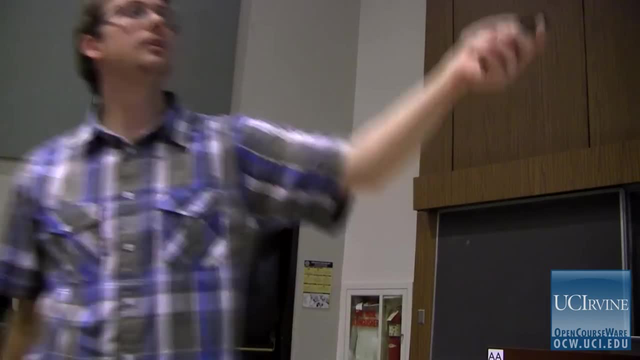 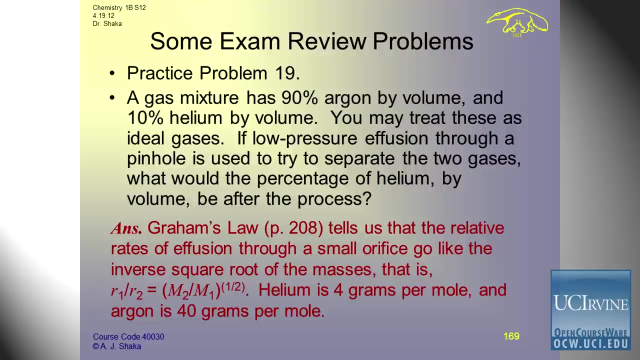 Okay, On the previous slide you had a equation Over R. this is R1 over R2, and then M2 over M1.. Yes, So this makes sense, right? Let's say 1 is helium. Okay, So the rate for helium is going to increase faster and faster relative to argon. 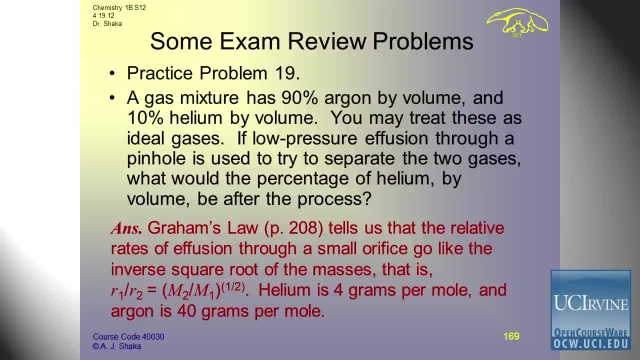 As the mass of argon or whatever. my second one is: it's heavier and heavier versus helium, So let's pretend it's not argon for a second. When this is argon, we have 3.162.. That's 3.164, right. 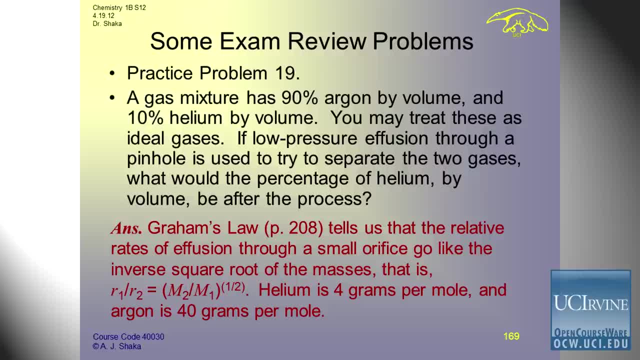 So M2, 40, over M1, 4, take the root 3.164.. If I made M lead right, something really heavy, let's just say something 200 grams per mole. okay, That now is 200 over 1, and take the root. 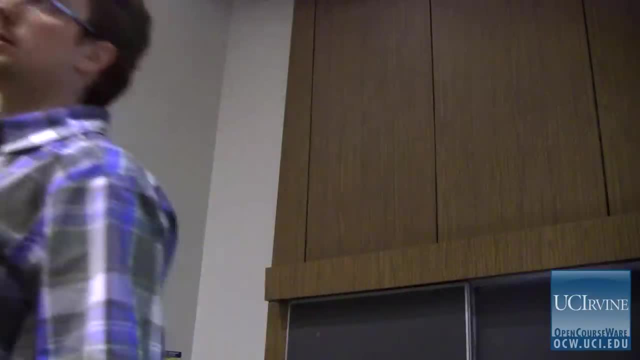 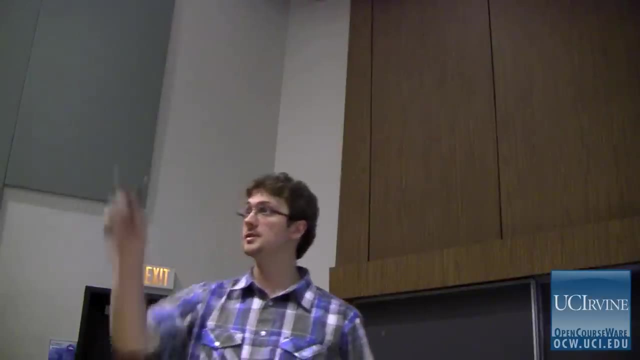 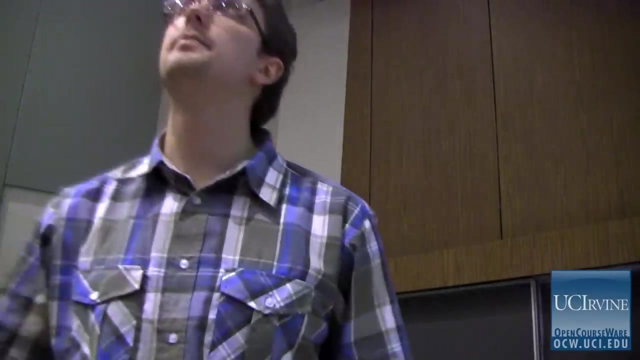 That's going to mean R1 over 2 is now Yes, Because helium is so much faster than whatever that really heavy gas is that I'm putting in there. Does that make sense? Okay, Is there any time to? I can hear the whole thing. 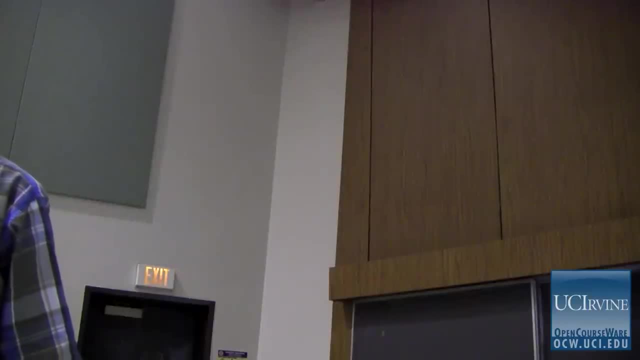 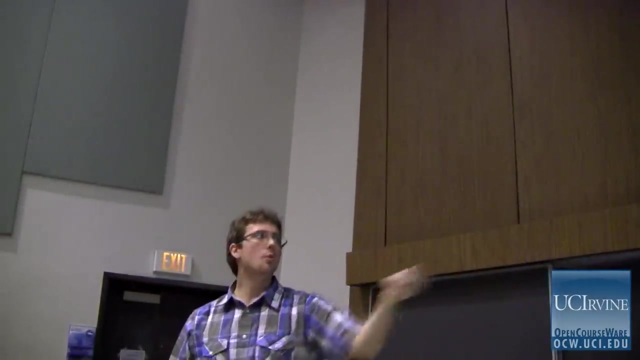 Can you explain why? Oh, it's just. it just makes the math easier. If we had a real situation, we would want to know exactly how much argon we had. This is a demonstration of using ratios to compare relative rates. We just said that, you know. 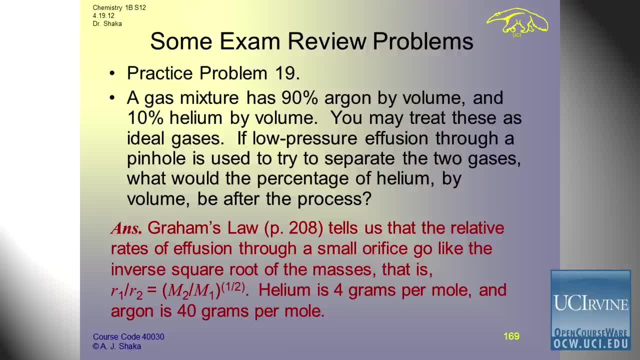 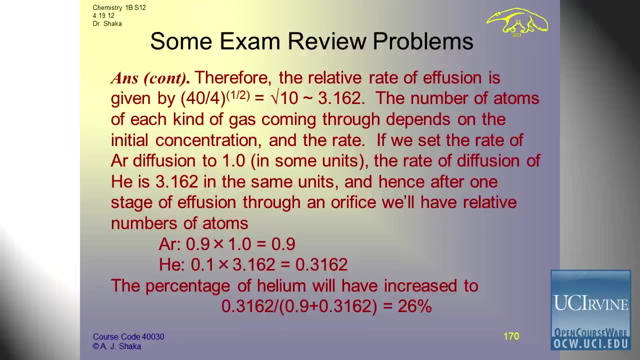 We say that R1 over R2 is there, you are 3.162,. okay, So I'm pretending that whatever the rate of R1 is, I just call that 1, and I'm saying relative to that. so R2 is 1, if the ratio R1 over R2 is 3.162, that lets me say: 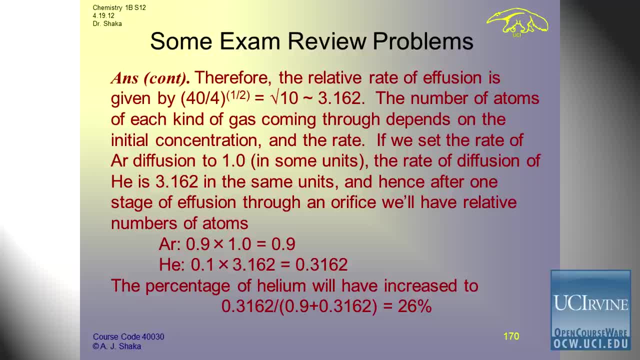 that the rate of helium transfer is 3.162 times whatever R1 is. Okay, I think I'll have to limit that one. Well, we've got plenty of time right. I wish there was a clock as long as this guy. 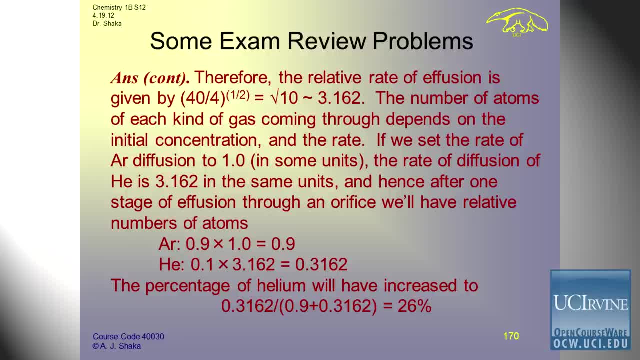 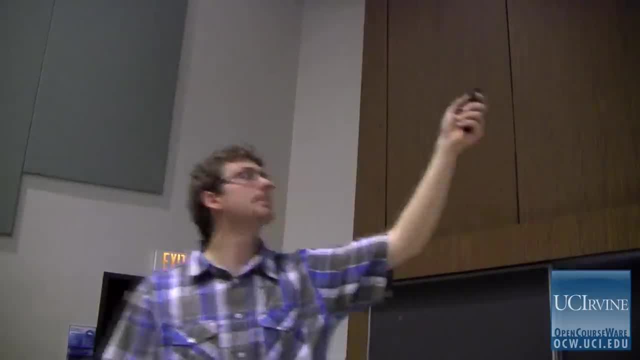 11.58,. class gets out at 12.20,. we've got a few more questions. If you have more questions on it, come down and ask me afterwards, okay, So we'll move on. Did anyone want just a moment to write something down now, real quick. 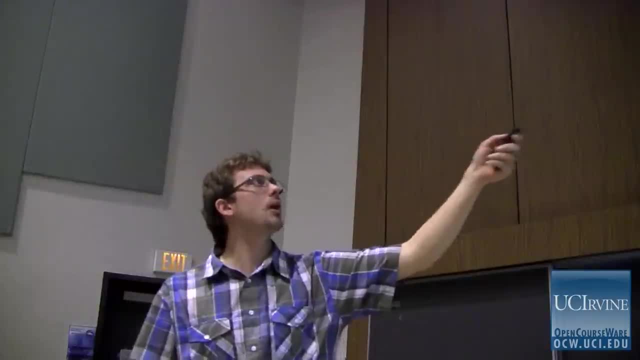 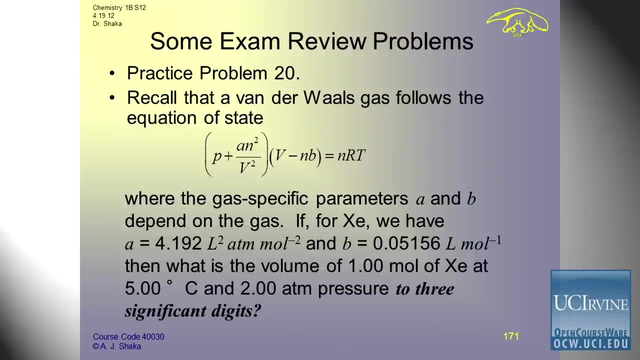 You got it, Okay, All right. so another practice problem- Okay, All right. recall that a Van der Waals gas follows the equation of state as follows. I'm not going to read through that. Remember that the ideal gas equation is just: PV equals NRT. 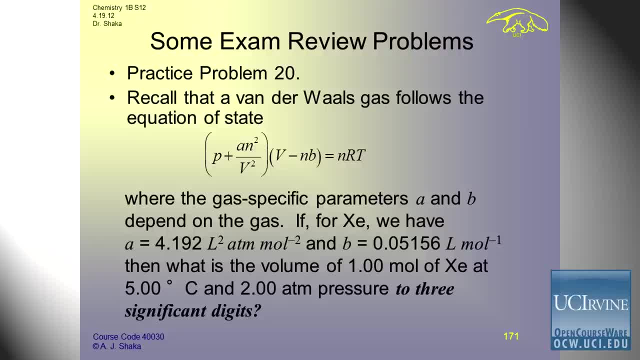 and here we've said: well, PV equals NRT is great, you know, but it's not fantastic. So we've added in these correction factors AN squared over V squared and minus NV, So where the gas specific parameters A and V depend. 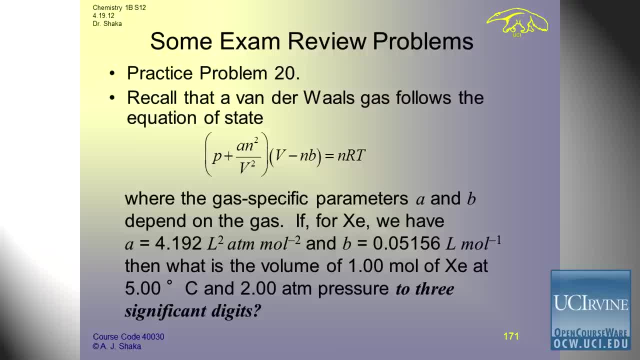 on a gas. if For Xenon we have A equals 4.192 liters squared ATM per mole and B equals .05156 liters per mole, Then what is the volume of one mole of Xenon at 5 degrees Celsius and 2 ATM pressure to 3 significant digits? 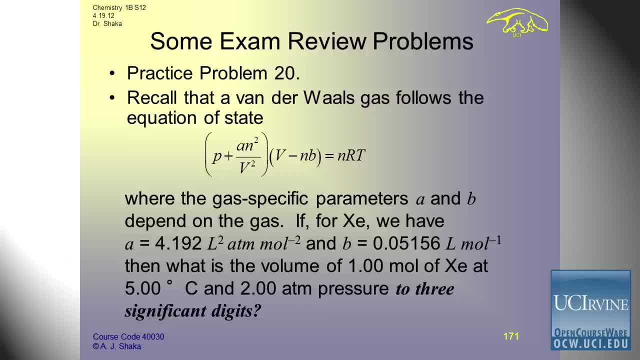 Now I'd like to take a moment here to point out something about units. So what if you were just looking at this? you'd think: what are the units of A? I know what the units of N are. right, N squared, it's moles. so that's going to be mole squared. 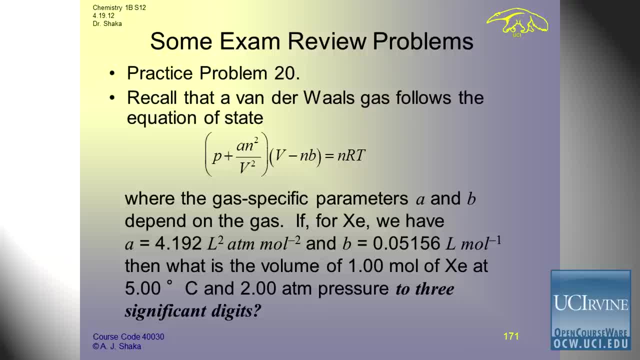 and the V, that's liters, that's liter squared. For me to add two things together, they have to be the same units, right? And so automatically I know the units of A, Because for AN squared over V squared to equal ATM, A has to be liter squared. 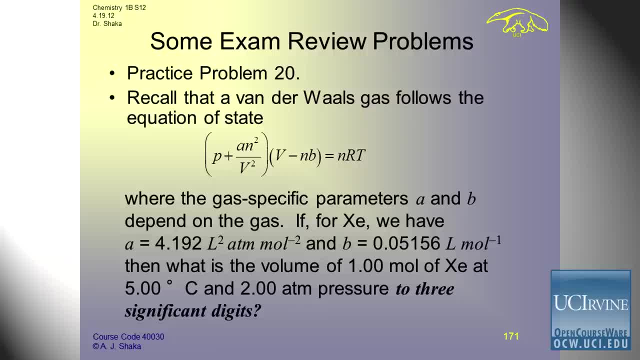 to cancel this out: ATM. so you have ATM per mole squared to cancel out the mole squared there. That's just a quick way to address that. Where are the units in this situation? Similar to NB, for volume equals liters. NB also will have to be liters. 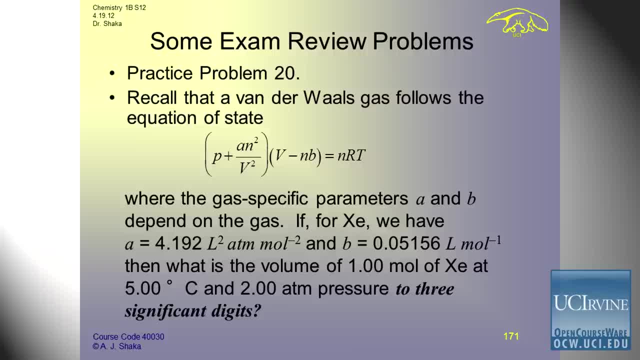 And so B is going to be liters per mole, because N is mole. So mole times liters per mole gives you liters, Excuse me. So go ahead and take a moment to try and find the. where was it And what is the volume? 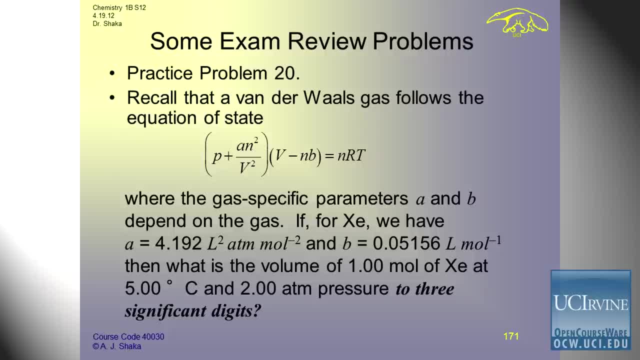 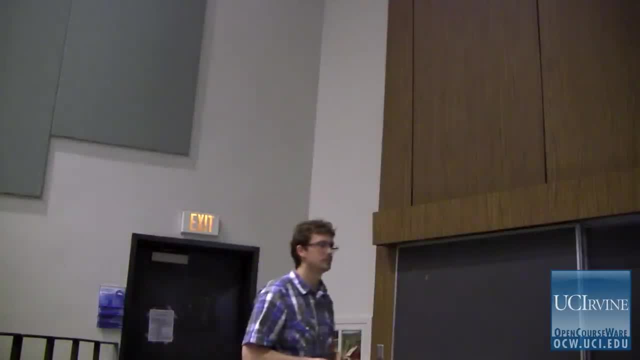 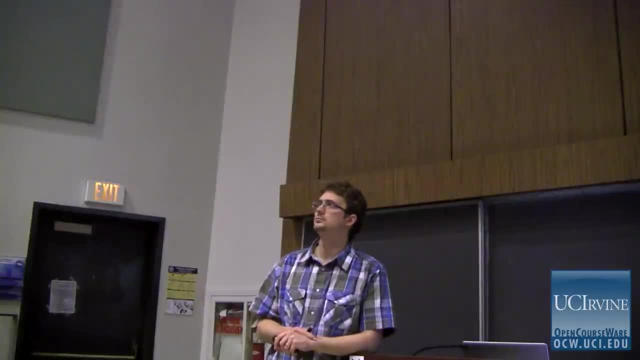 Try and find the volume of one mole of Xenon at 5 degrees Celsius and 2 ATM pressure, The three significant digits. Okay, Tip, Don't try and solve for V in that equation. You're going to make a quick guess. 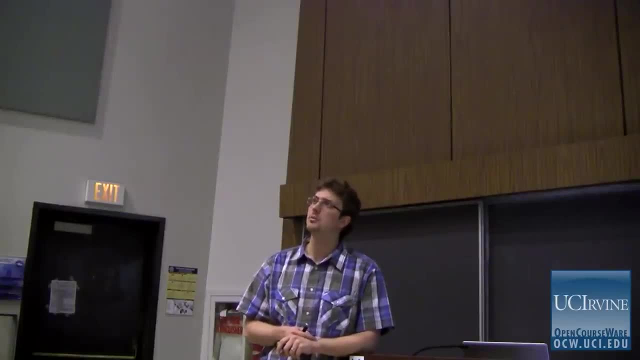 And again, the only way to solve for V is to use the equation that you have. That's not quite as accurate as that one, But it will let you almost get the answer. So, Dr Shaka, earlier in the quarter. 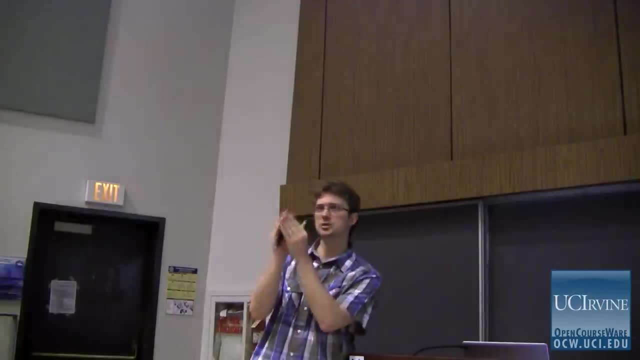 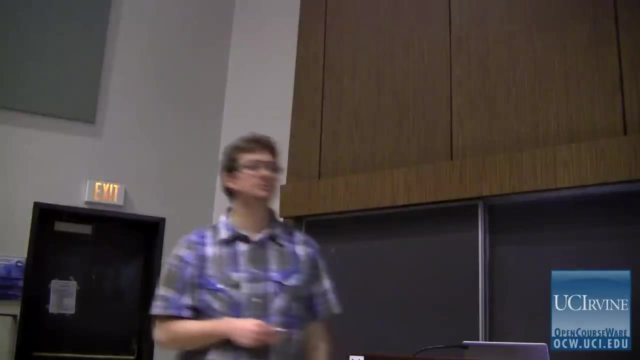 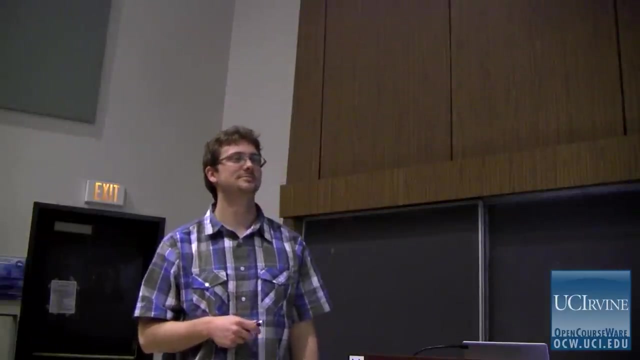 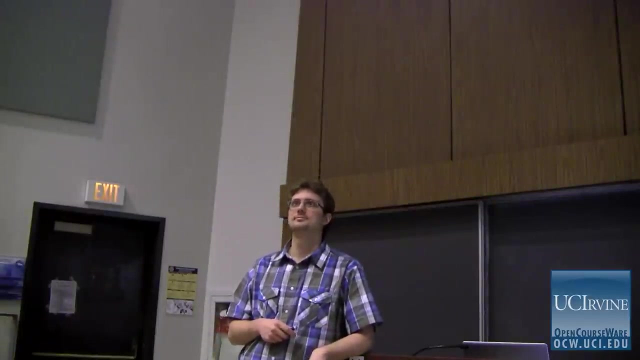 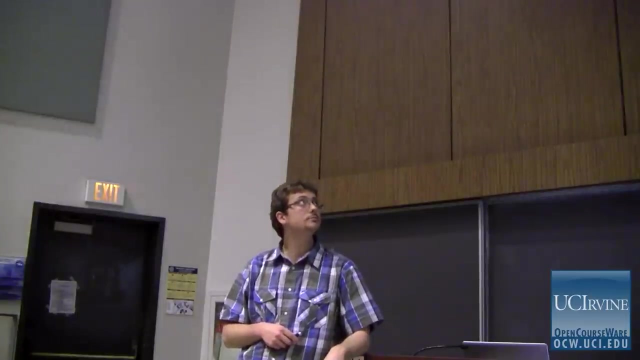 remember he has the get really close and then punch in the calculator a couple guesses until you're spot on Right. So don't try and solve for V. Thank you, All right, so let's go ahead and flip on over. So first thing, as Dr Shaka is fond of telling you, 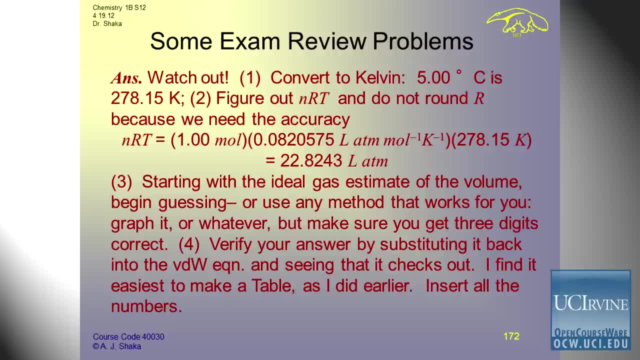 remember to convert Celsius to Kelvin. Keep everything in the same units. His advice is to use PV equals NRT to first guess almost the right answer, and then you're going to nudge your way. So figure out NRT and do not round R, because we need the accuracy. 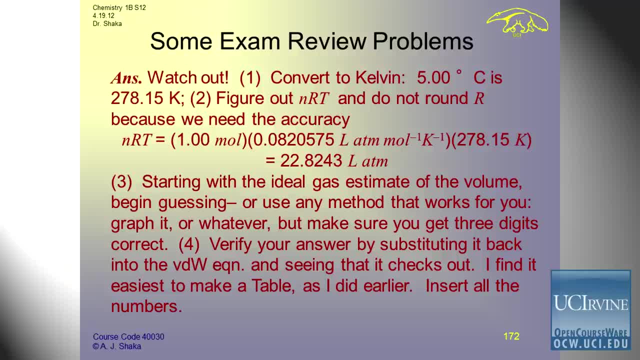 So something he keeps on harping on in the class is don't round too much, right? If he asks the accuracy, don't think at the end just oh, you know three digits, Just make sure at the end I have three digits. 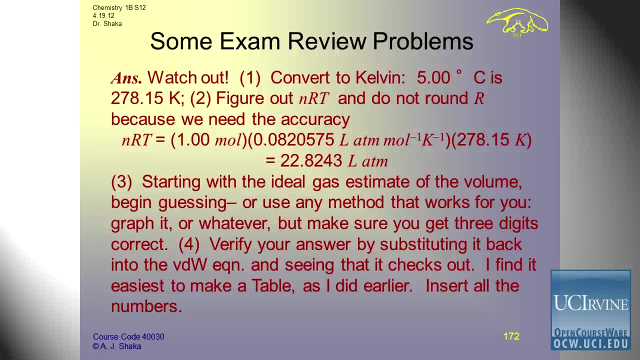 If you cut out certain digits earlier in the problem it's going to ruin your accuracy down in the end. So you have to keep that many digits all the time. So in this case we're using as many digits of R as is practical. 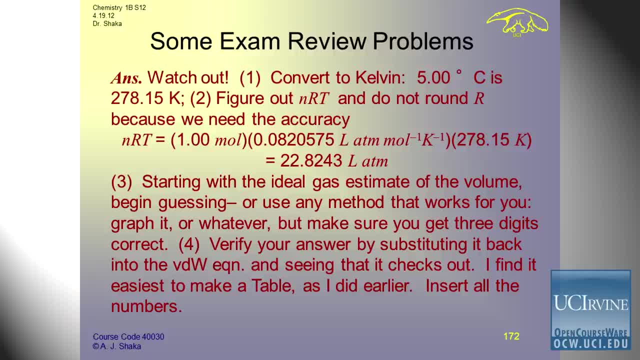 Going out to four is plenty. good, That's going to give us all the accuracy we need, and more to get our three digits in the end. So figure out NRT, don't round R, and that equals 22.8243 liter ATM. 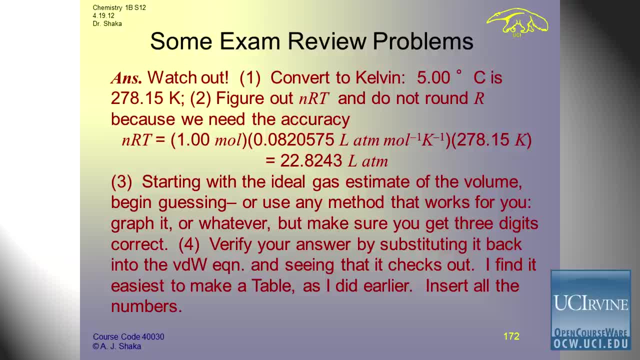 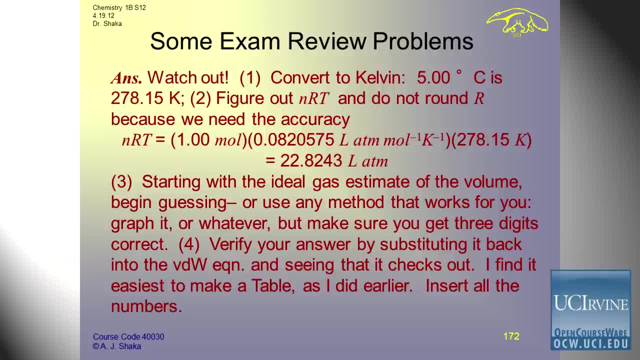 So we started with the ideal gas estimate of the volume when we begin guessing. So, or use any method that works for you, You can graph it or whatever, but make sure you get the three digits correct. to verify your answer by substituting it back into the equation. 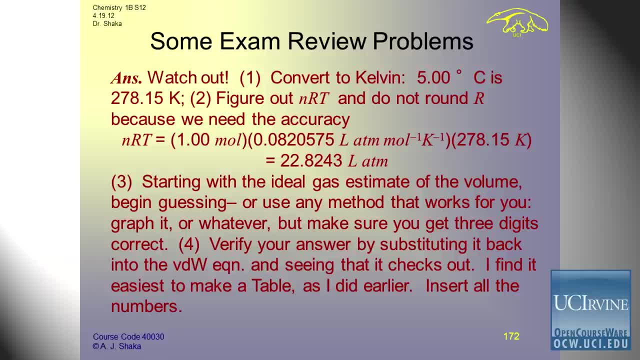 Okay, All right. So he's saying: well, we know NRT. If we go back to the, to the full equation, NRT doesn't have A and B in it. We're not making any assumption by just solving for NRT. 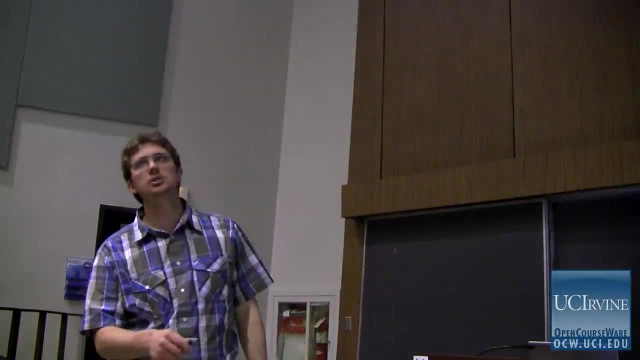 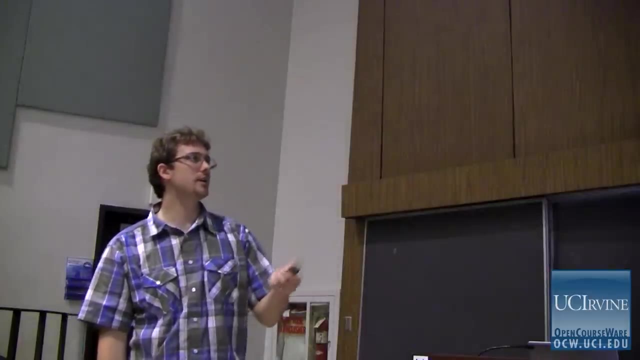 So we can do that right off the bat. It's this side With the more complex equation that gives. that causes us grief. So we can start with just PV as a quick guess, which doesn't have the A and B in it. 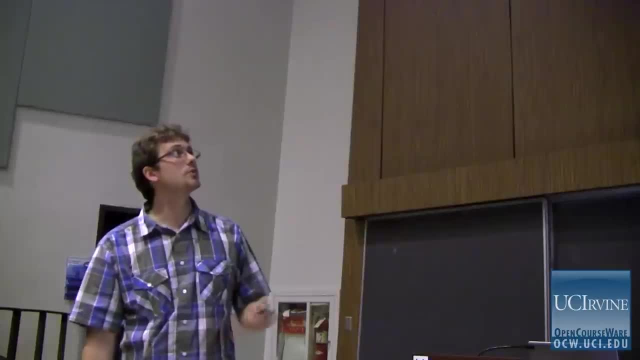 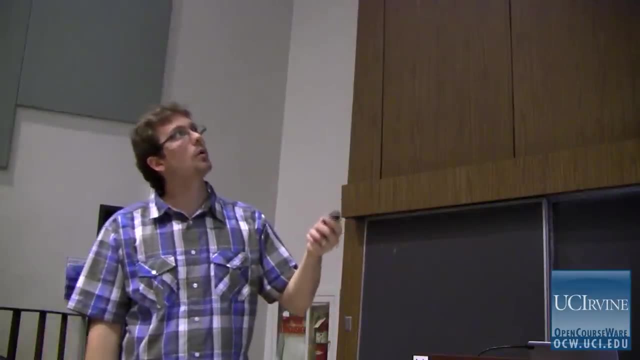 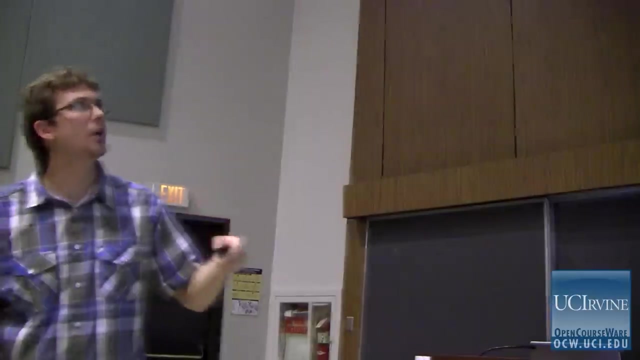 And then we can, in, in his words, scoosh our way over to the correct answer. So if we let our function of volume equal 2 ATM plus 4.192 liter ATM for volume squared times volume minus .05156L, so let me go back for a second. 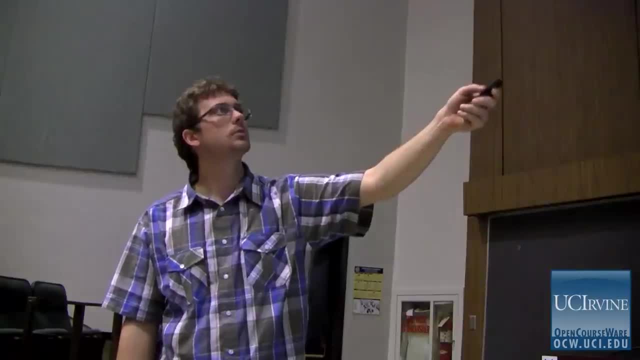 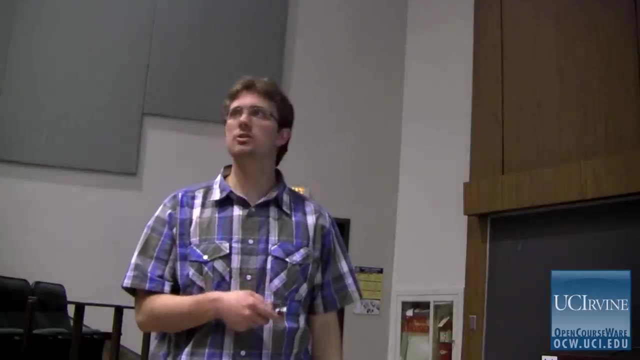 What we're doing is We're taking. oh, there we go. We have this equation right. We're trying to figure out the volume, So we can easily make this a function that depends on volume, And that's just pressure plus AN squared. 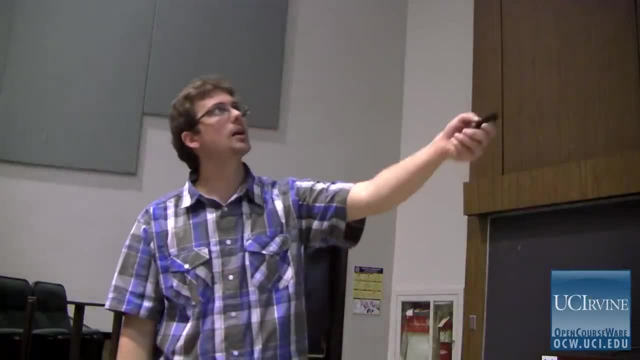 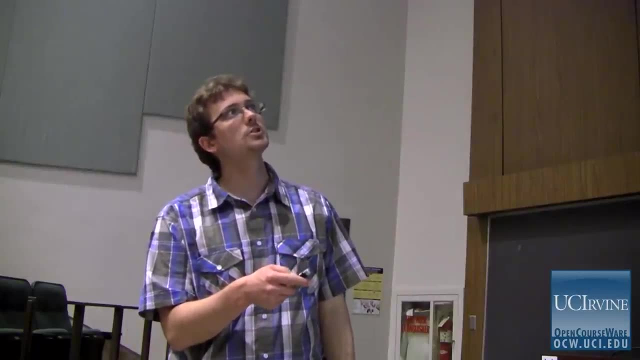 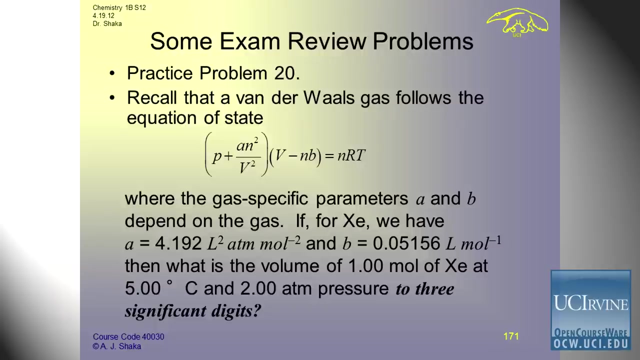 over volume times volume minus NB. So let's go back up to that slide. So our function: pressure plus the 4.192 liter squared ATM over B squared, So that's A, that's AN squared over volume. So that's AN squared divided by B squared times V minus the NB. 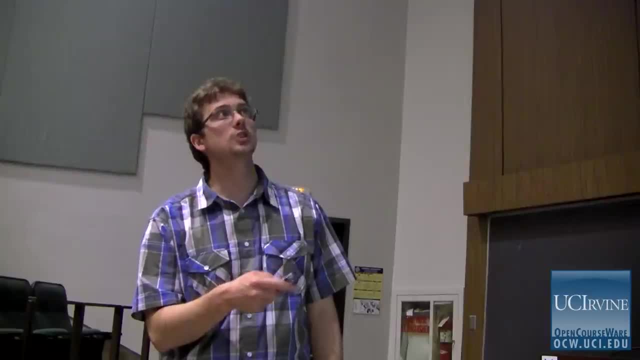 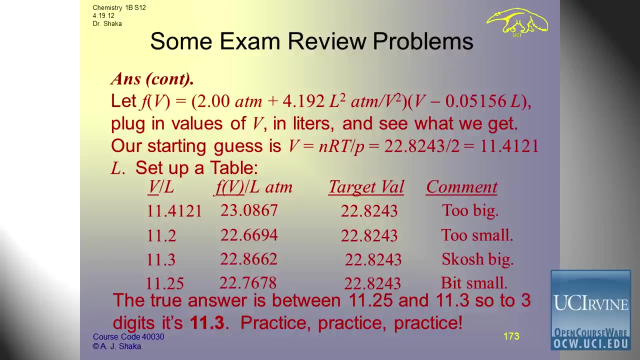 So he just figured out these numbers and put them in And this is our function for V. So if we plug in values of V in liters and see what we get, our starting guess is, using the ideal gas equation, just V equals NRT over P. We should all know that definitely. 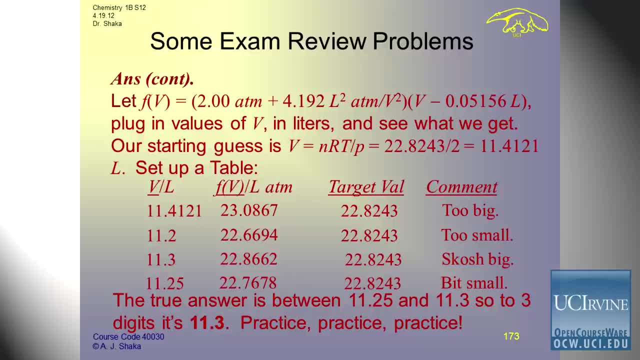 And that guesstimate is 11.4121 liters. So we set up the table, Okay, Where this is the volume in liters, this is the function of volume in liters, ATM, our target value, which should be 11.4121, and then a little comment on that value. 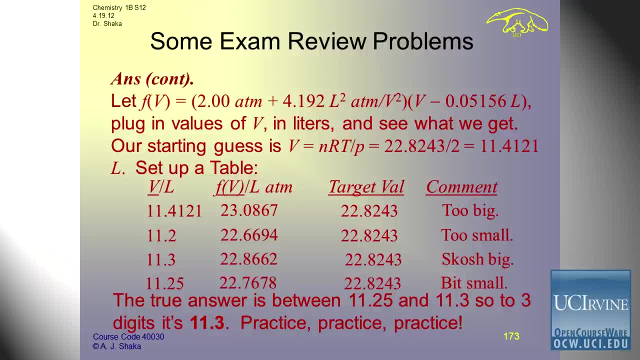 So when we do the ideal gas law, we have 11.4121, or the target value is 22.2.. When we do volume based on the ideal gas law, that's 11.4121. And the function, when we plug volume into our function, is 23.0867 liters ATM. 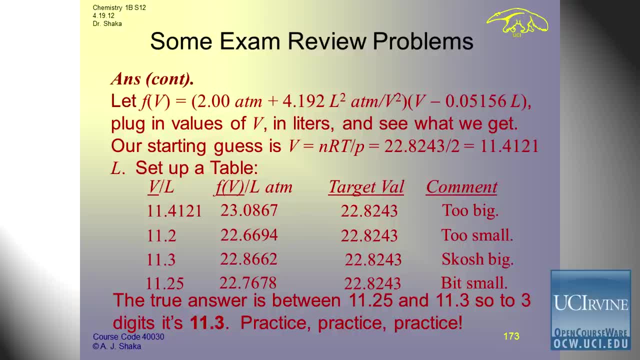 Our target value, which is NRT. right, we're trying to get PV equals NRT. Ideal gas law wasn't good enough. Van der Waals equation has A and B. We're taking that first guess, putting it in the function, we know that NRT is 22.8243.. 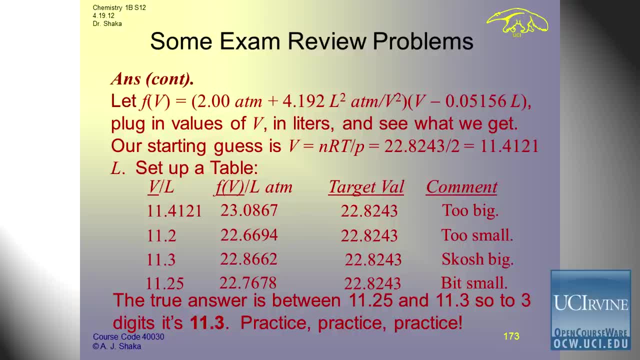 And we're trying to see how accurate we are. So volume 11.4121.. So we're trying to get PV equals NRT. So volume 11.4121 gives us too big a value. So we go a little bit smaller in volume, right 11.2.. 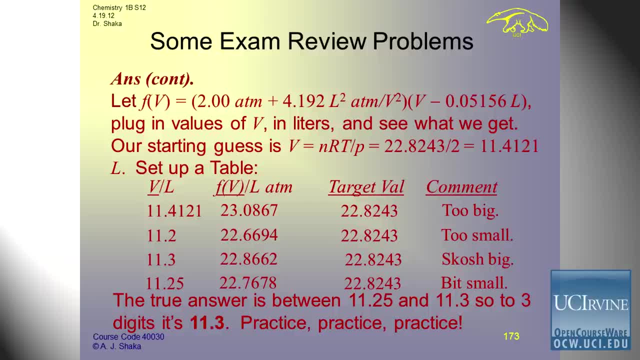 Well, put it into our function and that's a little too small. So 11.3, if you put that in, and we're just skooshed in His words, not mine. I think skoosh is a weird way to describe it. 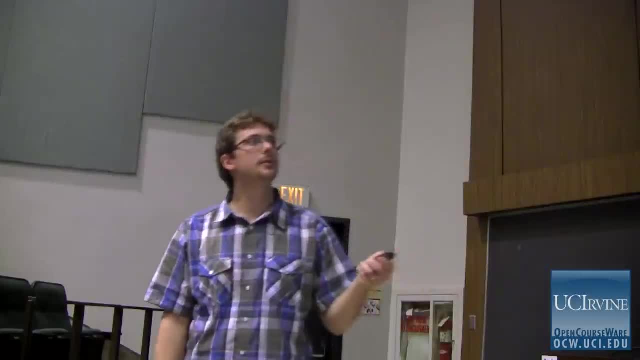 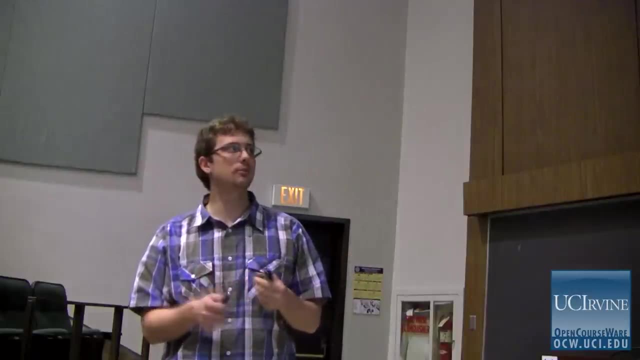 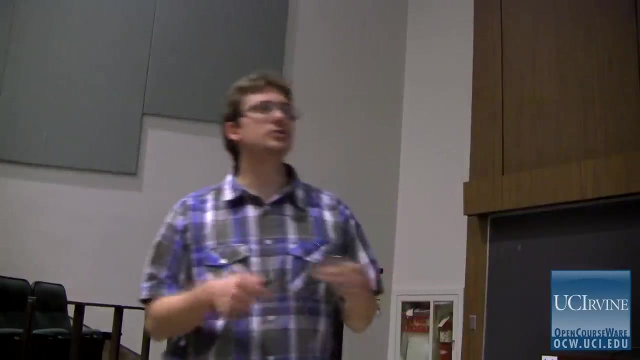 I've got to use timing, So 11.25.. That's a bit small. So, depending on what accuracy we're looking for, we know that the answer is in between 11.25 and 11.3.. So rounding to three digits, like it asked, that's 11.3.. 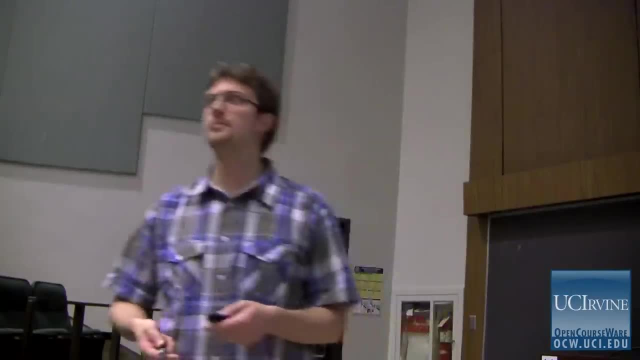 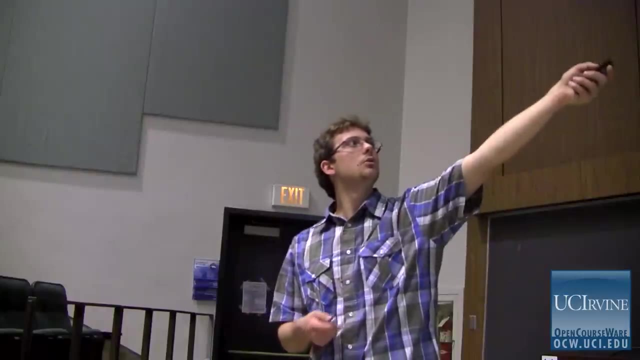 Practice that You have a question. Yeah, sorry, How do we know to divide NRT by a question, I think the last probably terms. they just put it in NRT So over. oh sorry, I'm sorry. Oh, I go all the way back, don't I? 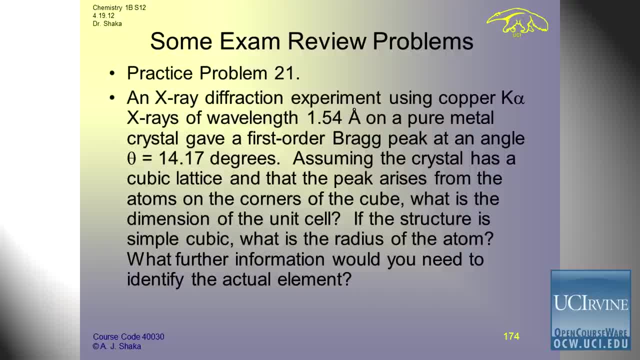 Okay, So equation accurate. Ideal gas equation not so much. right, We can replace all of this with PV and that's the ideal gas equation. So going forward. your question was: why does? let me bring it up- 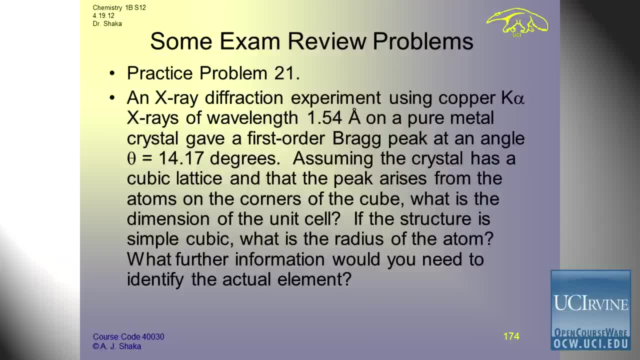 Why does volume equal NRT over P? That's just using the ideal gas law, right? Did that answer your question? I feel like I missed something in your question. Is there something that I didn't get to? Yeah, Okay, I did. 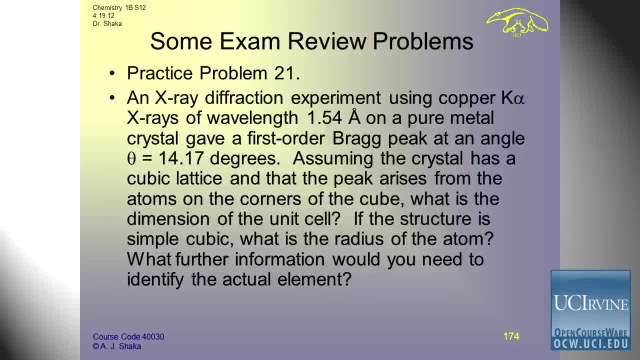 All right, Good, Good. Any questions with that? No, I think there's one more problem. Let me just go ahead. Yeah, So we have an x-ray diffraction question and we have 12.8.. All right, 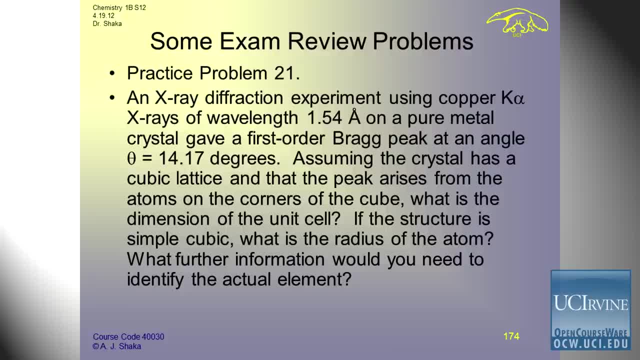 We got 12 minutes, All right. I think this is the last problem- An x-ray diffraction experiment using copper K alpha x-rays. so that's just describing what level of x-ray it's at- of wavelength 1.54. angstrom on a pure metal crystal gave a first order. Bragg peak. 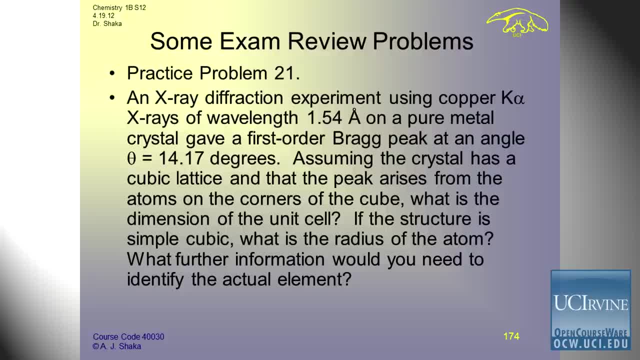 at an angle theta equals 14.17 degrees. If you're not familiar with this, go read the book. They have a quick and simple explanation on diffraction and how this is working. So we have a metallic crystal. It's just layer upon layer. 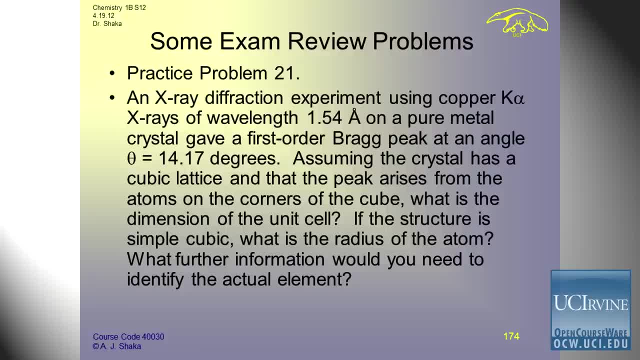 It's a simple cube, probably of metal. So the incident angle of radiation is 14.17 degrees and they tell us the wavelength is 1.54 angstroms, Assuming the crystal has a cubic lattice and that the peak arises from the atoms. 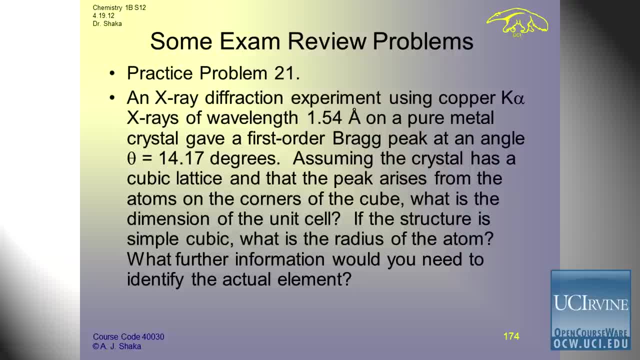 on the corners of the cube. what is the dimension of the unit cell? If the structure is simple cubic? what is the radius of the atom? What further information would you need to identify the actual element? So I'll go ahead and give you one minute. 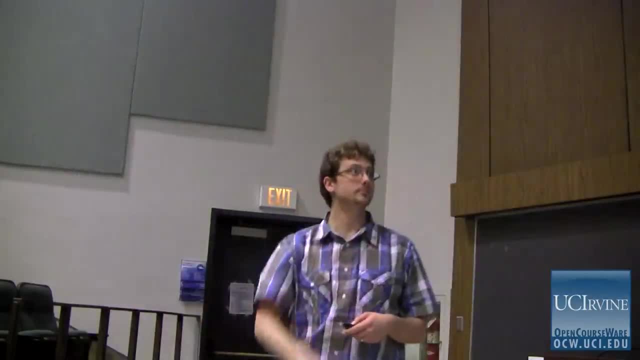 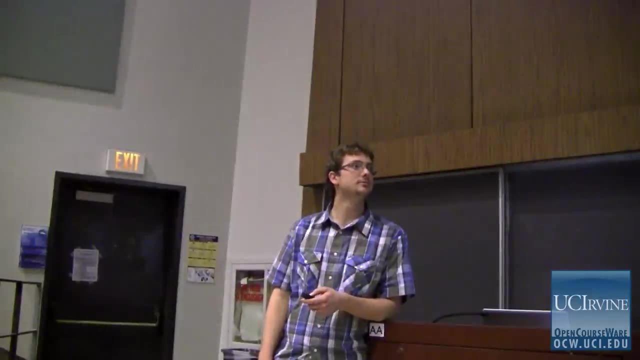 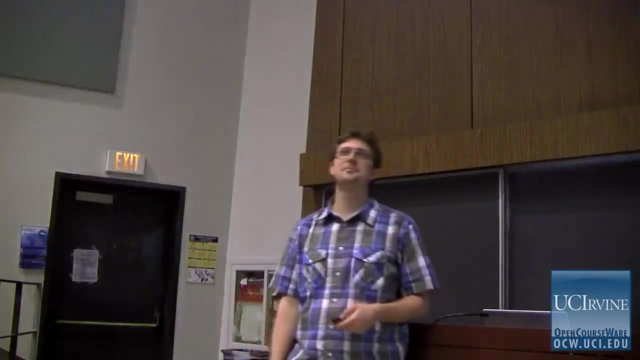 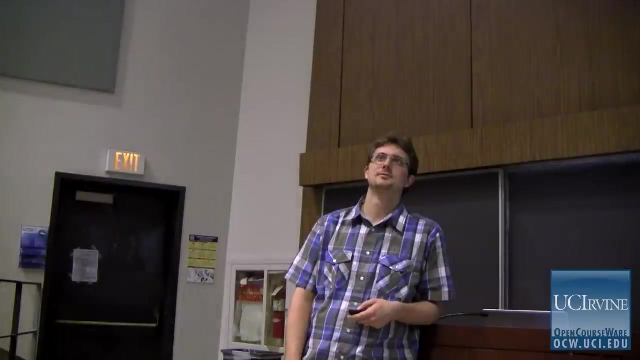 to work on this a little bit, excuse me, and then we'll work over it. yeah, It's funny. it's funny to be down here and actually see people like sleeping with their heads and stuff like that. Like I mean, I just want to like laser point them in the eye. 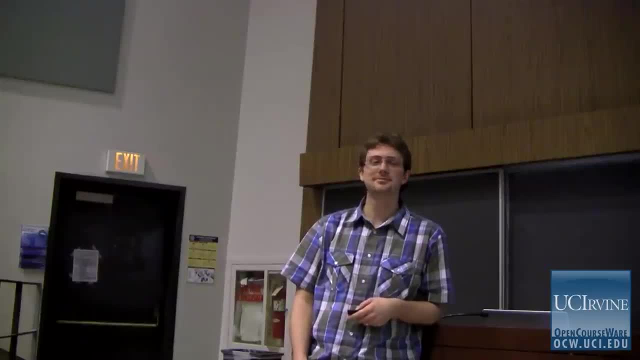 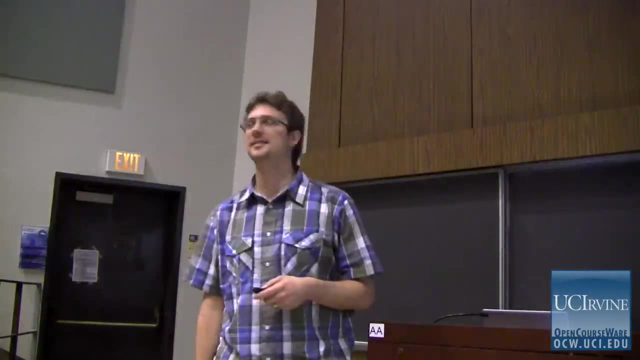 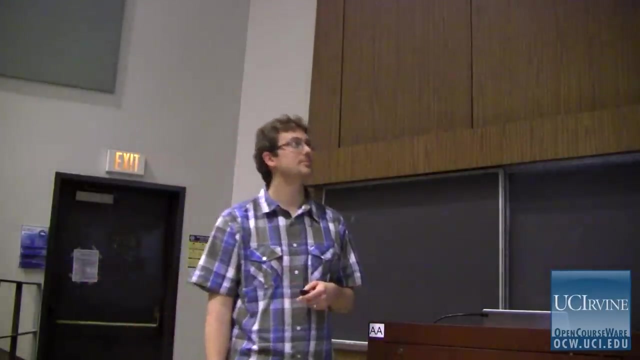 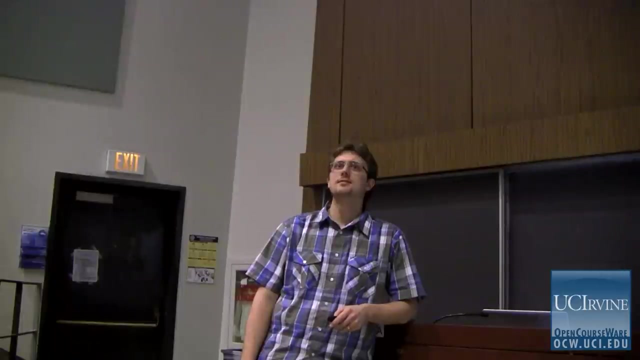 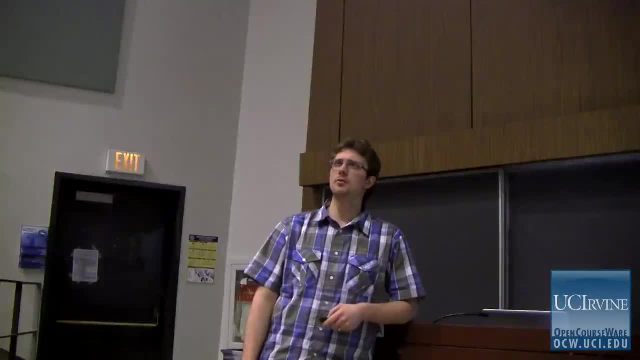 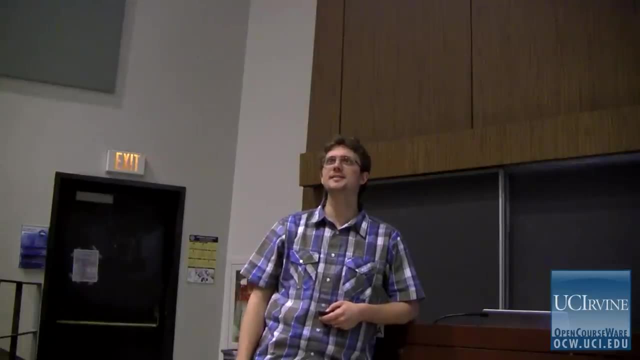 All right, All right, Real quick. before we go over it, I want to ask you guys up there in the balcony: is my camcorder still going? It is Okay. This is my first time teaching a lecture with this many people. 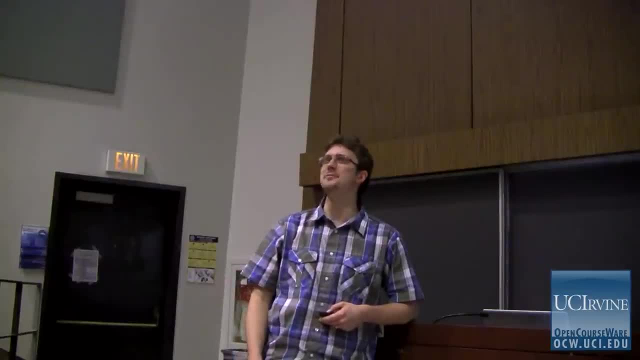 Never done it before. Can you all just give a shout out to my mom and dad? I'm going to send it to them. So I'm three. We're all going to say hi mom, Hi dad, All right. 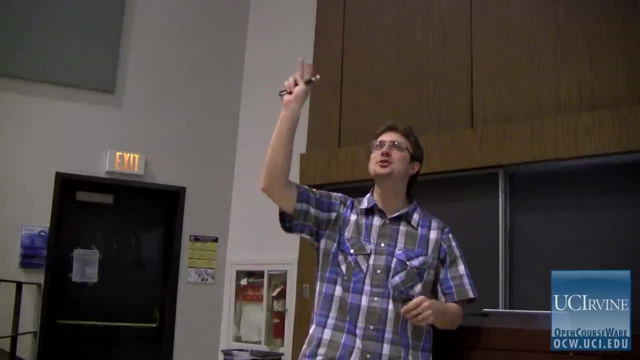 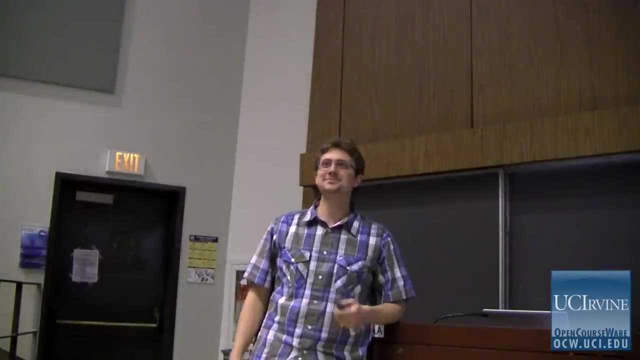 Just for me, Two for me, Two for me, Two for me. Okay, One, two, three Hi mom, Hi mom, Hi dad. Love you, Okay, So all right. Oh, my wife. 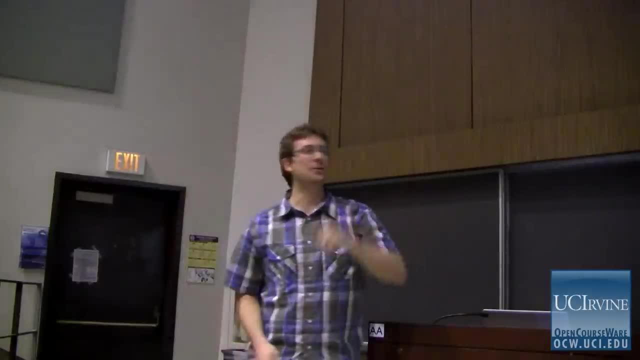 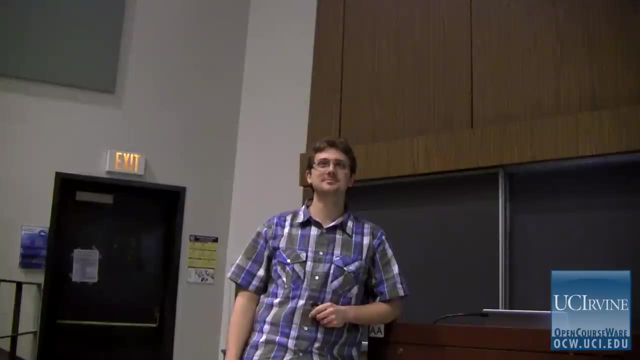 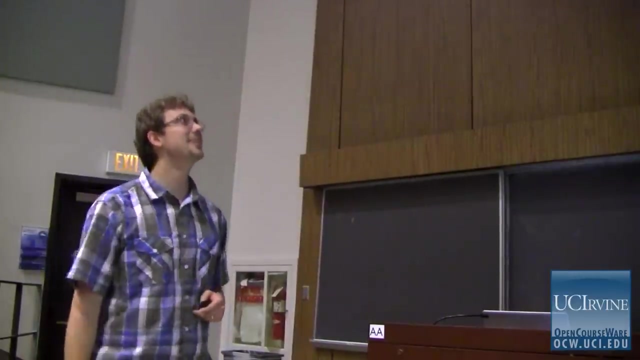 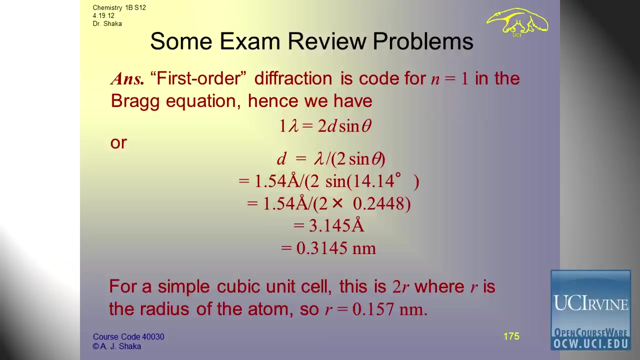 Hi Daniela. Hi Daniela, Thank you. Okay, Let's talk about this. How about this? All right, So we have a first order diffraction and that's code for n equals one. If we're thinking about this equation, okay, one. normally this would be n: n equals one. 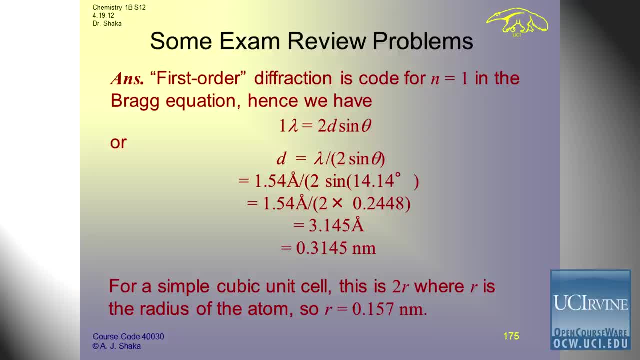 in the Bragg equation. Hence we have one times the wavelength, which we already have, because they gave us. that equals two times d sine theta. They gave us theta. What we're solving for is d, So let's go back one second here, because there was an assumption that was made and 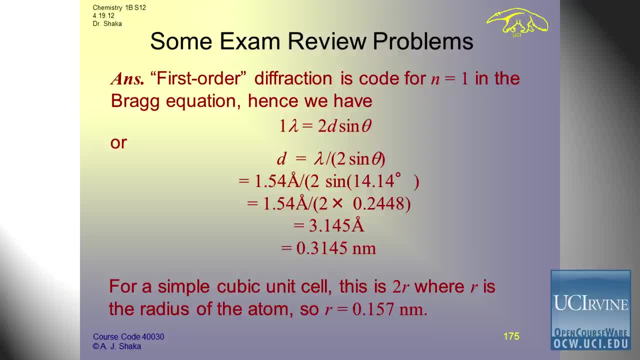 we didn't talk about it. When it says that, assuming the crystal has a cubic lattice and that the peak arises from the atoms in the corners of the cube, what that's saying is: d was a measure of the distance in between my slit, where the x-rays are being diffracted right. 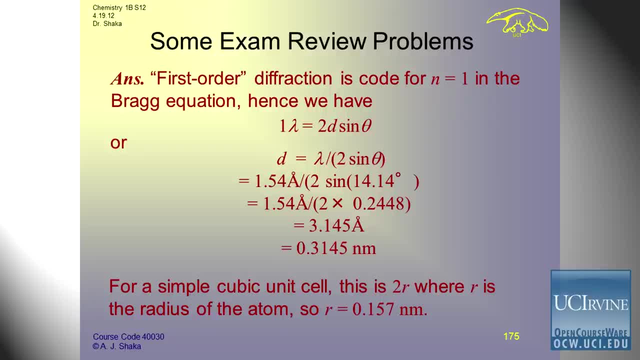 It's not always the case that one set of layers makes that diffraction. We're making that assumption. So if I just solve for d, well, maybe that comes down to ten angstroms and that could correspond to five or six layers. 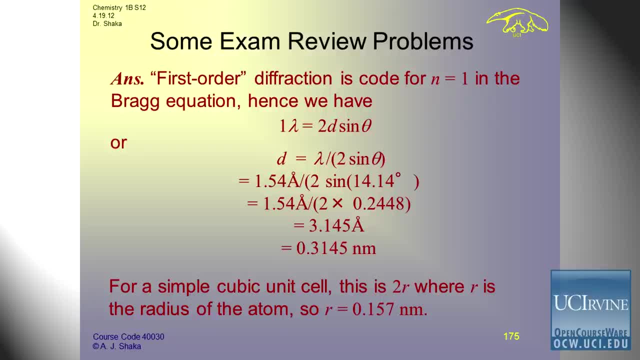 Okay, So we made the assumption that it's from the first layer and so d is just the distance in between the two corners. on that point, Okay, So 0.3,. so if you solve for d, that's 0.3145 nanometers. and for a simple cubic unit cell. 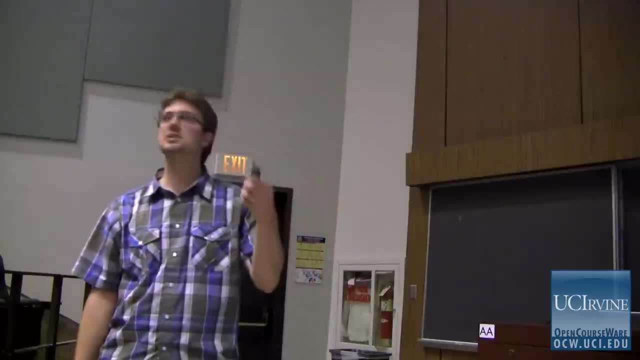 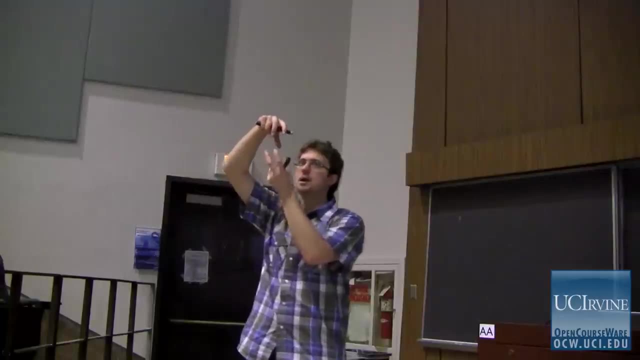 this is 2r. Remember we were trying to solve the radius of the atom. If it's a cubic lattice, I have atoms at all the cubes, and they're touching each other, right, Right, They're touching each other and I know the distance in between, the middle point of those. 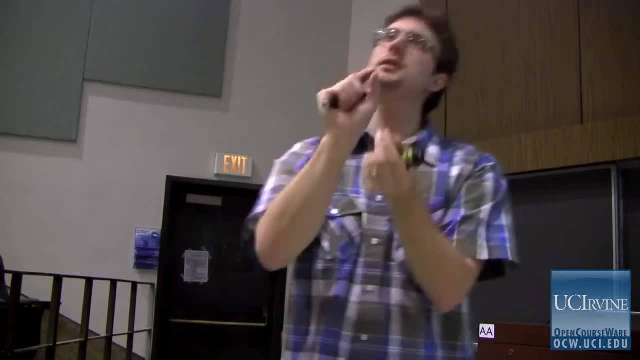 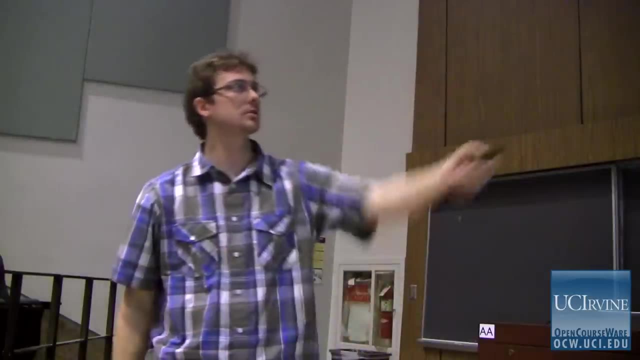 two atoms because they're right at the corners. then I know the radius of each atom because I know the distance and the radius is just 0.157 nanometers. So cut that in half. So we're trying. 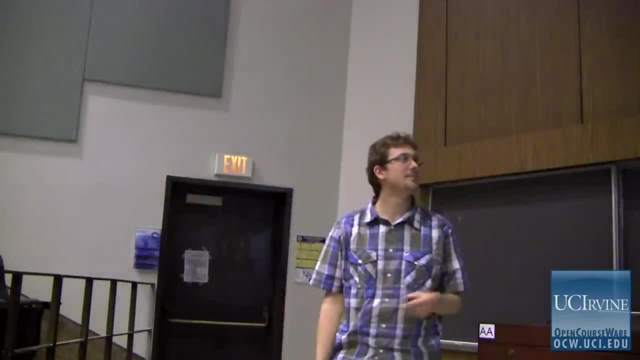 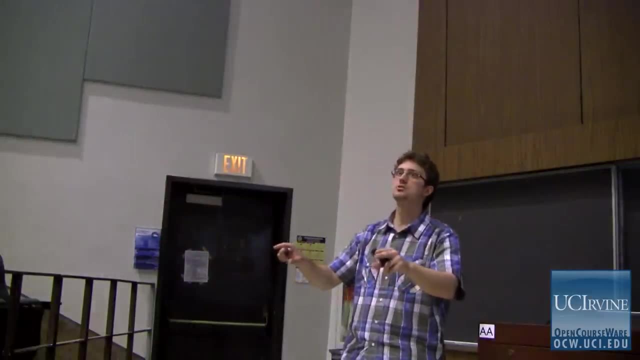 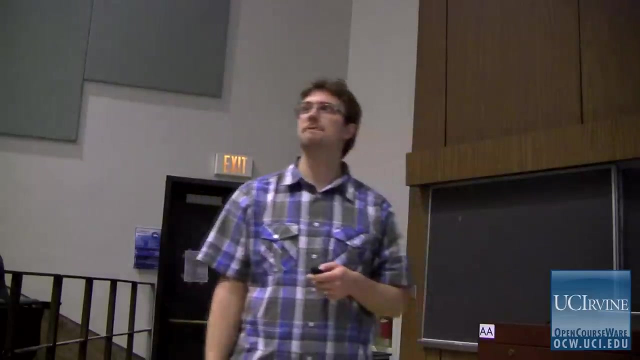 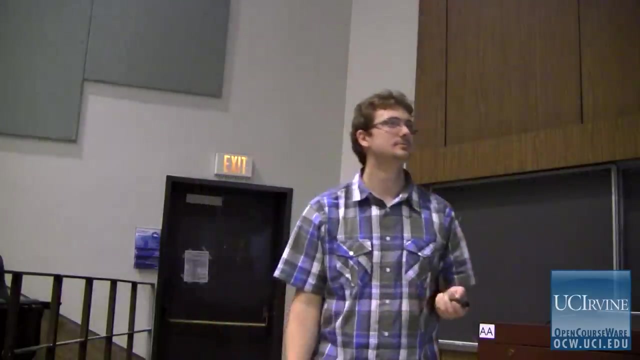 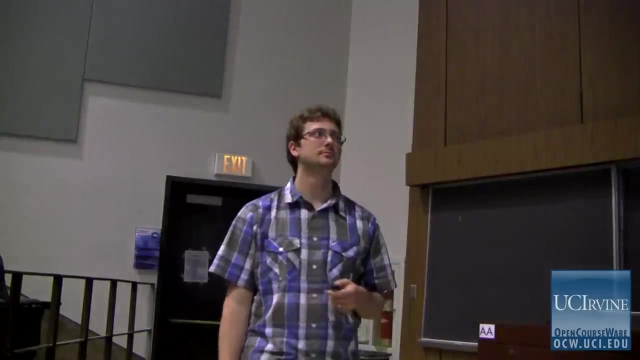 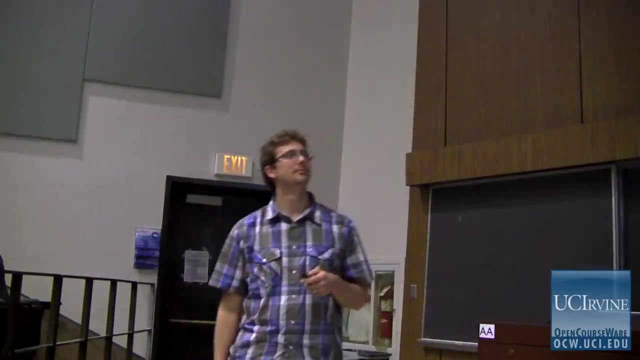 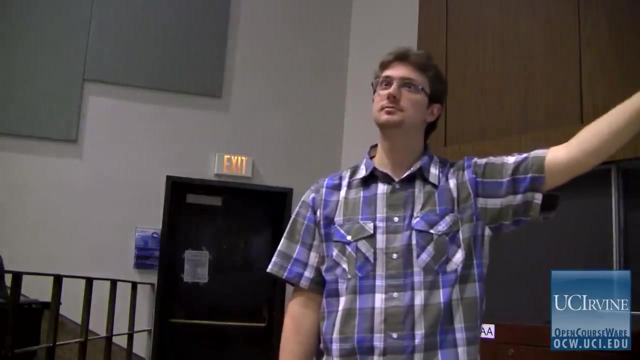 Oh, sorry, Sorry, My bad, My bad. We're just writing down. Do we have questions? Questions? so far, Just writing down. Okay, All right, Let's see what we have. All right. Moving on, I'm hearing a lot of murmurs, which I don't know if that means yes or no. 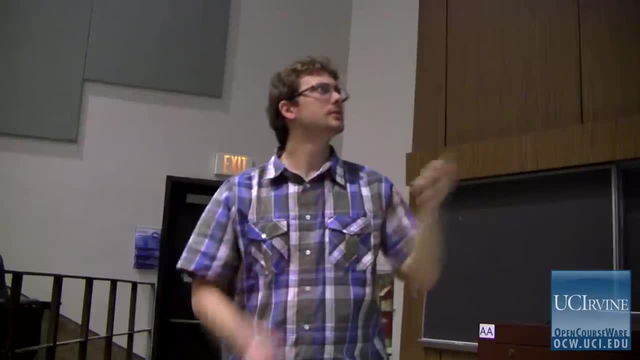 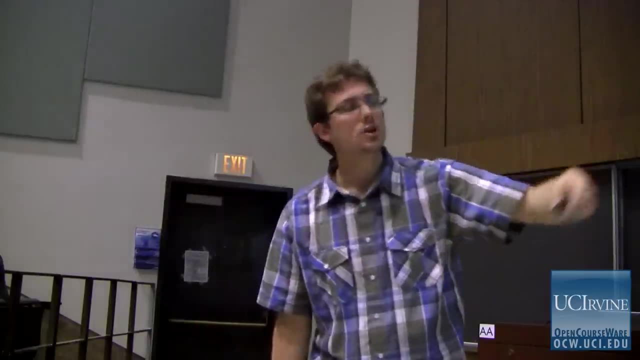 So we were trying to find the. Let me read the end of the question again real quick. We were trying to find the mass, right Yeah, What further information do you need to identify the actual element? So what do we need to identify the element? 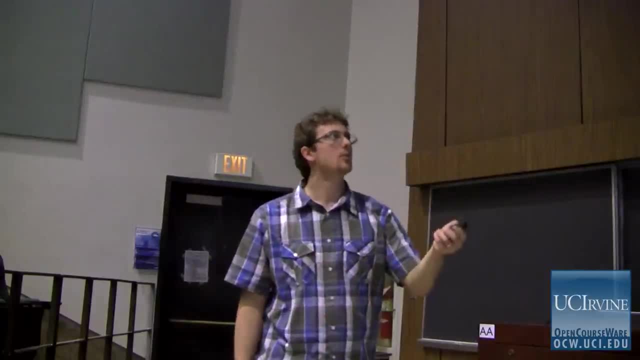 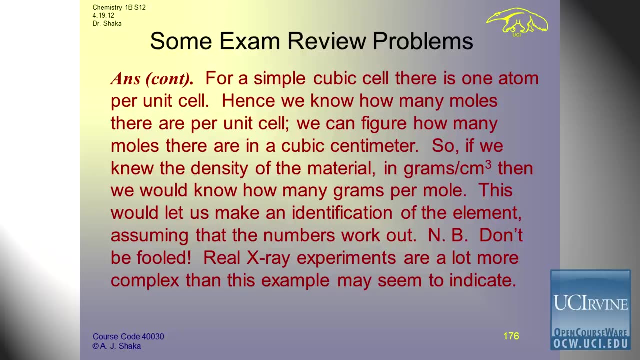 Well, we already have the volume, right. We have the radius. What's the last thing that we would need For a simple cubic cell? there is one atom per unit cell, right? That's because at each corner we have one-eighth of that atom contributing to the unit cell. 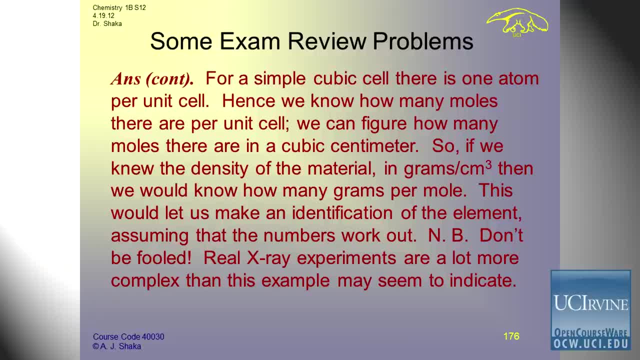 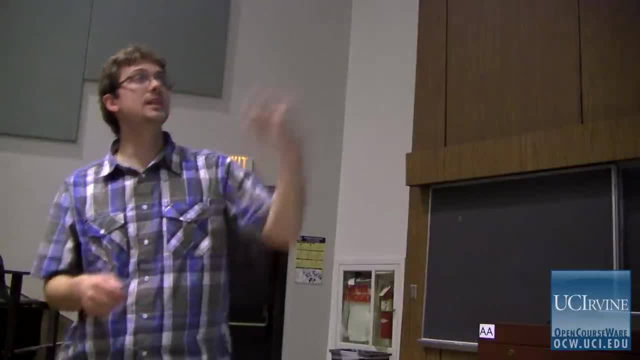 Eight corners, that's one atom. So we can figure out how many moles there are in a cubic centimeter. So if we then knew the density of the material in grams per centimeter squared, then we would know how many grams there are per mole.